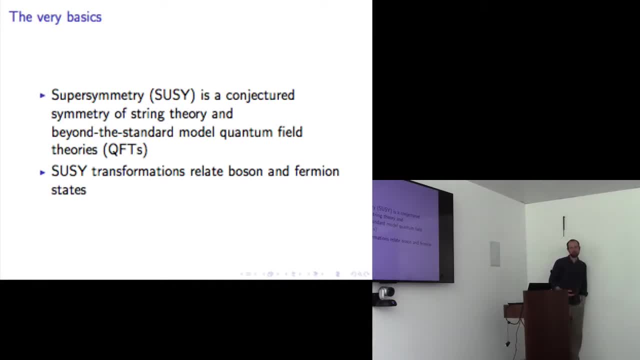 kind of ragging on it, hating on it or lamenting how badly things have gone for it. It's a bit exaggerated, but whatever. But what it is is a conjecture, right? So it doesn't have any kind of direct experimental evidence of any sort in favor of it at this point, so keep. 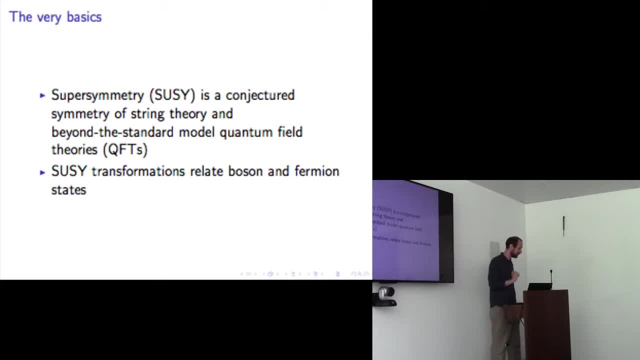 that in mind, in the course of discussing it, Any kind of direct empirical evidence that it's true, But it's a conjectured symmetry of string theory and quantum field theories that go beyond the standard model right. So the thought is that there is a transformation, that these theories are invariant, under which 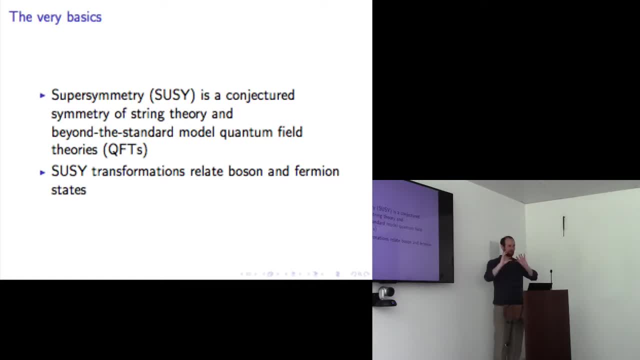 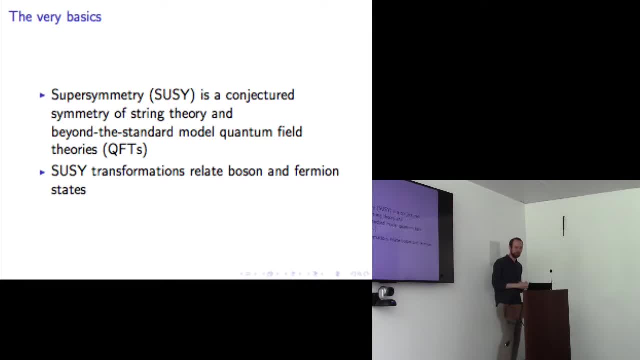 state and you apply a supersymmetric transformation to it and turn it into a state of fermion, of a fermion right Now. why would we look at it as philosophers? now? I mean essentially, the answer is because it hasn't been done previously and it is of great intrinsic interest. 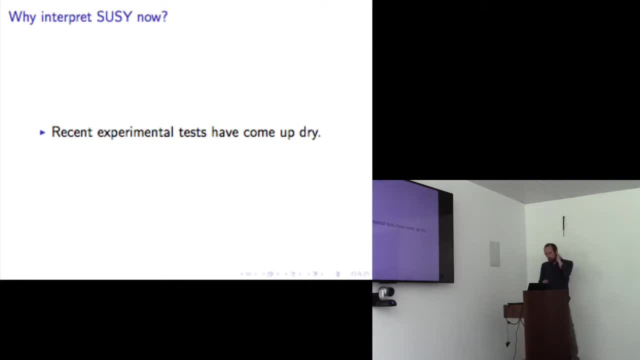 So it's absolutely true that they were hoping to find it at the LHC. oh is, oh, is that? how bad is that then? the flickering? is it okay? Alright? alright, that's cool, Alright. so it's actually true that they were trying to discover at the LHC and did not, but you. 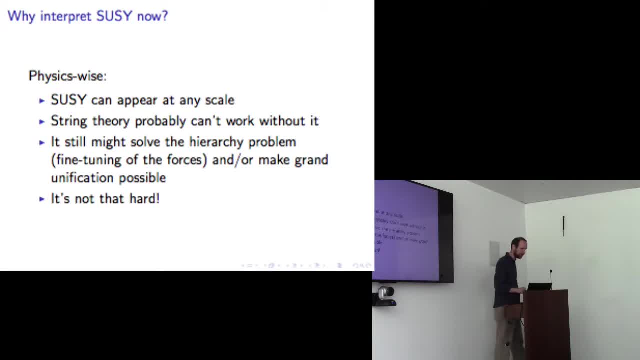 know, of course it's also true physics-wise that there's no restriction on which energy scale Suzy could show up at. So I was the outside member of the dissertation committee for a guy working on a PhD program that I was working on a PhD program that I was. 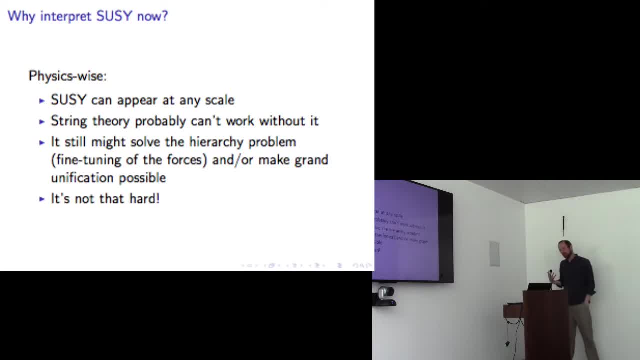 kind of dissertation in theoretical physics at Michigan and he was working on supersymmetry and I was like, well, hey, you know, how does your confidence? I tried to ask this question from a Bayesian point of view. I was like, how does your confidence in the truth of supersymmetry? 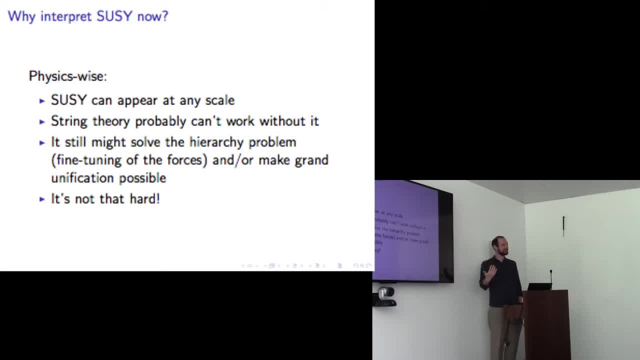 how would it change if we didn't find it at the next accelerator? And his answer was: well, you know, it can show up at any scale, So supersymmetry will outlive us all. right, It wasn't a very Bayesian answer, but I think it's a true answer in a sense. We still don't. 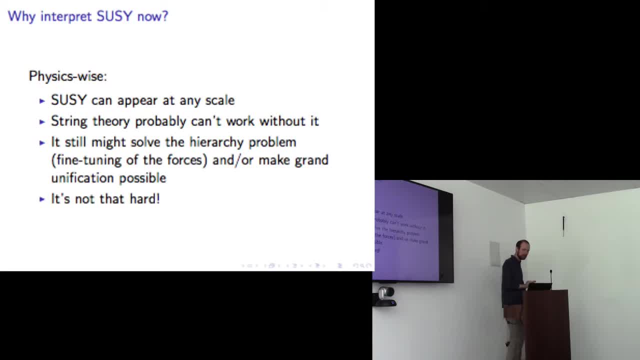 know anything that rules it out in any way, And the reason I think these days to be somewhat confident that it might show up is that string theory does seem to be at least a promising program in quantum gravity and as far as we know, it can't work without supersymmetry. 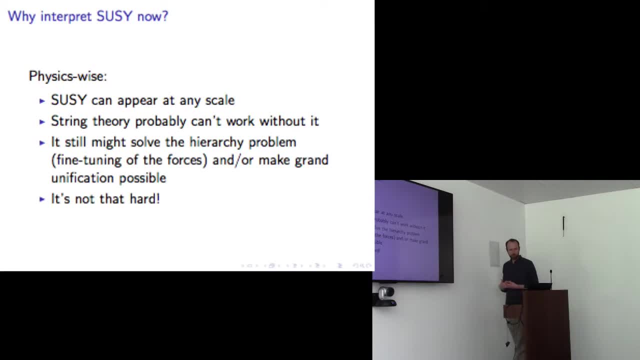 in the sense that we don't know how to really represent fermions. And it's still possible that it might solve what's called the hierarchy problem or the fine-tuning of the strength of the different forces. right, Why is the gravitational force so much weaker than one of the other forces, for example? And possible that it might make? 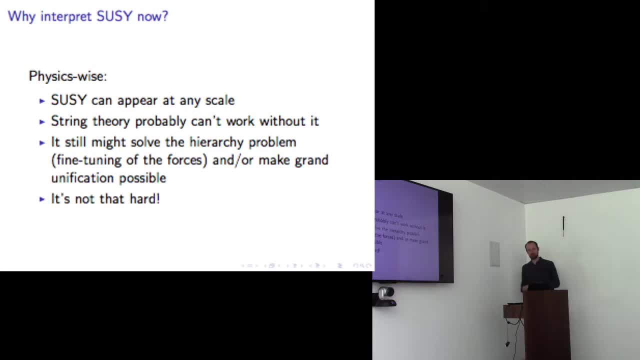 grand unification of the three non-gravitational forces possible. And another reason physics-wise to look at supersymmetry is that, as I hope you'll feel as we go through these slides, that Susie isn't that hard compared to some of the other stuff that we work on in the 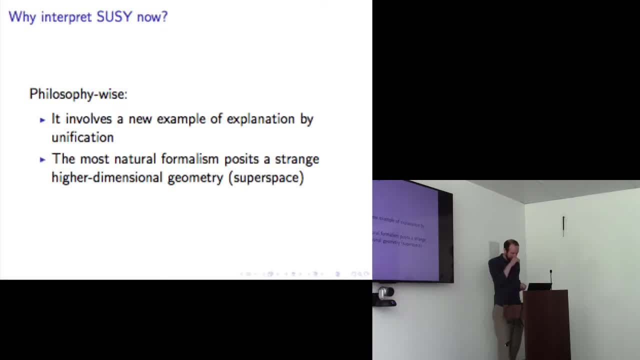 philosophy of quantum field theory. Okay, As far as philosophy goes, there's some very cool reasons which have essentially been pointed out prior to my work on the topic by first. well, Robert Weingart wrote this paper on the philosophy of string theory. you know, a few decades ago at this point, 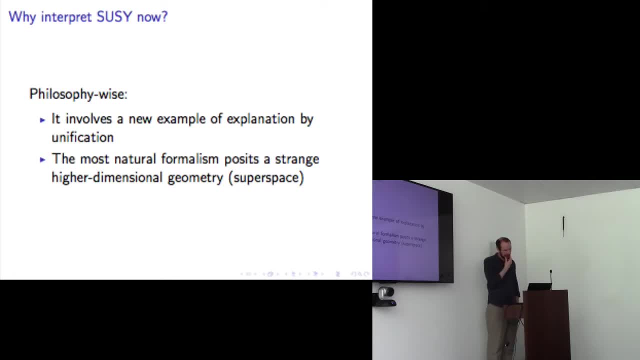 which pointed out a number of the interesting issues in the philosophy of string theory And the philosophy of supersymmetry, and then some of the you know- essentially a new question about supersymmetry, somewhat different from the ones that. I'll put it this way somewhat. 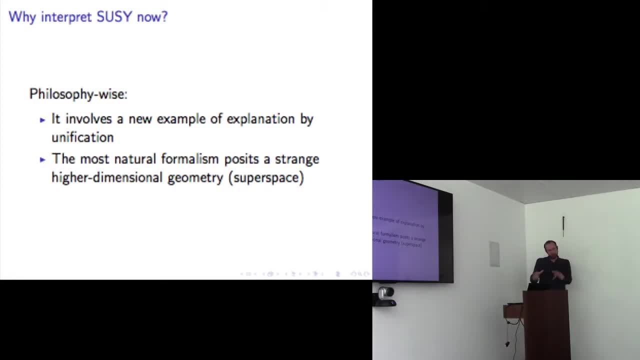 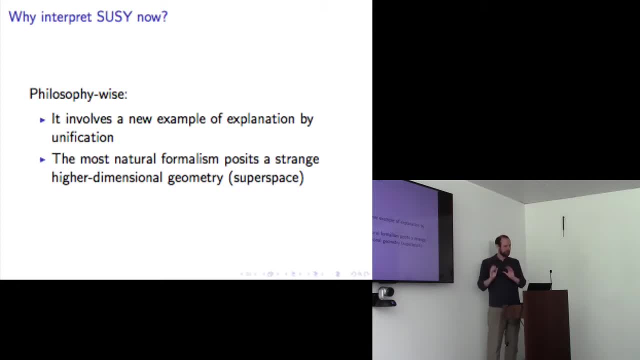 Here's a bunch of things. Here's a bunch of things. Here's a bunch of things. Geometry: positive by supersymmetry. we call it superspace. is that space-time right? So, philosophy-wise, SUSY involves a new example of explanation: by unification, because we're 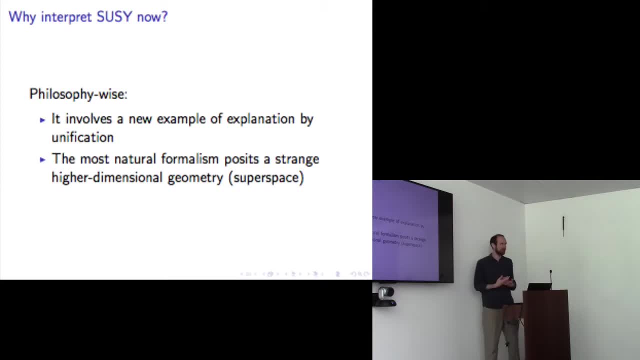 unifying explanations for fermionic phenomena and bosonic phenomena, right. So that's an important issue of philosophy, of science, obviously, And the most natural formalism to use for SUSY involves positing of strange geometry with more dimensions than we usually think, of space-time as having, which is called superspace. 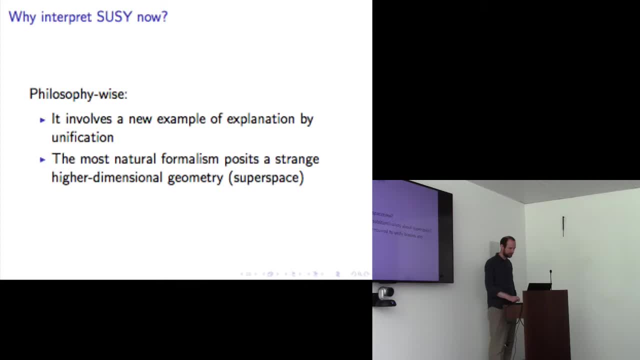 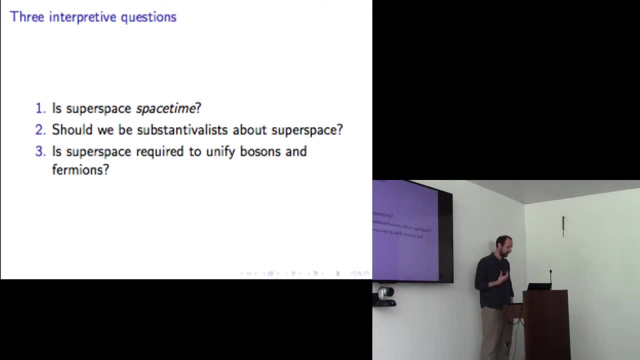 So that's where most of the interesting issues come from. So here are three interpretive questions. The first one is the one that Tushar's work is focused on, which is: is superspace, space-time Right? Should we think of it as space or temporal, or should we think of it as another way to? 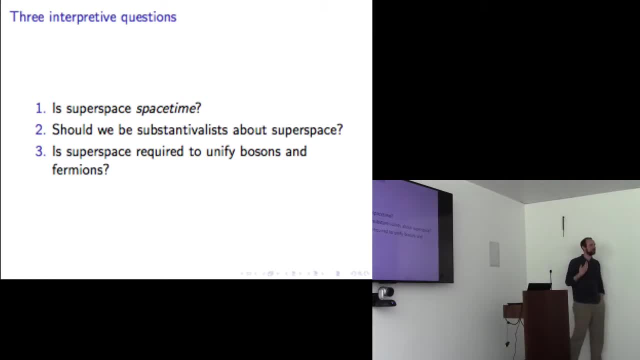 put this. perhaps a way to put it that makes it clear that it has is a question I think that has content is: is superspace the same kind of thing as space-time, the way we thought of it previously? You know, compare the question with Minkowski, came up with Minkowski: space-time right. 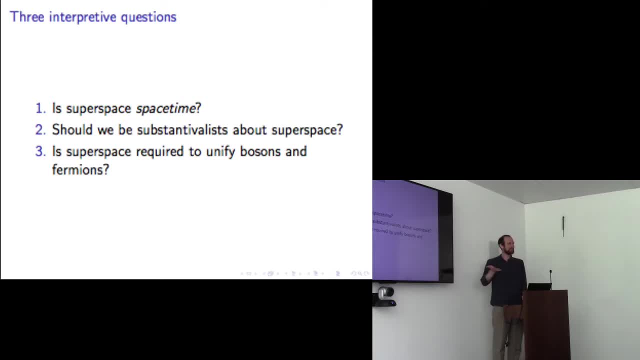 Is space-time the same kind of thing as we thought of space as being prior to that? The second question, which some people might say is very similar but I would say is quite distinct, is the question of: should we be substantivalists about superspace? 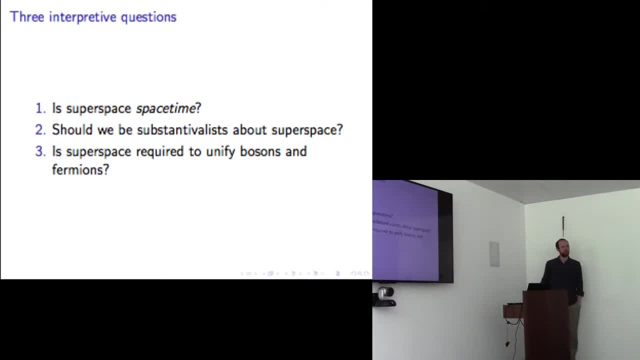 And in the way I'm going to use the term substantivalism, as you'll see, you can say no to the question about superspace being space-time and still say yes to the question. we should be substantivalists about it. And finally, I may or may not get to this, depending on time. 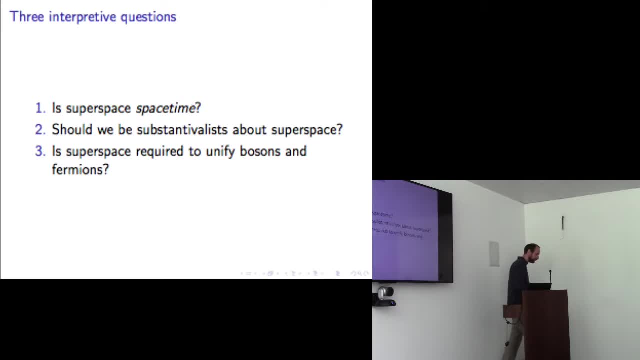 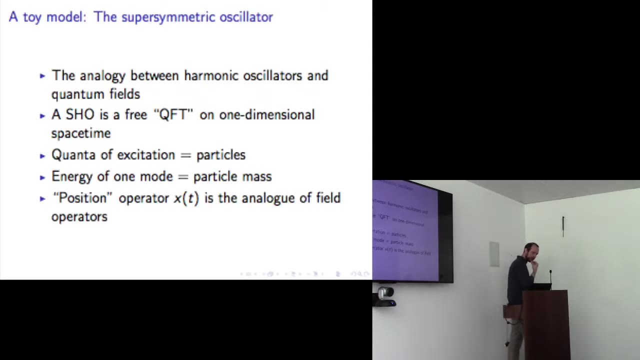 There's a question about whether we have to posit the existence of superspace or the spatiotemporality of superspace in order to unify bosons and fermions. Weingart had a view about that that, I think, is wrong. Okay, so here is the part where I'm hopefully going to be teaching you something. 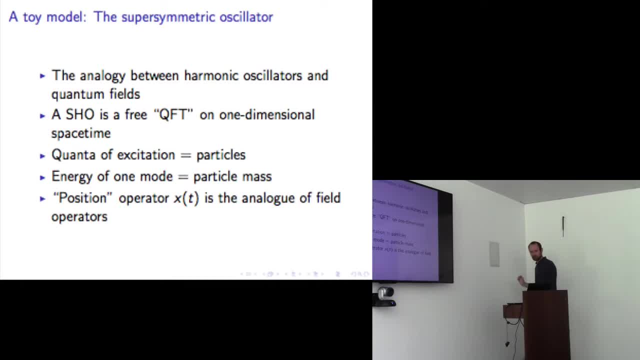 What does supersymmetry look like? What is the kind of simplest way to understand a phenomenon? And to do that We're going to look at a simple harmonic oscillator. So if you have worked through a text on quantum mechanics, you have used a simple harmonic. 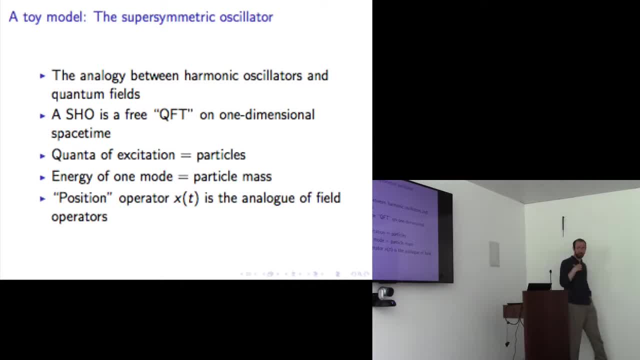 oscillator in what we call to presage what I think I'm going to say. you've looked at the simple harmonic oscillator in what we call its bosonic version, where there are unlimited modes of excitation available to the oscillator, as opposed to there being. 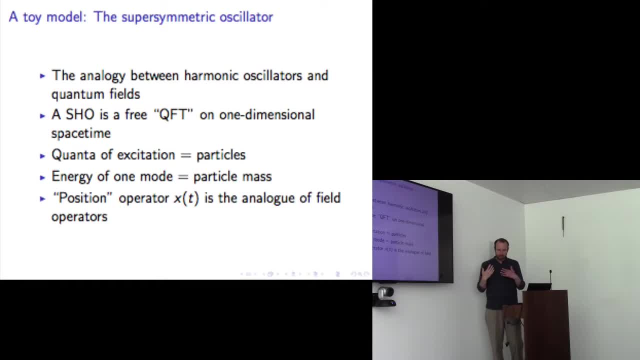 to presage another. There's another thing I'm about to say, a sort of exclusion principle that keeps the oscillator from being excited beyond the first mode. Let me focus on something that will be useful to you as well, if you think much more about. 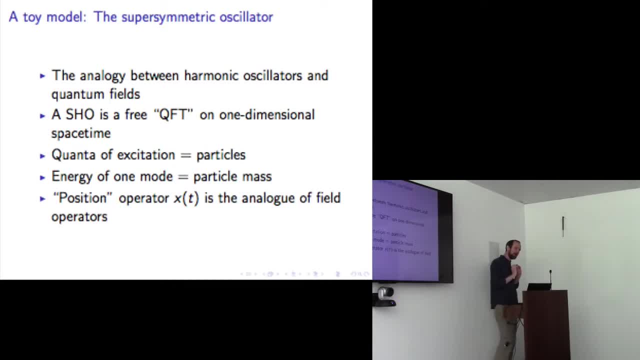 the philosophy of quantum field theory just in general. There's this interesting analogy between harmonic oscillators and quantum fields and this is one of the nice things. If you ever read Paul Teller's- I don't know, It's kind of in some ways dated, but also classic book Interpret. an Introduction to 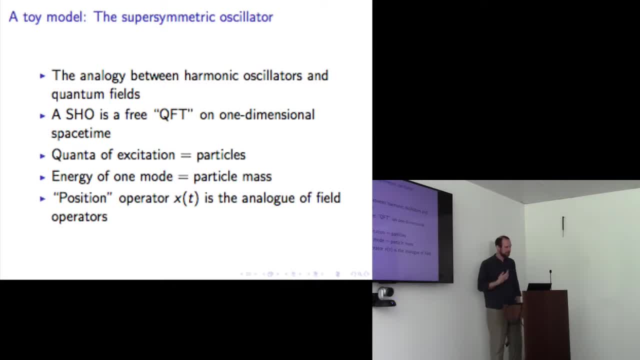 Quantum Field Theory. it's one of the things that he brings up very nicely, this analogy between harmonic oscillators and quantum fields. Or it also comes up in Teller's early papers on the topic and some of Nick and Bob Weingart's. 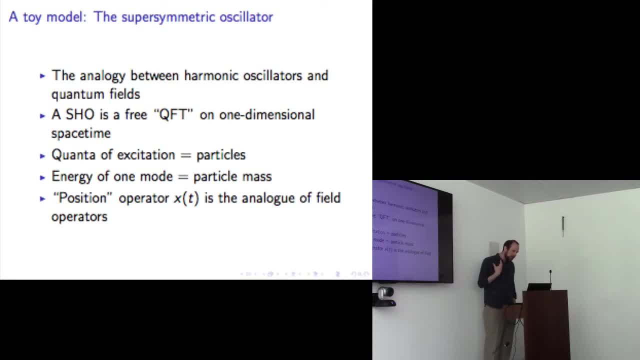 work. responding to that, There's this analogy between harmonic oscillators and quantum fields. If you look at just a simple harmonic oscillator, okay, you're thinking, well, there's this thing, It has this position, degree of freedom, right, and it has some amount of energy which is 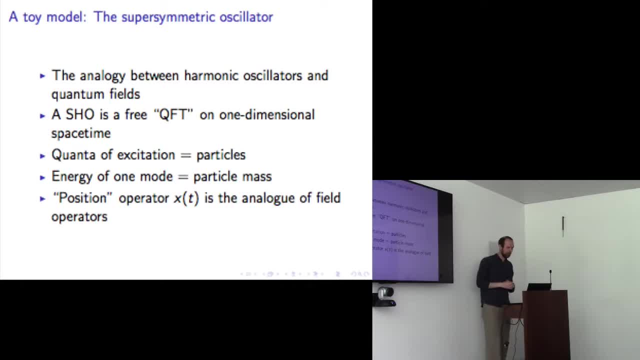 how many modes have I excited the oscillator by Now? what I want you to do is: don't think of that. position, degree of freedom, right? What is that? Well, it's kind of like you know, if it's a one-dimensional oscillator, it's kind of 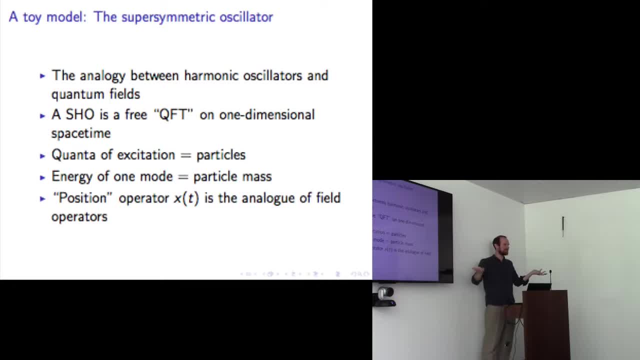 like a scalar, basically right. It's just like a number. What's the position of the bob, of the oscillator? What I want you to do instead is think of that. I want you to think of that position as the value of a scalar field on one-dimensional. 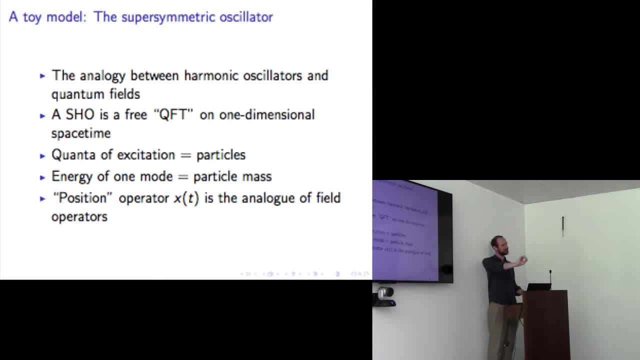 spacetime, right? So this is a spacetime of one point of space and you know a continuum of time, okay? So there's just one point in space and the field can get more or less excited at that point and that's it. 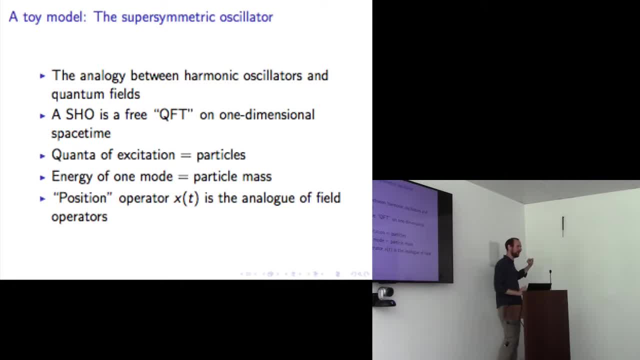 That's all that's going on in this imaginary world, okay, So there's a scalar field and that is the number that is quantum mechanically analogous to the position. It's the number that's going to be the constant of the oscillator bob in this example. okay, 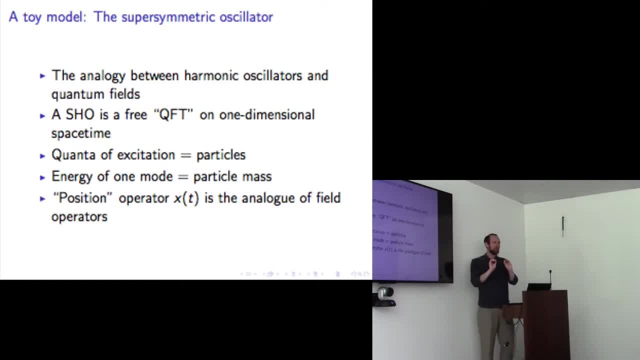 So think of the simple harmonic oscillator as being like a quantum field with one degree of freedom. In that case, right, a simple harmonic oscillator is kind of a free, that is to say like non-interacting, because there's nothing for this thing to interact with. it's just one field. 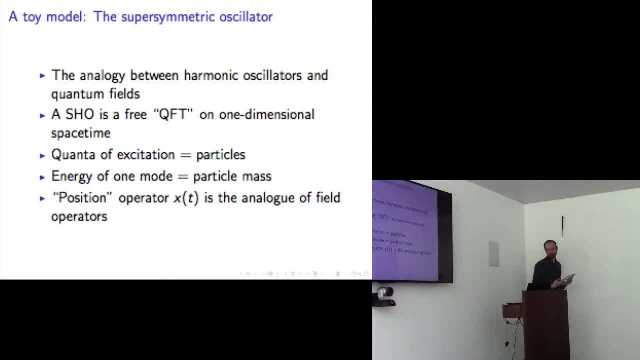 It's a free quote-unquote quantum field here on one-dimensional spacetime. Now what does it kind of mean In quantum field theory terms if I excite that oscillator and, you know, bump it up to an energy level beyond the ground state? well, that means I've added energy to it, right? 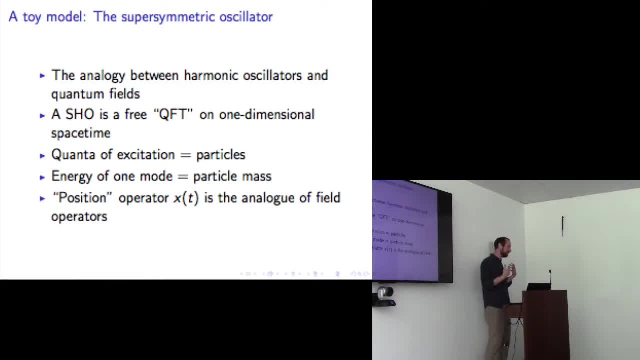 And in the particle picture of quantum field theory. that means, you know, excited states are particle states, right? So if I excite the oscillator, I'm adding particles, Essentially right. the only thing that's going on in this system is: well how excited. 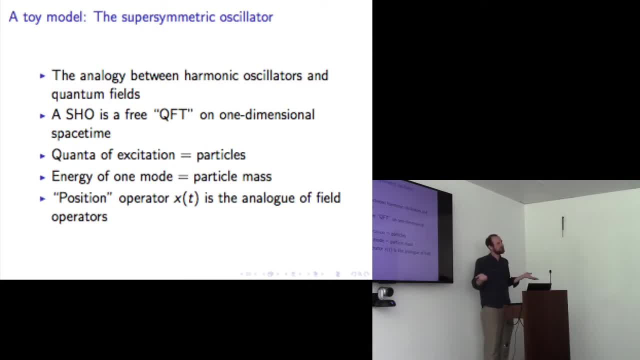 is it That tells you how many particles there are? right, There's one point in spacetime and the only thing that can happen there is it can be occupied by more or less particles. So quanta of excitation or modes of excitation of the oscillators are particles. 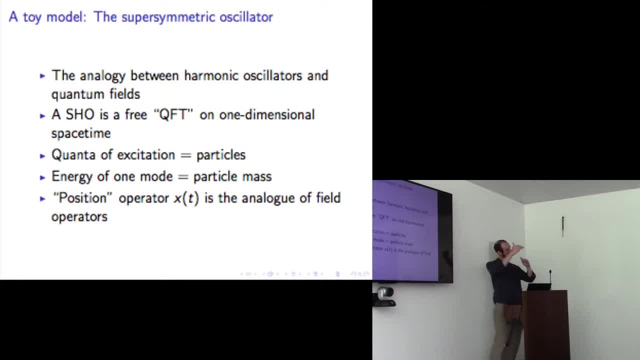 Well, if I add a particle, I've added, you know, I've excited the oscillator by one energy level, right? So that means the energy of one mode is the mass of a particle, right? Because that's the amount of energy that I get if I add a particle to the system. 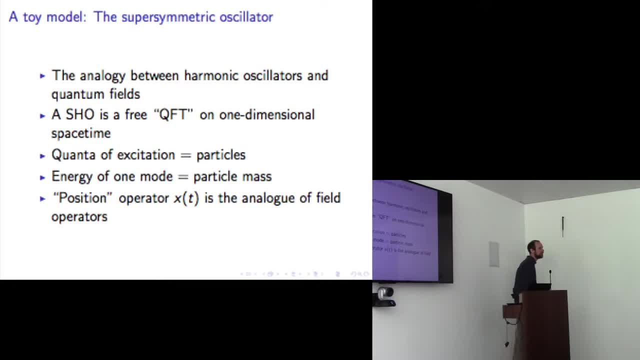 And since these things can't move, they can't move, They don't have any kinetic energy. So the only energy for the system is the energy of the particles and masses And, as I said before, the position operator is in this case the analog. 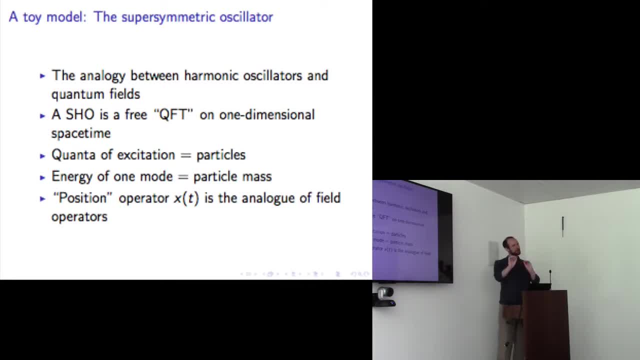 Well, remember, the position is the analog, The position of the bob, of the oscillator, is the analog of the field right, the value of the scalar field. So if we're doing quantum mechanics, we're going to represent that using an operator. 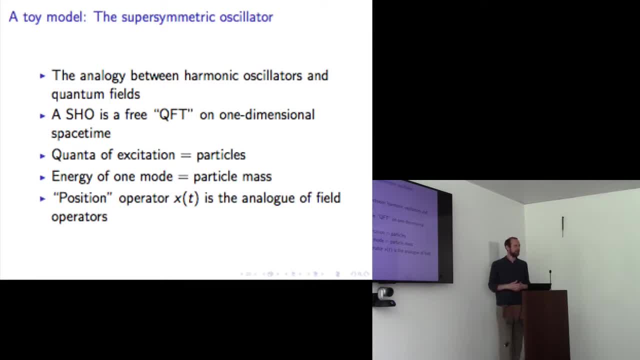 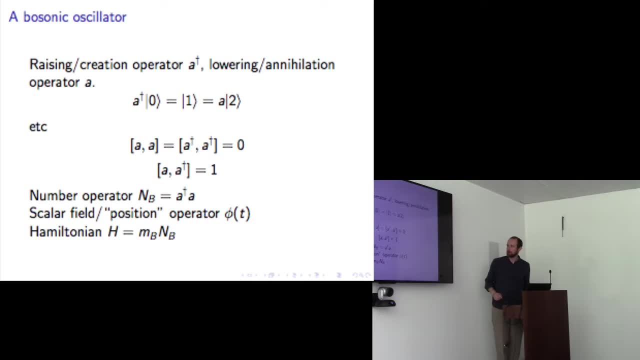 and that's going to be analog of what we call the field operator in quantum field theory, which we usually use the symbol 5.. All right, So I will now start to use the symbol 5 for that position operator, which is in the quantum. 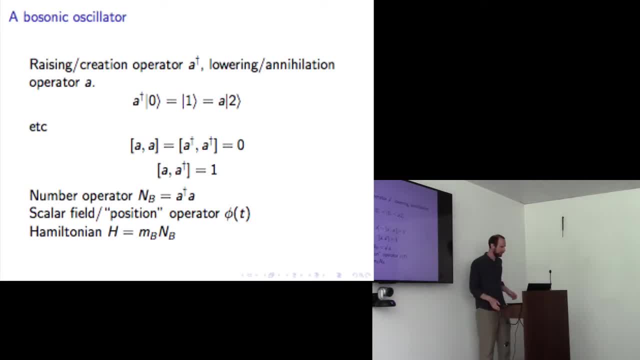 field theory, analogy, the field operator. Okay, So the bosonic oscillator is the oscillator you're familiar with from your textbook. You know, you pick up like you know, like Messiah or something, the messiah, I guess you're supposed to say. 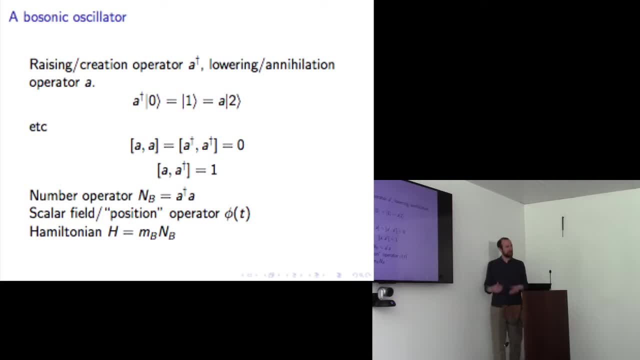 And you look at the regular harmonic oscillator and it's the bosonic oscillator. It's the bosonic oscillator. So just build it up in the usual way. You have a raising operator for the oscillator which we will think of in quantum field theory. 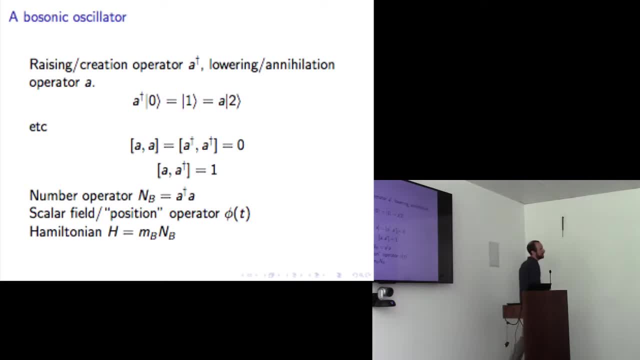 as the creation operator because it's bringing in a particle right. You apply that, apply that operator and you create a particle, A lowering operator, which is the annihilating annihilation operator in quantum field theory terms. And the thing that makes this the bosonic oscillator is that those creation and annihilation 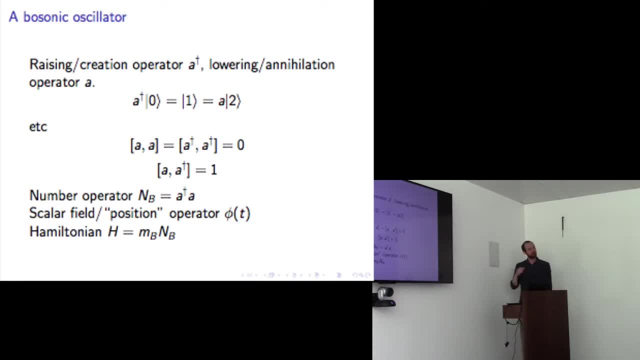 operators obey regular commutation relations as opposed to anti-commutation relations, which is what's going to happen to the fermion oscillator, Right, Okay, Now we can come up with an observable constructed by just you know, putting a dagger in front. 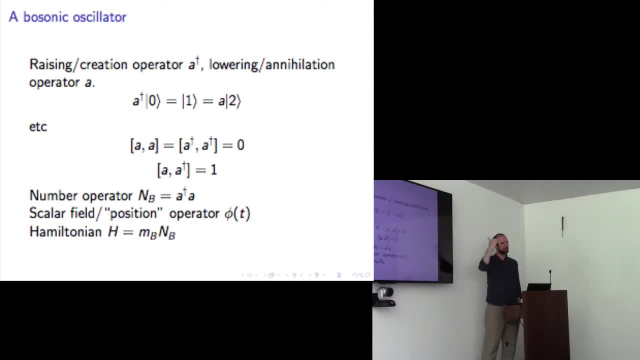 of a, which is going to give us the number of particles, That is to say, it'll tell us how many excitations there are in the oscillator And, as I said before, we're thinking of the position operator as the scalar field. 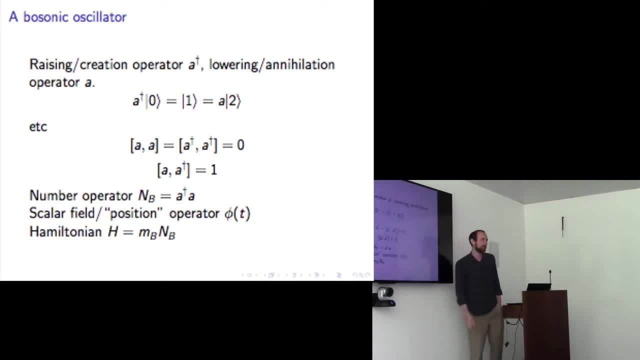 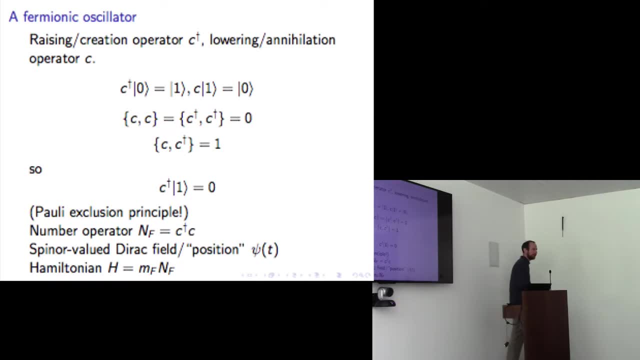 And all the energy is going to be in the mass of the particles, So the Hamiltonian is going to be the mass of one boson times that boson number operator. All right, The fermion oscillator is a little bit less familiar, but it's still really similar. 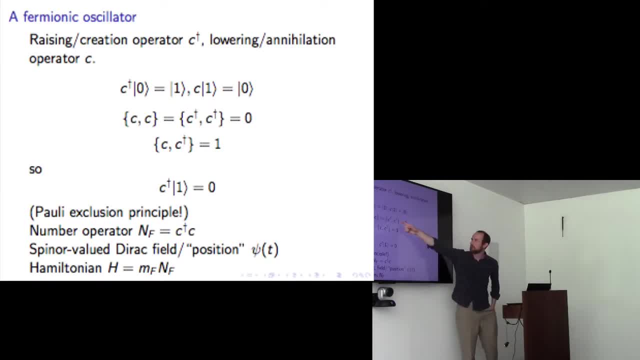 The difference is: instead of applying commutation relations, we're going to be using the creation and annihilation operators, So we'll use C instead of A for the boson creation and annihilation operators. Instead of applying commutation relations, we require that they satisfy anti-commutation. 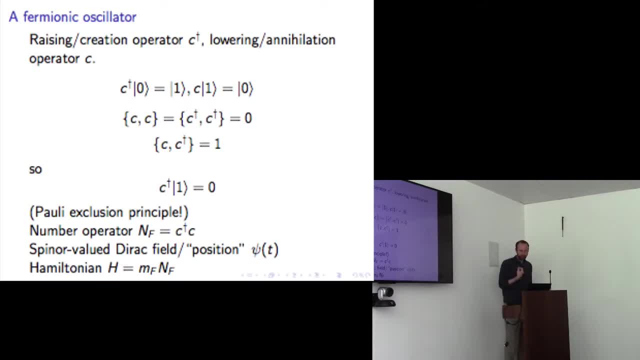 relations, Okay. And that has a consequence which is sort of physically evocative, which is, if I apply the fermion oscillator creation operator to the state that R is in Right, If it already has a fermion in it, it already is at the first energy level- then I get nothing. 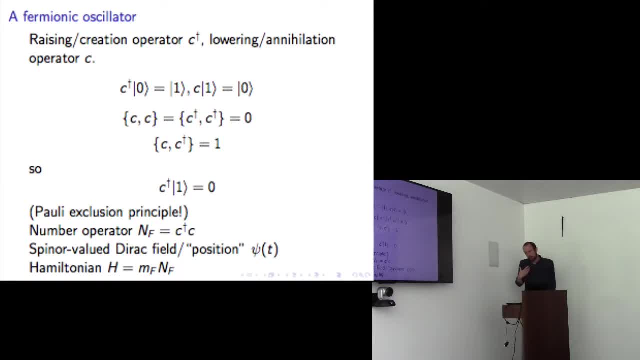 back, Right. So the energy levels available to the fermion oscillator are just the ground state and the first energy level. So you can only have one fermion in this oscillator, Right. So it's an exclusion principle going on here. So we already see some kind of fermion behavior in this thing. 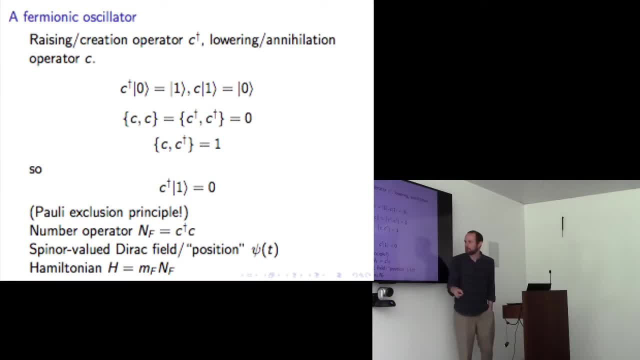 And then we can define the fermion number operator, just like we did for the boson. The quote- unquote- position operator is going to be a little different. It's going to be a spinner valued position- quote unquote instead of a scalar value position. 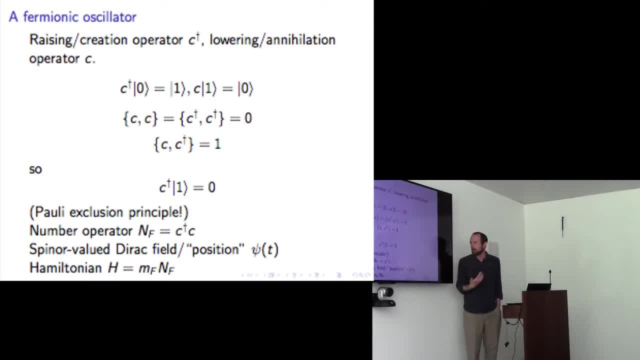 That won't be especially important for what we're talking about, But I'll use psi of t for it, just like we use for a fermion field operator, Right? So that's going to be the direct kind of version of a field operator here. 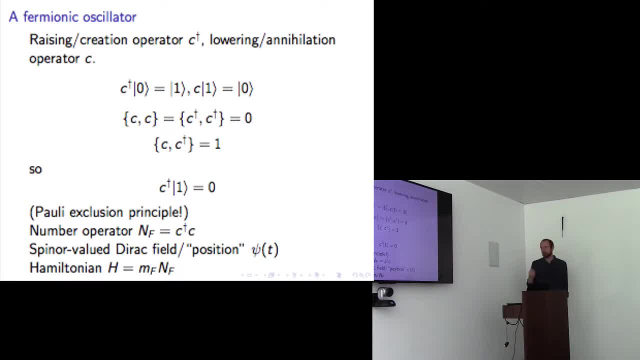 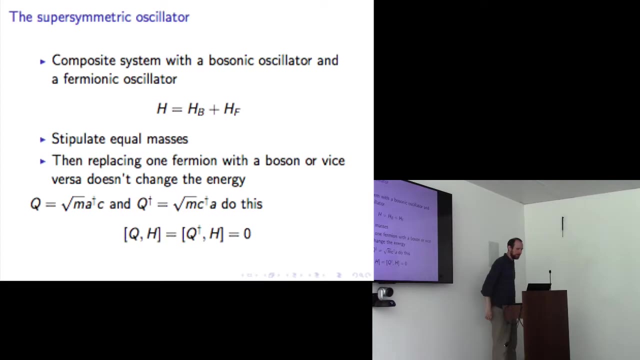 And we come up with a Hamiltonian, just like we did for the boson, where we multiply the fermion mass by the fermion number operator, And that number operator again is just going to have eigenstates of zero and one, because you can only get have zero fermions or one fermion. 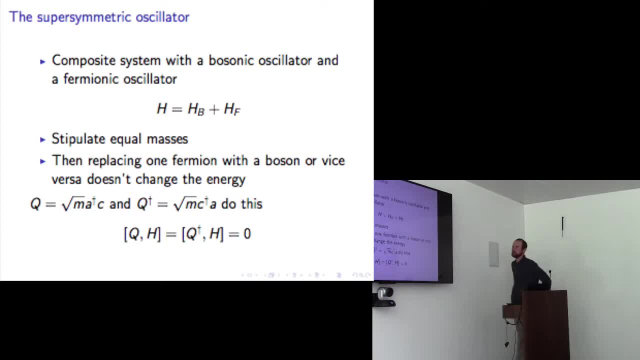 Now supersymmetry. See, we're not very far in and we can already tell you what supersymmetry is. Right, How do I make up a supersymmetric oscillator? Well, I create a composite system. Right, Just using the usual tensor product way to come up with a composite system. 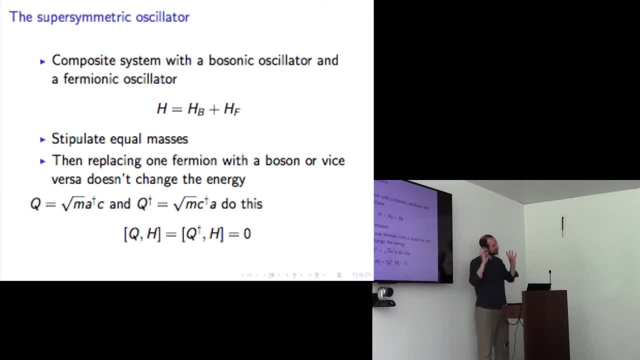 And I put in a boson- oscillator, tensor product that thing- with a fermionic oscillator. So I got a composite system And we call it supersymmetric. Well, what's the only difference between the boson and the fermion as far as their energy? 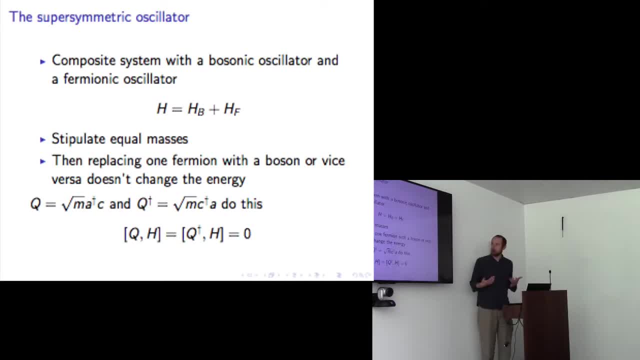 goes, The only difference is, well, OK, well, the Hamiltonian, you know, is the sum of the two Hamiltonians, Right? So the only difference between the two oscillators, in terms of their, the things that we can notice with our energy observable, is the mass of the boson versus the mass of the fermion. 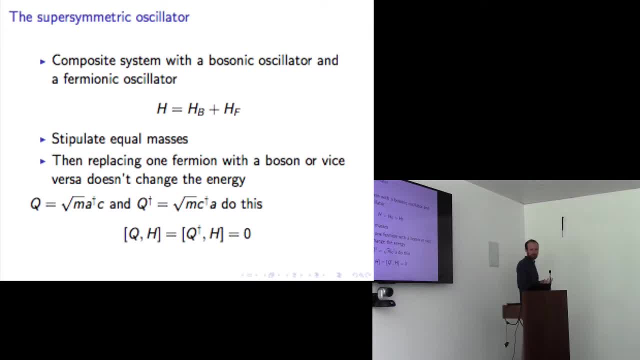 So if we stipulate the masses are equal, then replacing one fermion with one boson or vice versa can never change the energy. And I can define these operators Q and Q dagger. So Q right is going to remove a fermion and add a boson. 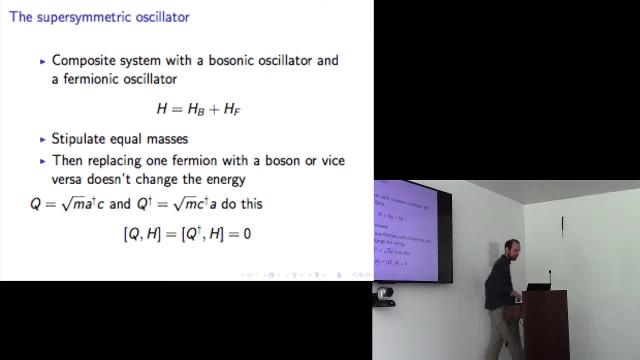 It's, you know, we have this square root of M thing out front to normalize it. You know you don't need that technically, but it's, you know, makes things more fun and easier to do. And Q dagger is going to remove a boson and add a fermion. 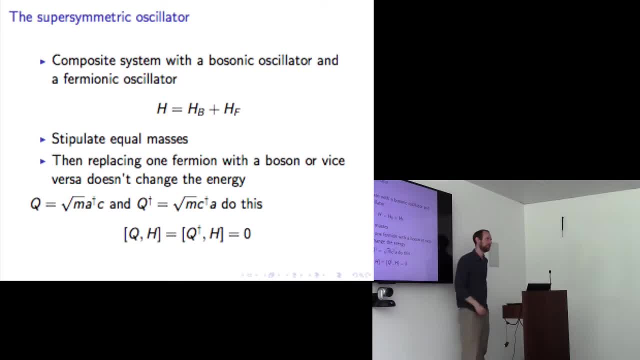 These things both commute with the Hamiltonian, which, you know, is the sure sign that they are symmetries of the theory. Right So Q and Q dagger? well that they generate symmetries. Right So Q and Q dagger are the generators of the symmetry for this theory. 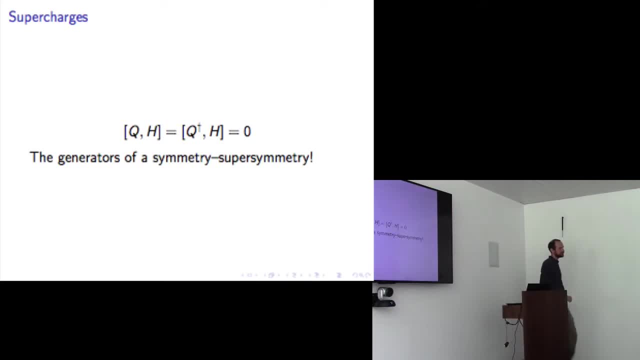 Supersymmetry. Yeah, So if we did this with two harmonic oscillators, just two bosonic harmonic oscillators, we took the Hilbert space for one of them, the tensor product, with the Hilbert space for the other, we would think of these as having like, in terms of ontology, having two oscillators. 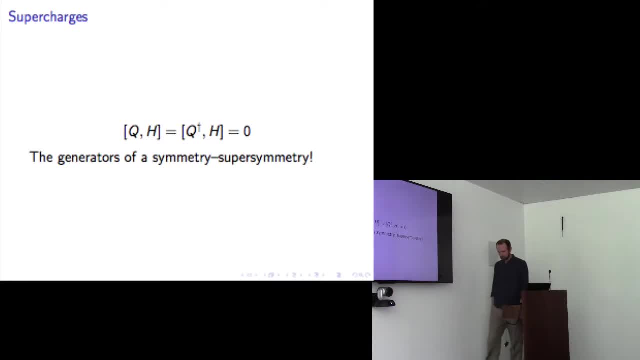 and we could possibly couple these two oscillators. Now this looks a lot like the same construction. So we have a bosonic oscillator and a fermionic oscillator. So what in this? maybe we'll return to this, but what? how do we get to this ontological 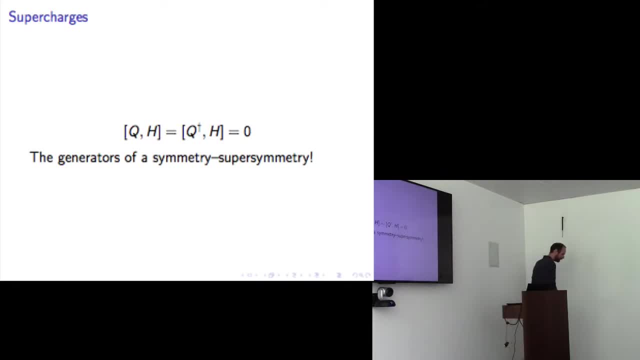 picture where this is actually one supersymmetric oscillator rather than one bosonic and one fermionic oscillator. Yeah, It's an interesting kind of like, right? so it's an interesting question here, You know, and there's a lot of levels to it- about what sort of you know, what sort of 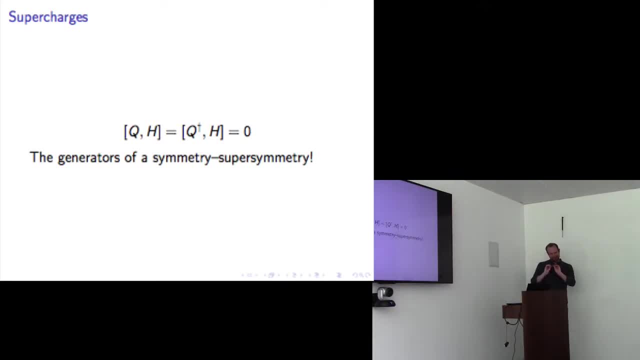 what kind of like ontological input goes into constructing the model? Yeah, I think so. in that case, I would say, whether you want to call it one supersymmetric oscillator or a system of two oscillators, a system of two coupled oscillators, that in. 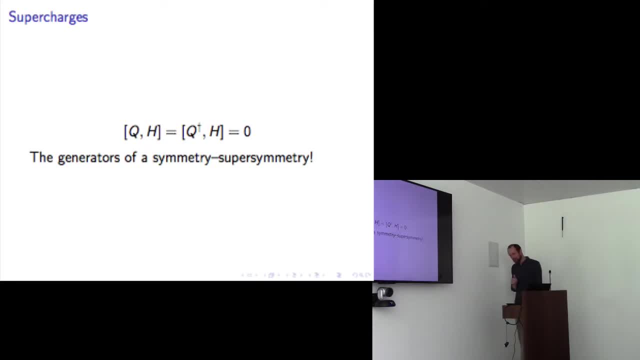 a sense exhibits supersymmetry. that's where I think you might be getting into. this is a purely semantic question territory. What would be in common with that system would be that there would be a symmetry of that system that interchanges a particle from the one oscillator to the other oscillator. 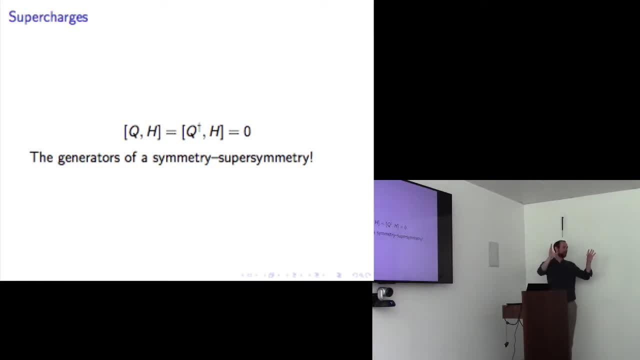 right, the system where it was just two bosonic oscillators that were coupled with equal masses And so well, I mean they're not really coupled in any interaction sense, right, but they're a composite system. So in that case I would say the physically important thing to keep in mind with that, 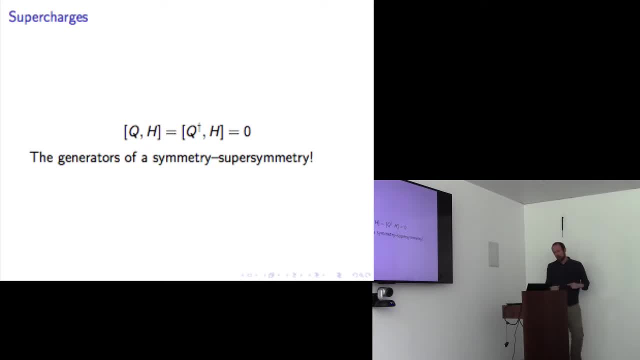 system of two boson oscillators is that they're not just you know, they're not just you want to say you know, they're just quantum mechanics, they're not just quantum theory. I think the only difference between a system of two boson oscillators is: you know, from 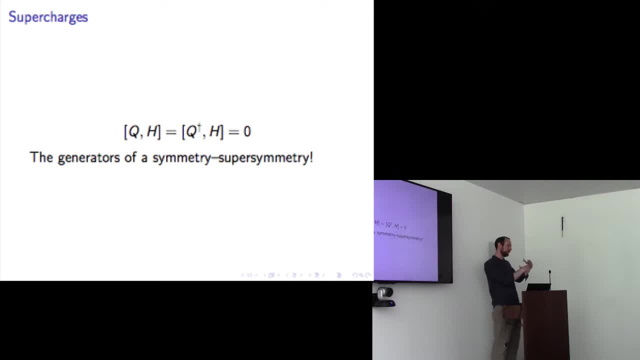 the point of view of quantum mechanics or quantum field theory, which might not be all the physical facts there are, if you're something like abomine or something, but from the point of view of purely canonical formalism, there's no real physical difference between having 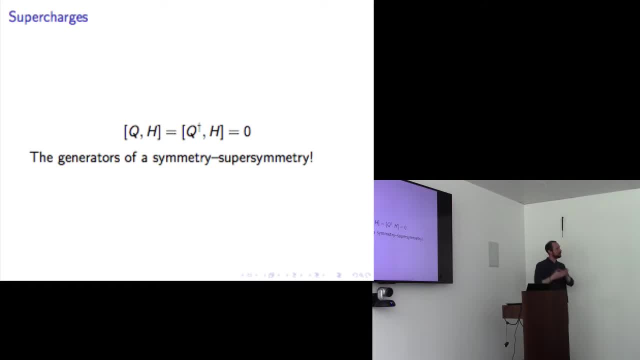 one excitation in this oscillator and none in this one, having one excitation in this oscillator and none in this, one model as one where there's two oscillators, a Bose on and a Fermi on one in some sense, and there's no fact of the matter about whether you have one excitation in the Fermi oscillator. 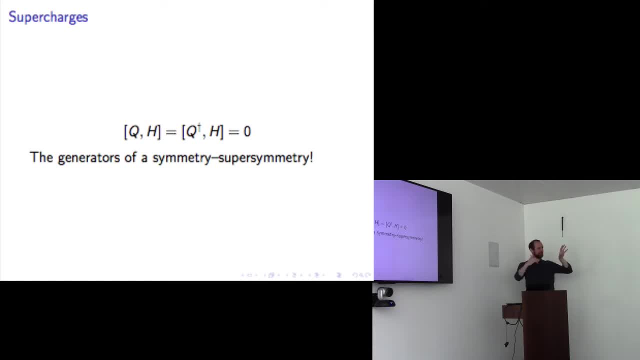 and zero in the Bose, or one excitation in the Bose oscillator and zero in the Fermi. That's another useful way to think about this and it might be helpful And indeed right. there are going to be some invariant facts about, for example, like: 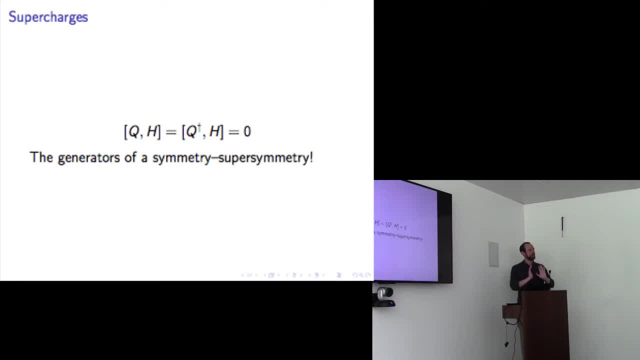 you know, for example, if I have a system that I write up as applying, I write up the state applying the Bose on creation operator like five times the ground state. it is a supersymmetry invariant fact that there are more Bose ons in that system than Fermi ons. 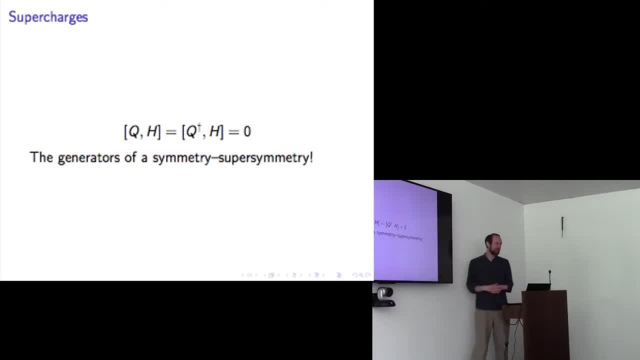 for example, right. So yeah, it's. yeah, that's a really, really helpful clarification question, and I think there's nothing wrong with thinking. I think there's nothing wrong with thinking of this as a system of two coupled oscillators. 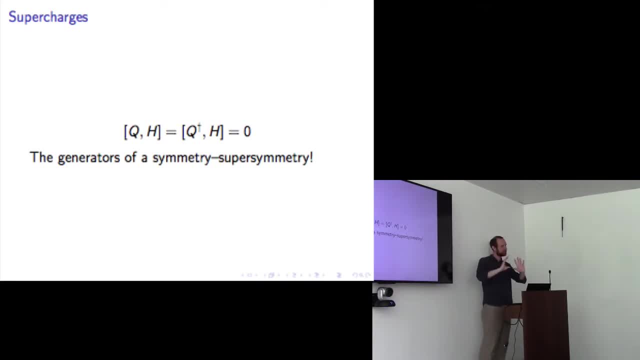 rather than just, I mean two again, I shouldn't say coupled, but a system of two oscillators that are composite as opposed to like one oscillator, right? Good, good, Okay, so this all looks really normal, right. 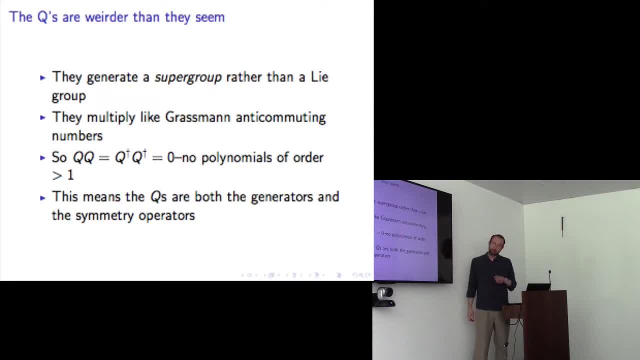 We've just got a regular symmetry. boring, but right. the Q operators are stranger than they seem. The reason they're stranger? The reason they're stranger than they seem, in a sense, is because they turn scalars into spinners and vice versa, right? 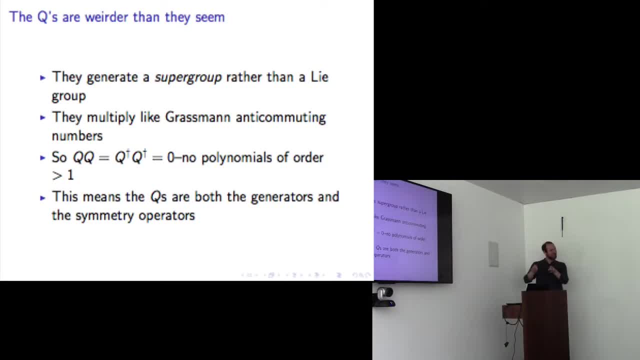 So that means that they have to be spinners in that sense, right, If you have an entity that you multiply something by and it turns it from a scalar into a spinner, then that thing that you are using for the multiplication has to be spinner value itself. 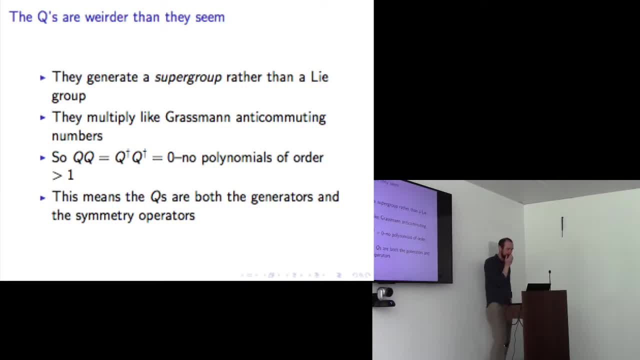 right, So the Qs have to multiply like spinners. So the Qs have to multiply like spinners themselves, and that's what makes them strange. So they generate what's called a supergroup rather than a lead group, right, If they multiplied like. you know in some sense that they, if they didn't multiply like 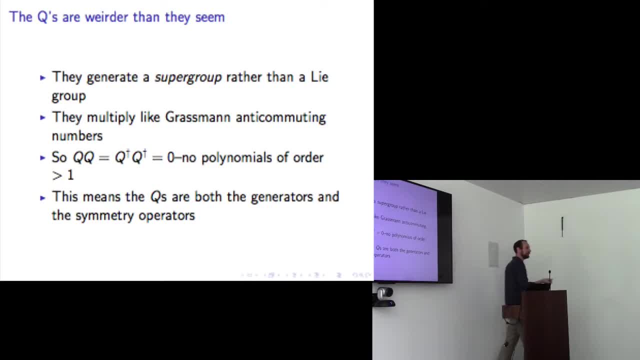 spinners. if they multiplied like scalars, they would be a regular lead group, right. But because they multiply like spinners, they generate a supergroup, And that is to say, they generate a supergroup of objects that are characterized by their 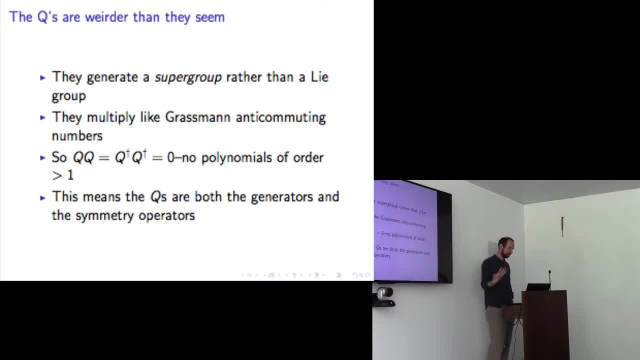 anti-commutators rather than by spinners. Okay, Another way to put this is that the Qs multiply like. so. this is. this is the part of the Suzy stuff that is not going to seem super familiar from your intro: quantum mechanics textbooks. 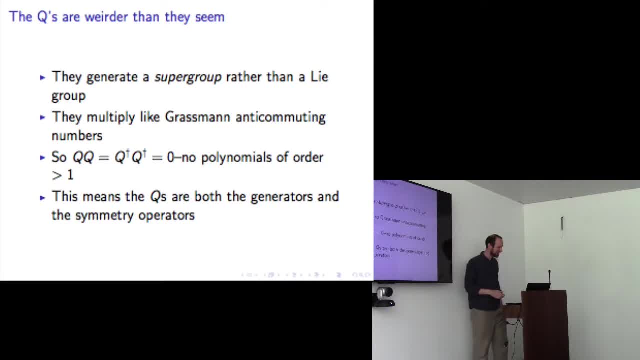 Not coincidentally, it's also the part that I feel the least comfortable with myself. You know, as I always tell people, I'm not that great at math. But you know I'm not that great at math. But the Qs multiply like Grassman-valued anti-commuting numbers. okay. 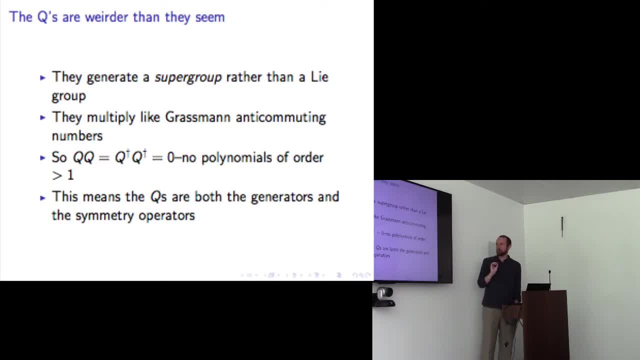 That means that you know so any. so in particular, right, if I take Q squared or Q dagger squared, okay, the rule is going to say that the anti-commutation, The anti-commutation rule is going to say that QQ plus, you know, QQ equals zero, right. 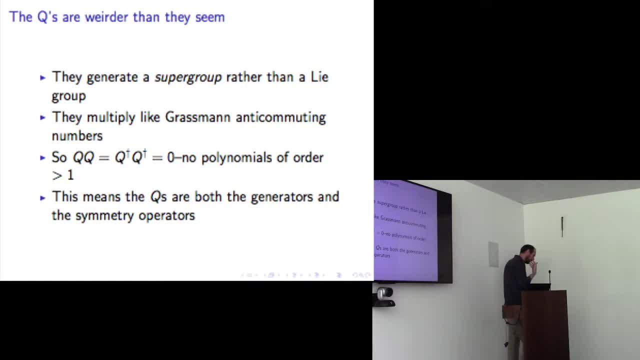 In general, it's going to be like Grassman numbers are going to obey. it's good that you have this right- Two Grassman numbers, A and B, are going to obey the rule of the anti-commutator equals zero. 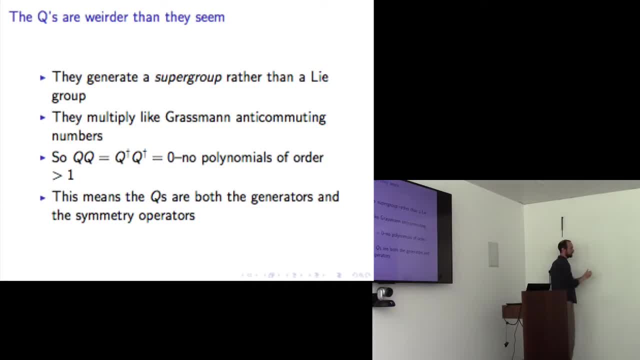 which is say, AB plus BA equals zero right. So given that Q and Q dagger are like that, you know, no Grassman number can have a non-zero square right. So you can't have polynomials of order greater than one in the Qs or in any Grassman-valued object. 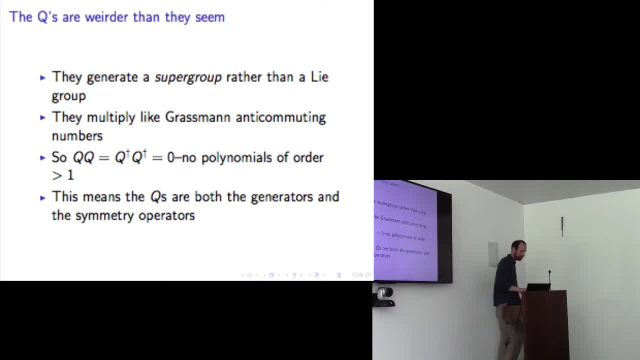 And that's kind of funny because, you know, let's suppose I was trying, you know, to exponentiate Q, right, you know? because if I'm thinking of Q as the generator of the symmetry, I'm thinking, well, you know, like something like the exponential of Q. okay, 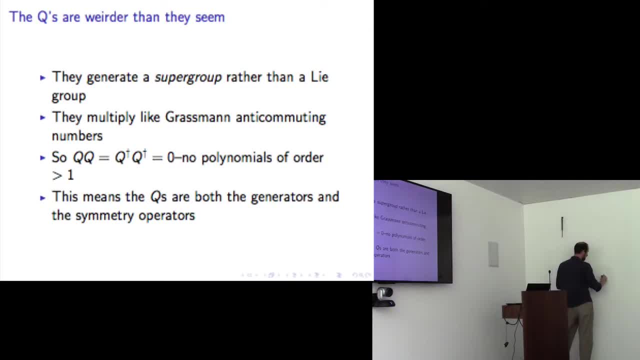 Well, that's just going to be like one plus Q. you know some. you know like some, like factor times Q have some other factor times Q squared plus you know Q cubed, but uh-oh, these are all. 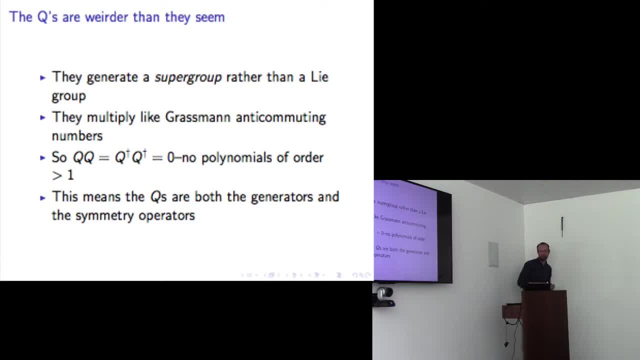 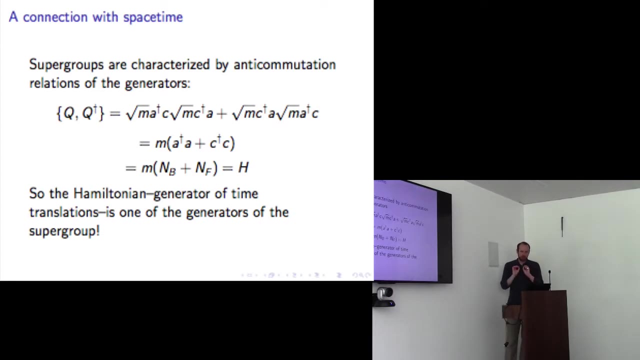 gone because you can't have higher order polynomials in these things. So really, there's a sense in which the Qs are both the generators and the operators that implement the symmetry. Okay, And here's where. so here's where we start to see the suggestion of this superspace structure. 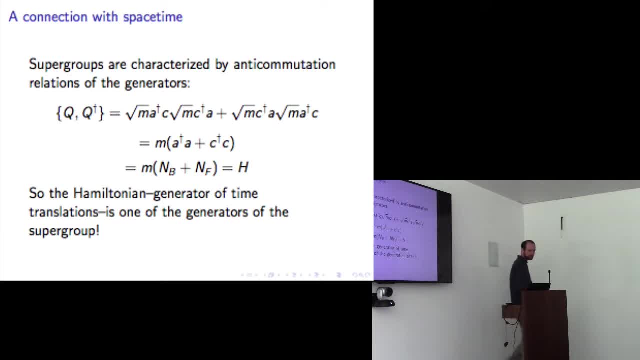 Right, We'll see a connection now with spacetime. Unlike a regular Lie group, a supergroup, as I was saying, is characterized by anti-commutation relations rather than commutation relations of the generators. Okay, So, um, oh, I think I said no, I didn't like that. 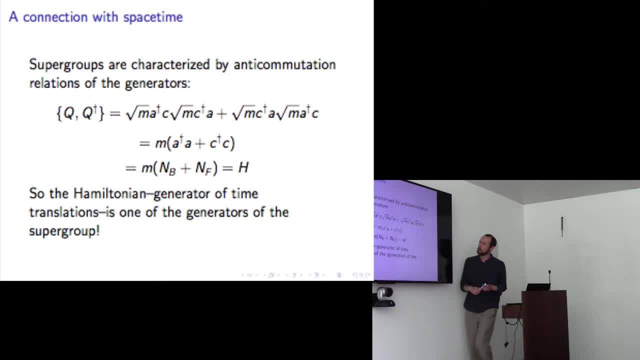 So so Q and Q dagger right. um are going to have these non-trivial anti-commutation relations, And you know if you're going to have these non-trivial anti-commutation relations. you know, if you're going to have these non-trivial anti-commutation relations, you're going. 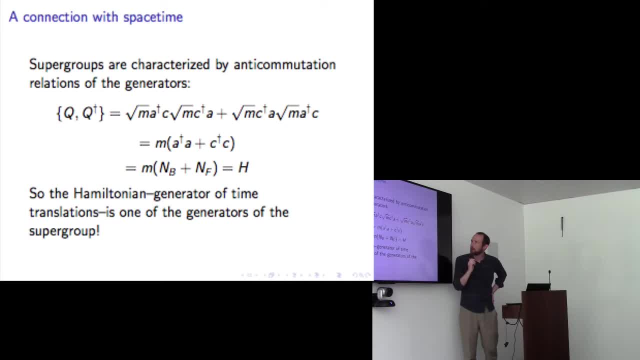 to have these non-trivial anti-commutation relations. So if you kind of go through it right, it turns out that, um, the anti-commutator of Q and Q dagger is going to be, uh, the mass times, the boson non-brapitor plus the freemium. 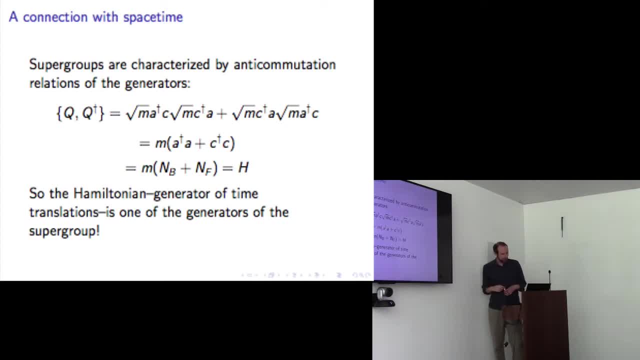 non-brapitor, which is just the Hamiltonian. Okay, Um, so the Hamiltonian, which is the generator of time translations, is, uh, one of the generators of the superdome, Right? Um, if it, if it fits into the anti-commutation relations with superdome, then it's going. 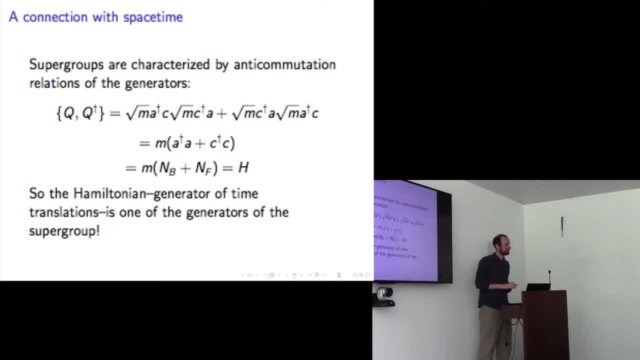 to be some of the generators, It must itself be another one of the generators. Okay, So I can't build a group for this symmetry without including the time translations in that group. Right, In a sense, the supersymmetry transformations have to be thought of as a part of a group. 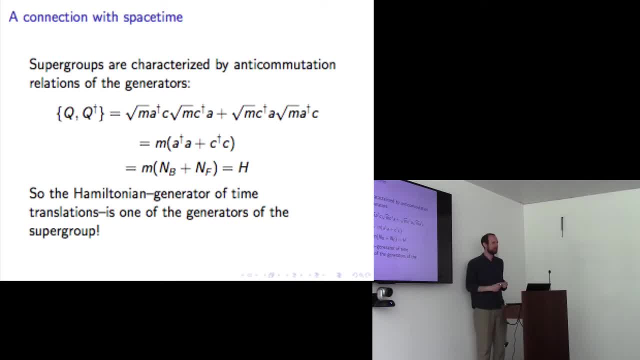 of symmetry transformations. that includes the time translations. You know, remember, we're just talking about one-dimensional space-time, So the time translations are really like all you have as far as space-time symmetries go. But this generalizes. if I do a supersymmetric field theory on Minkowski space, I'm going 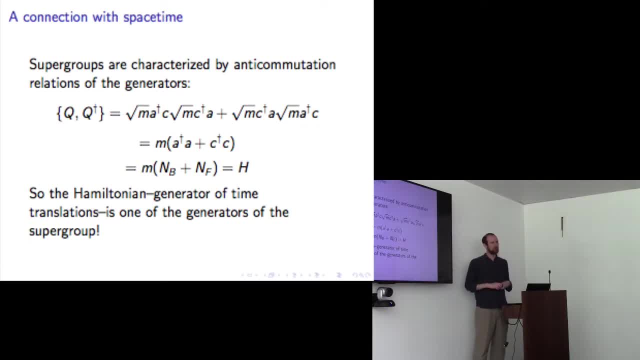 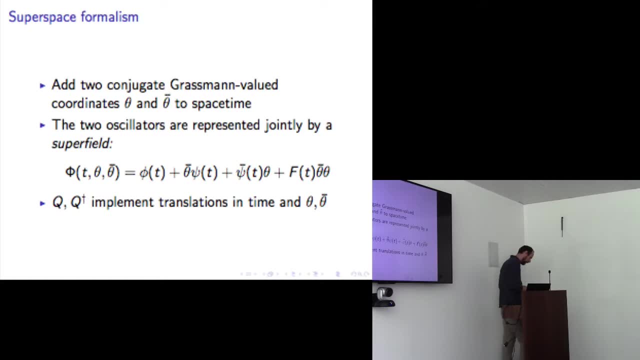 to end up with a group called the super Poincare group, which includes the whole group of space-time symmetries in this subgroup. Okay, Now that's suggestive, Right, But maybe the thought goes I should try to come up with a formalism where 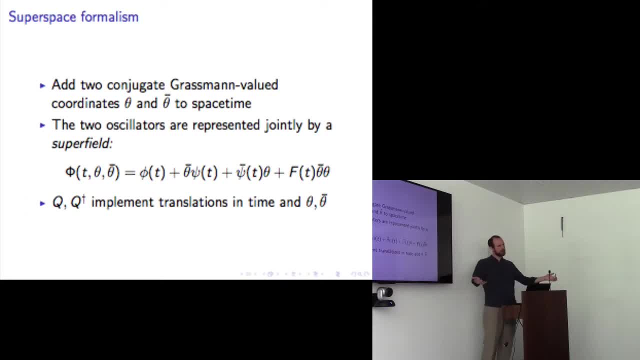 I have some generalization of space-time, which is the entity that is invariant under this supersymmetry. you know this kind of supergroup which includes the supersymmetry transformations and also the space-time symmetry transformations, And I can do this by adding Grasman-Valley coordinates to space-time. 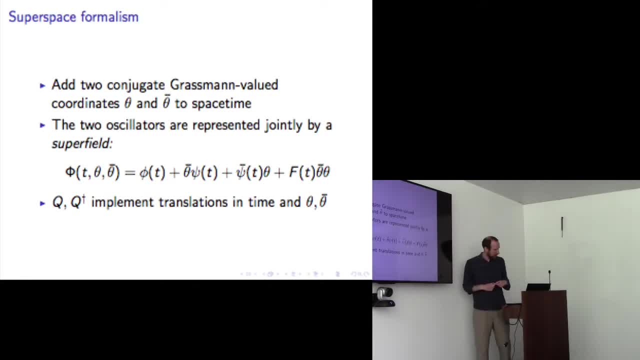 So in this case I'm going to add two coordinates, And You can think of them as conjugate. That's why I have theta and theta-bar written on there, right? You know essentially what I'm doing here. 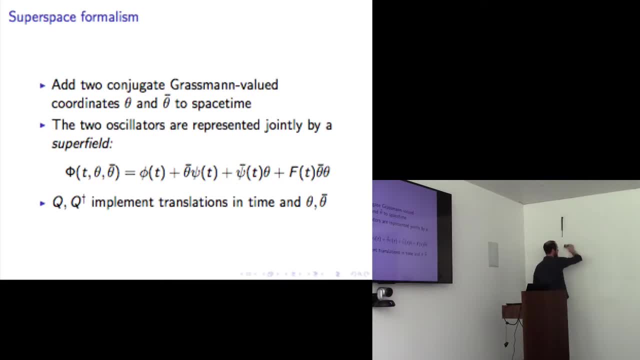 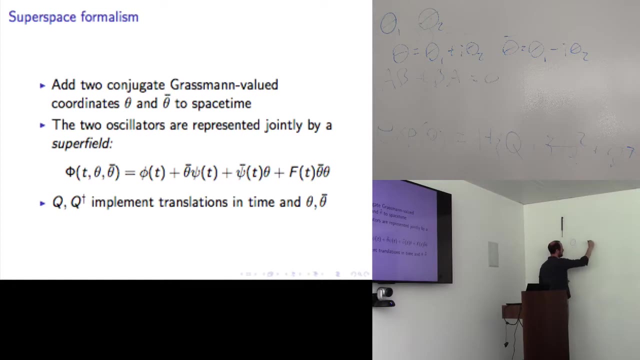 This is a trick that gets used all the time in textbooks on this topic and almost never explained. It's not very basic, But what I'm really doing is I'm saying there's two Grasman-valued variables, theta-1 and theta-2.. 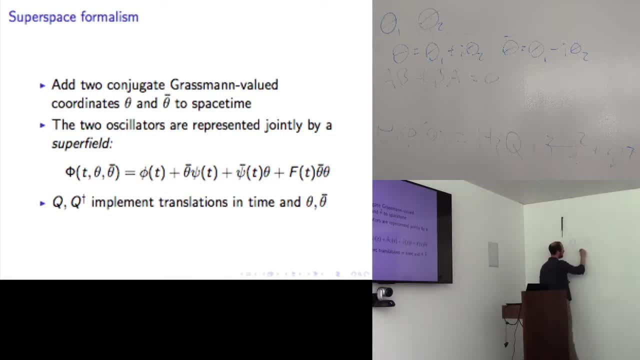 And then I'm saying: You know, I'm renaming them so that theta is theta-1 plus i theta-2, and theta-bar is theta-1 minus i theta-2, right, So then I have. You know, it just makes it easier to work with them if they are conjugate to each other. 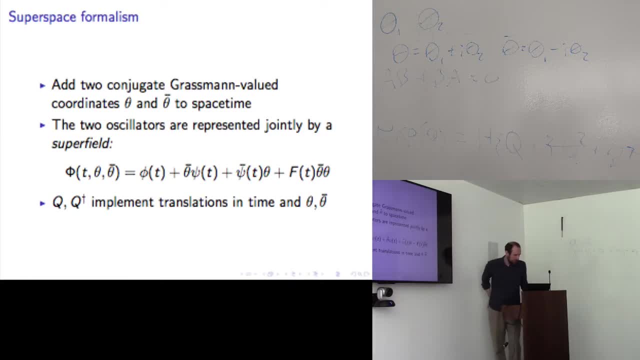 So I've relabeled them that way. That's what I've done. So there, I've just saved you some time when you pick up your first actual textbook that's going to be used. It talks about supersymmetry. It does not explain what I just told you. 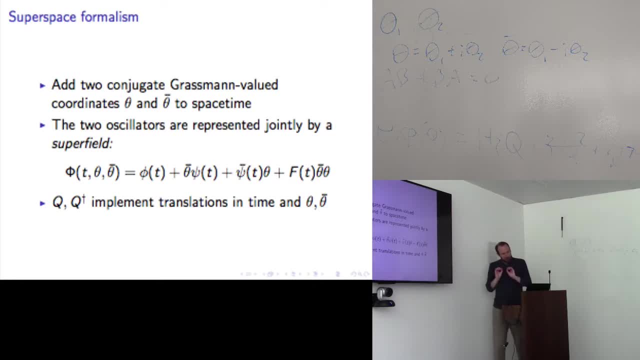 So now, at this point, right, remember, I have these two oscillators that are ordinarily represented separately by these fields: little phi and psi. right, Well, now I can come up with an object called a superfield, big phi, which is not a field. 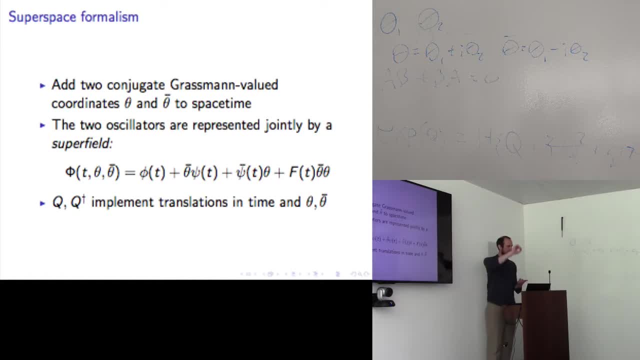 over spacetime, which is just the t-axis, Right. Right, It's a toy model, It's a field over spacetime, plus these Grassman value coordinates, right, And we're going to call that thing superspace. It's spacetime t plus those theta and theta-bar coordinates. 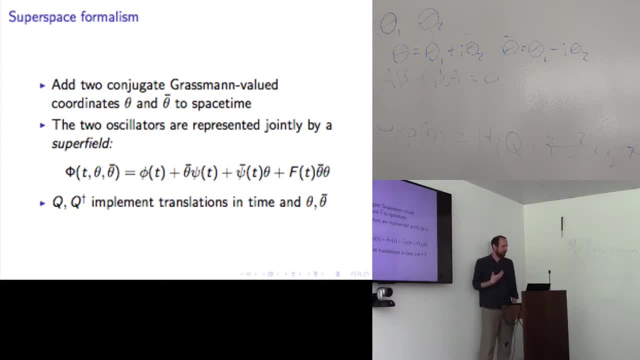 And I can represent the fields of the two oscillators jointly using this superfield big phi. I'll just call it phi from now on, And you know it's just the boson field plus the fermion field, multiplied by the two. 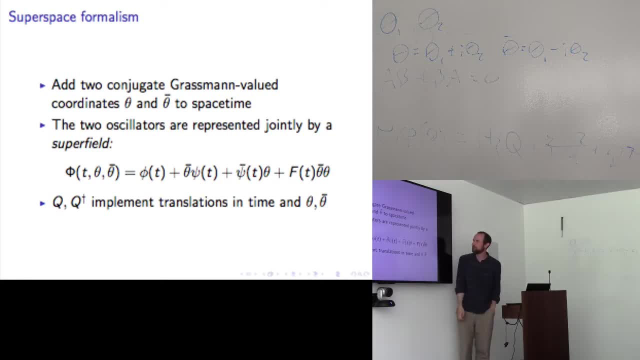 theta coordinates, And then I add what's called this extra auxiliary field at the end. That's added to make calculations easier. When you construct the observables from the superfield, this drops out, and it doesn't matter what you use for it. 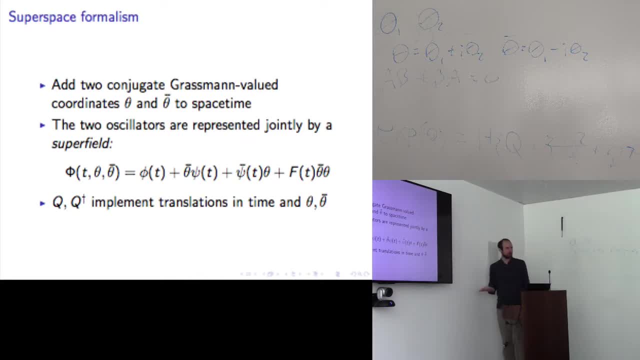 So it's kind of people call it the dummy field. sometimes I'm actually a little curious whether there might be some kind of interesting physical interpretation to this thing. But one thing to keep in mind, though, is that, from the point of view of what's invariant, 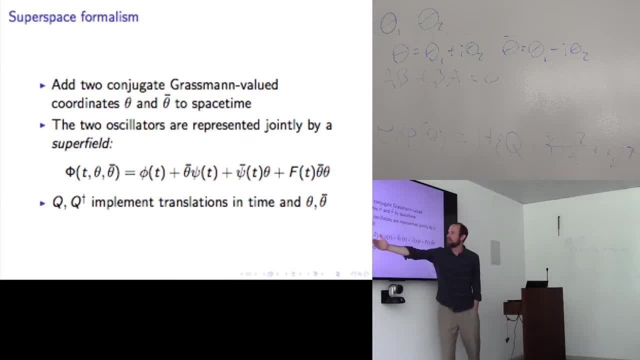 under supersymmetry. what's invariant is this, and not how it decomposes into this stuff, Right? So when you are thinking about things from this superspace perspective, you don't want to think of these components of the superfield as being separate things. 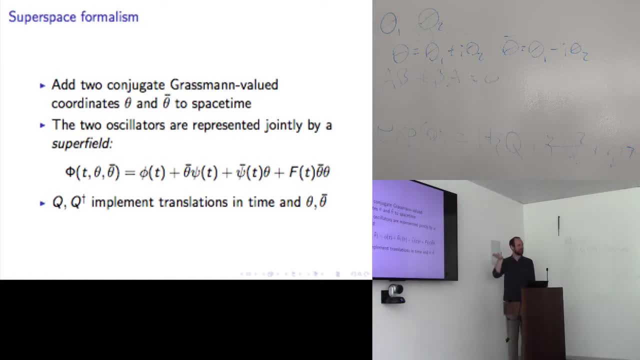 That's the kind of the anti-superspace way of thinking about this thing. right From the superspace perspective, it's really this: and then we can coordinate-ize, in a sense, the superspace and, with a choice of coordinates, break it down into these components. 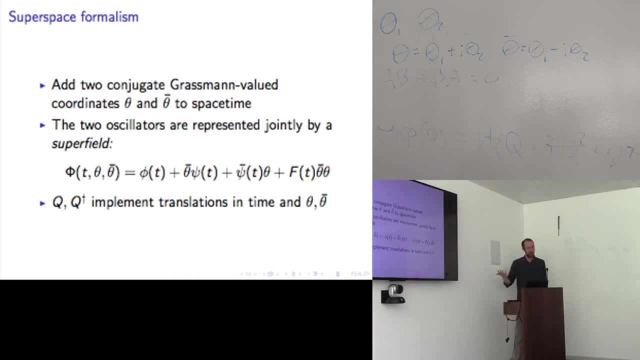 But the whole superfield is supposed to be this, Right, It's supposed to be what's fundamental on this superspace form, And then what Q and Q dagger do is actually implement translations on this space of T, theta and theta bar Right. 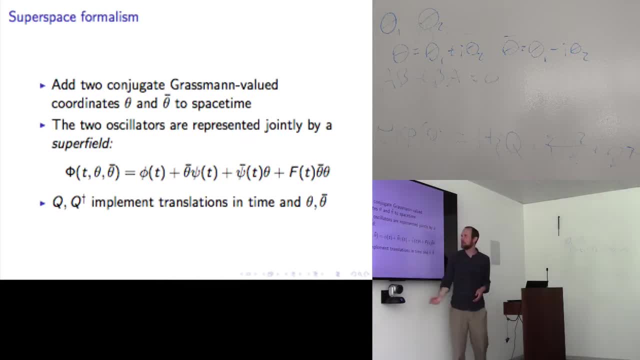 They translate you along theta and theta bar. So, for example, you might be at theta equals zero and theta bar equals zero, in which case the superfield is just constituted by the boson field. Right, You might say, like I only have excitation in the boson part of the oscillator. 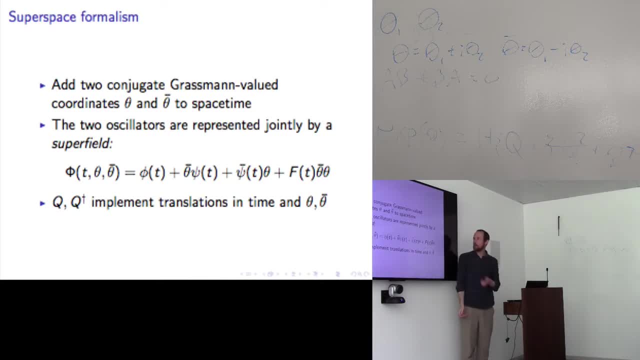 So this is a pure boson state. Well then, how do I implement a supersymmetry transformation? How do I introduce fermions into this system? Well, I have to create a non-zero fermi field, right, And that involves- oh, I've got to translate myself away from- theta equals zero. 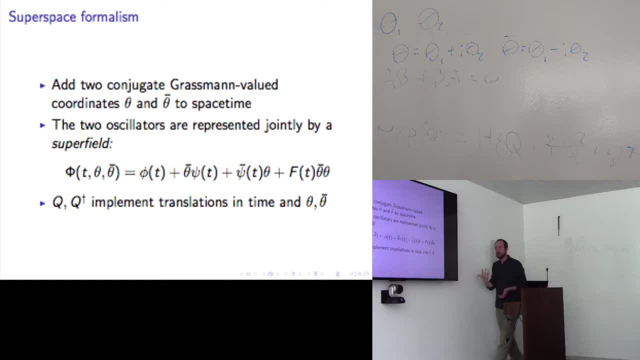 Okay, So that's, that's the sort of intuitive way to understand that these supersymmetry generators, right, These Q's, implement translations in superspace, And by coincidence, you know, because of the fact that they don't, because of the fact, 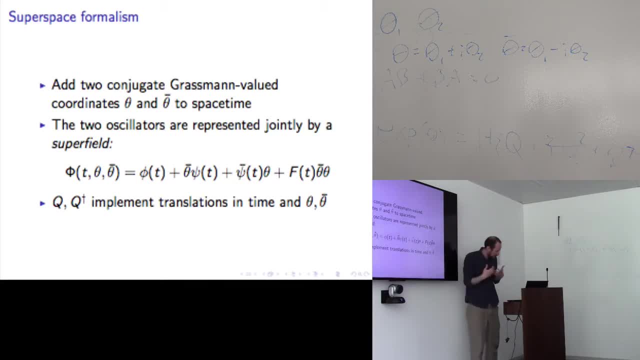 that they have non-trivial anti-commutation relations with the Hamiltonian. they also move you in time. So if you, if you do two supersymmetry translations in a row, you're going to. that's going to constitute time translation in this case. 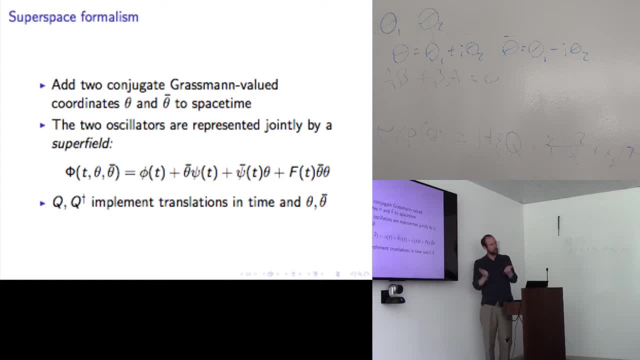 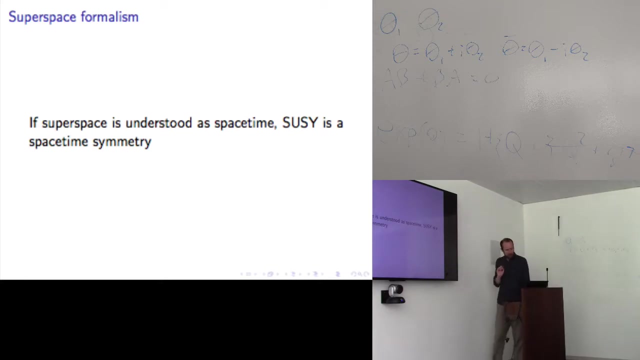 And in general in the super Poincare group. two supersymmetry transformations are going to be a space-time translation. So sometimes physicists use the slogan: a supersymmetry transformation is the square root of a space-time translation. Okay, Now if we understand superspace as supersymmetry. 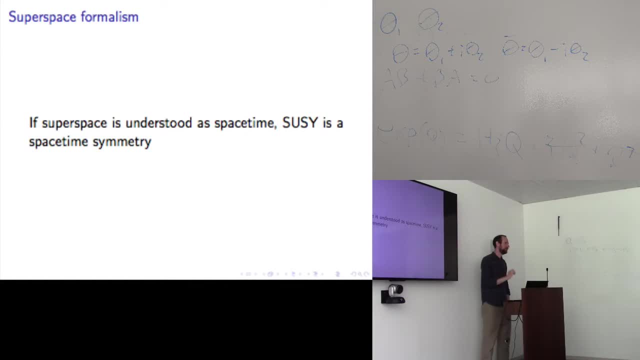 Okay, If we understand superspace as spacetime, SUSY is a spacetime symmetry, Right, That's the way. that's the way to think about the stuff I just told you. Um, now there's a question, right, Should we think of it that way? 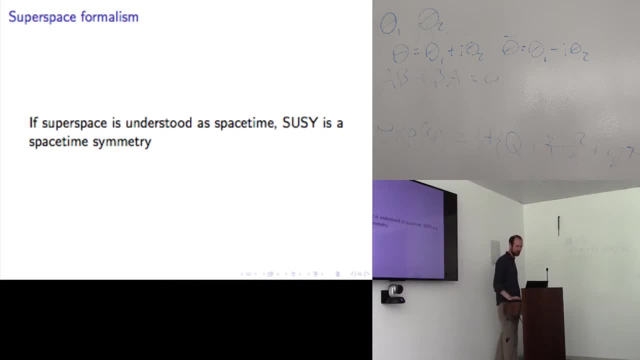 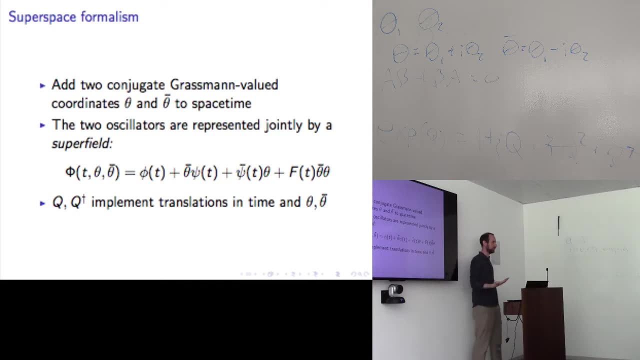 That's the kind of one of the kind of philosophical questions in the neighborhood here. But it is available to us, at least as a notational tool, to think of it that way, to think of SUSY as a spacetime symmetry. The question is, is that the right way? 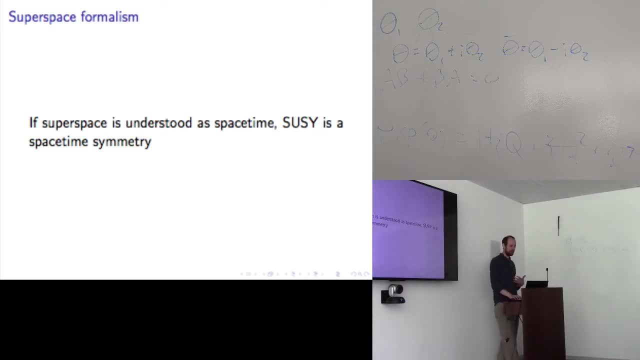 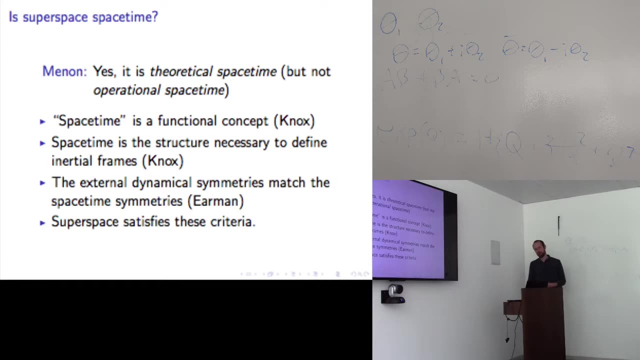 From a kind of ontological- or you know, understanding the theory in the best way- kind of perspective, Is superspace really spacetime? Um so Tushar Menon has, has you know, written on this topic. You can find his paper on the PhilSci Archive and in his forthcoming Nick and Chris Utrich's. 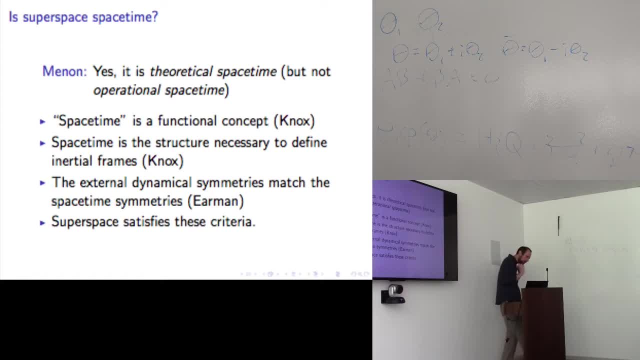 new anthology. He gives an answer, you know, which is a sort of classic answer. He gives an answer. This is probably the most qualified. yes, right, Um Tushar breaks up spacetime into two parts, one of which is the role of theoretical spacetime. 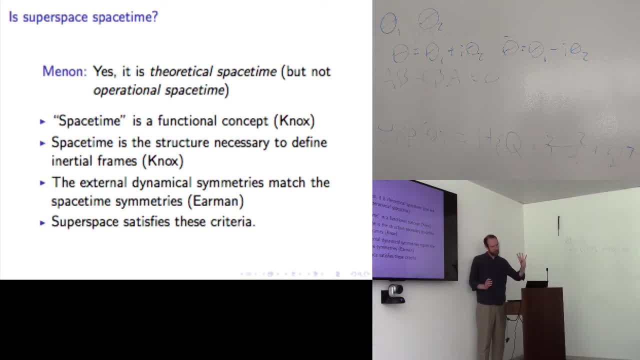 which is essentially the spacetime structure that gives us the essentially the structure of um geometric symmetries of the systems, right, And that's that's what he calls theoretical spacetime. And you know, of course, a lot of the stuff we've already seen provides reasons to think. 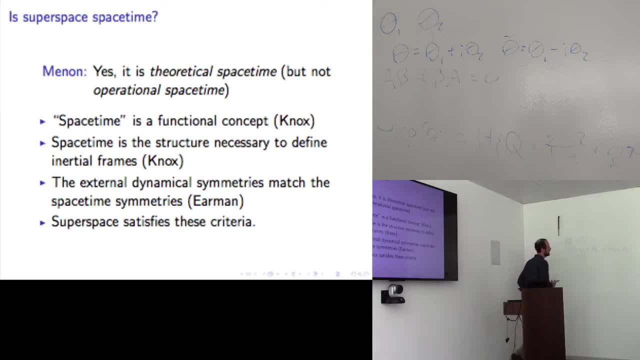 yeah, superspace is theoretical spacetime in that sense, right? Uh, we, we believe it, CARL EHRENFELDizzito. He also points out it's not really operational space-time in a sense. So operational space-time he means the space-time that we measure with ordinary rods and clocks. 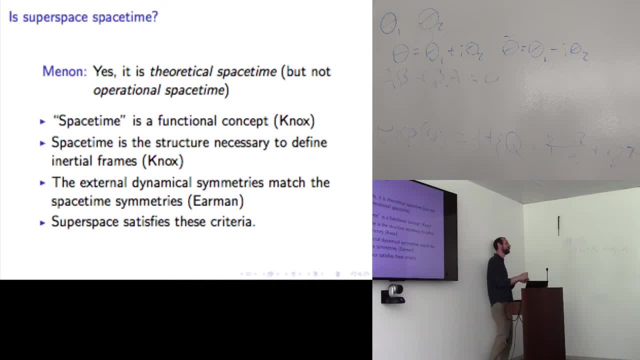 and light rays and stuff like that. Now there's a sense in which we do, of course, measure the space we live in with those things, but there's no physically intuitive sense in which you can build a rod that's going to give you the distances, quote-unquote, along those theta dimensions. 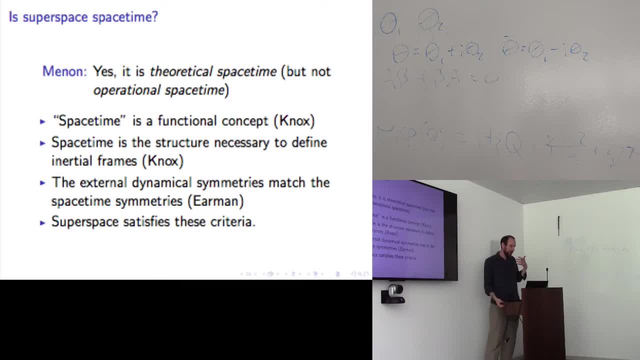 So in that sense it's not operationally illuminating to think of superspace as space-time. So from that point of view, superspace is not space-time. But from the theoretical point of view, in terms of determining the fundamental- well, I don't want to say fundamental, because that gets to the metaphysical issue we were talking about- 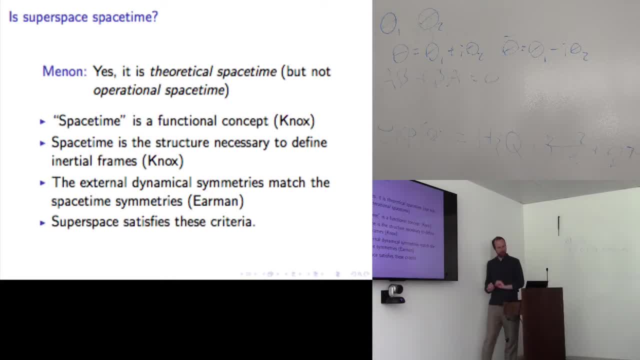 But in terms of thinking about the geometric symmetries of the universe we live in, that should be thought of as the most general geometric symmetries. I'll put Tushari's view that way: Superspace is space-time. 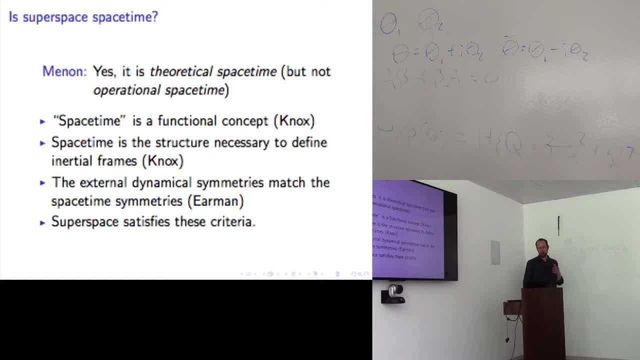 And in addition to this kind of perspective of Zony, he kind of connects this with the space-time functions of Elmer Knox. Right, He points out which Tushari would agree with, but they have somewhat different functional definitions. Knox says space-time is a functional concept. 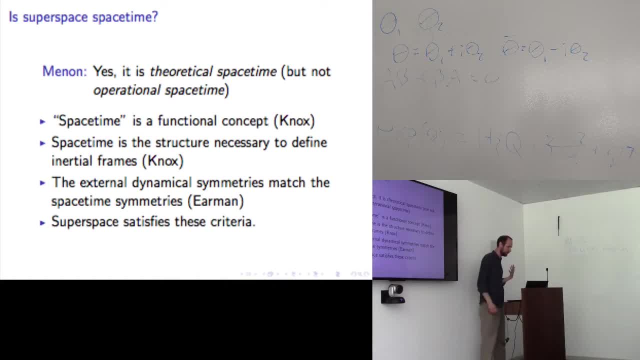 In Knox's case. you know this is one of the things that will be discussed. I gather that James is going to be leading a discussion group on space-time functionalism, which is a cool topic. to state Knox's view in one sentence: 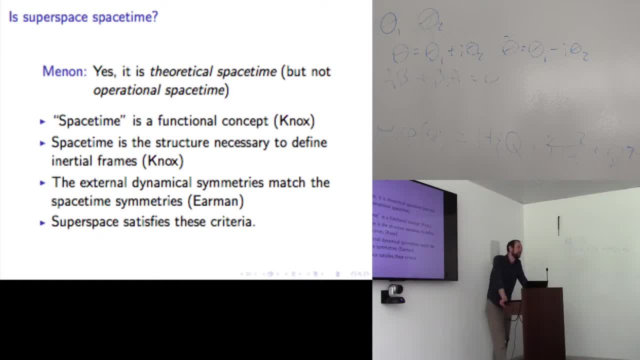 Space-time is a structure necessary to define inertial frames. Knox means local inertial frames, but we're talking we're not talking general relativity right now, so we don't need to focus on that, that qualification. But so Knox's view is that, whatever you might say, 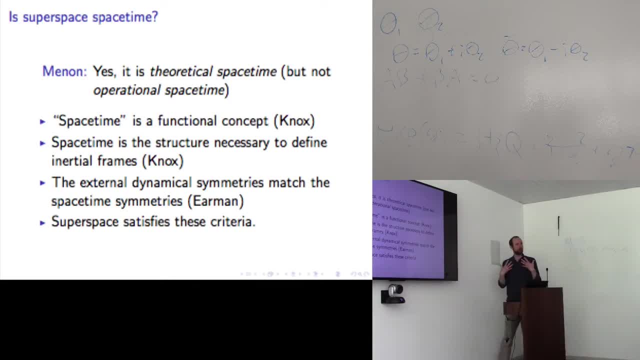 the kind of minimal structure required, the minimal structure you need to posit in order to tell me what the inertial frames are for a given theory. That's the space-time of that theory, All right. Additionally, there's this famous posit. well, really, you know kind of two posits that Ehrman gives. 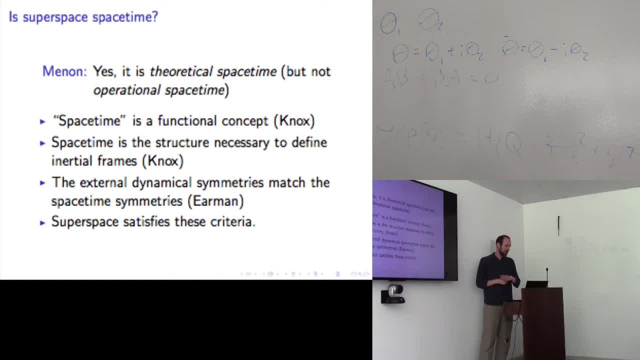 in World Enough and Space-Time, SP1 and SP2, that what Ehrman calls the dynamical symmetries, which we should really think of as the external dynamical symmetries, because he's not talking about like gauge symmetries, for example. 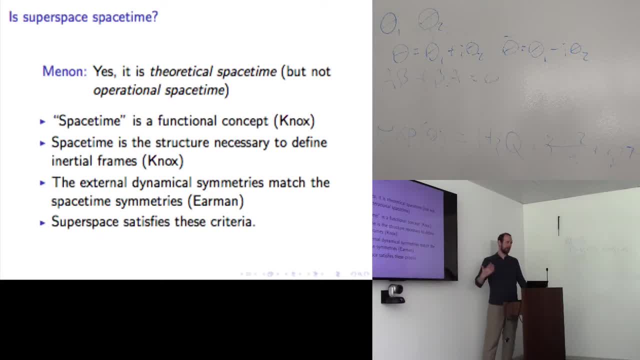 The dynamical symmetries have to match the space-time symmetries, right? So you look at, you look at mechanics, you look at Newton's mechanics and you think, well, we want to posit a space-time for Newton's mechanics. 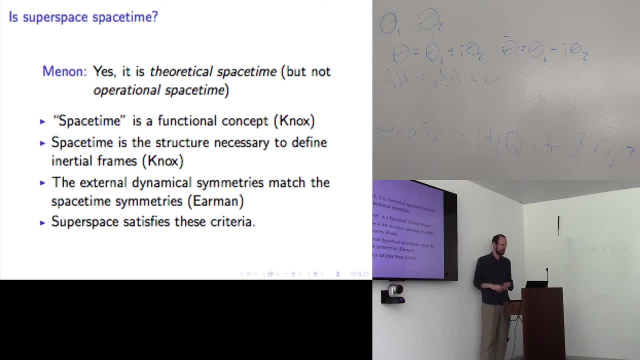 that has the same symmetries as Newton's equation of motion, in some sense right. And Tuchars suggests: well, superspace satisfies these criteria. These should be thought of as the criteria for, or some of the different possible sensible criteria. 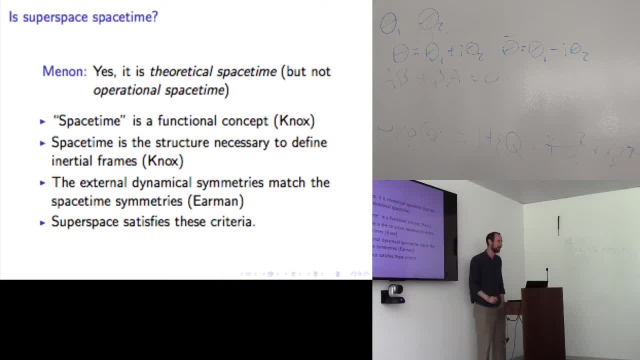 You know Tuchars' own criteria are probably closer to Ehrman's than to Knox's, But these should be thought of as the different possible sensible criteria for what it takes to be theoretical space-time right And the reason why there's a kind of interesting reason. 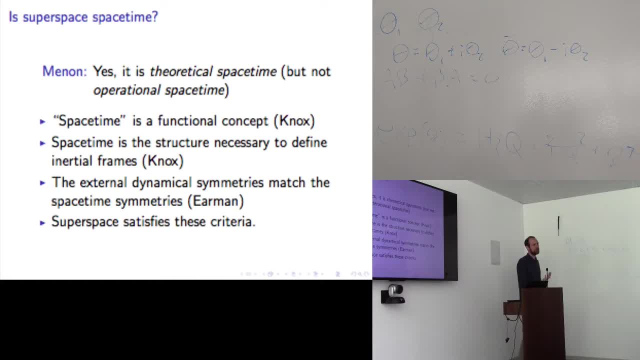 why supersymmetry satisfies Knox's criterion, which I'm not going to go into all the details here, but basically you can define a notion of inertial frames on superspace. they're not force-free frames, right? So because? because what's the definition of force? 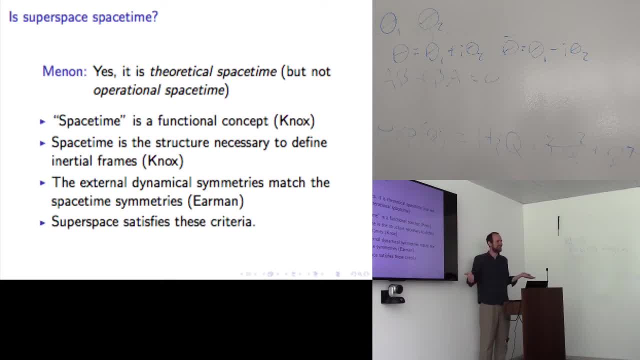 along one of those theta dimensions. That doesn't make any sense. But what's the definition of motion along those dimensions? It doesn't really make a lot of sense. And anyway, we're talking about field theories. so, like force and motion are highly derivative concepts. 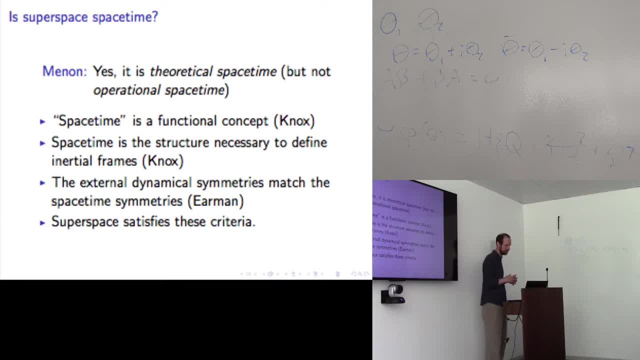 probably anyway, although Chip Stevens would disagree with what I just said, Maybe not with the motion part, but definitely with the force part. But what we do have is a notion of which frames give the simplest formulation of the theory's equations of motion right. 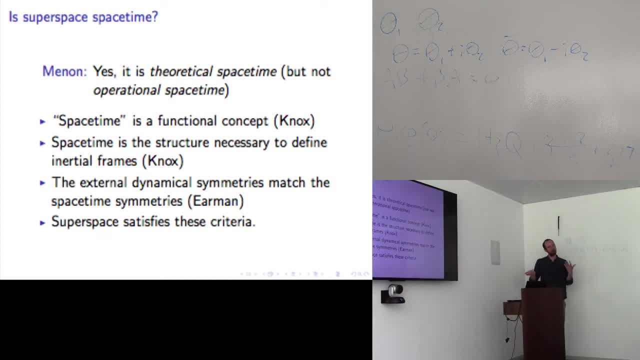 And that's really, ultimately Knox's idea of what is an inertial frame. An inertial frame is a coordinate system that allows us to state the equations of motion as simply as possible, And we do have that notion in superspace, which is the notion of what's sometimes called a super-nitral frame. 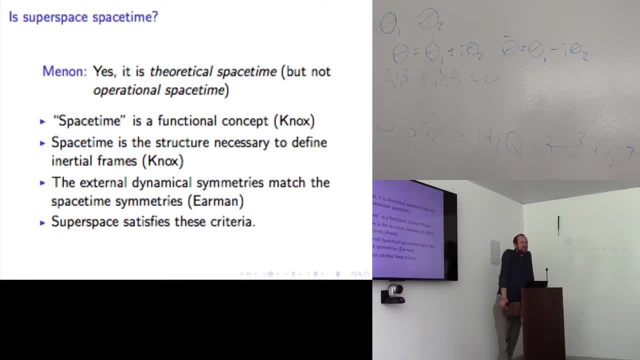 Yeah, Can I give you an example? Sure, So let's say I take instead the electromagnetic field and I have some scalar that defines its value at every point in spacetime and I just tack that on to the vector that tells you that defines your inertial frame at every point in spacetime. 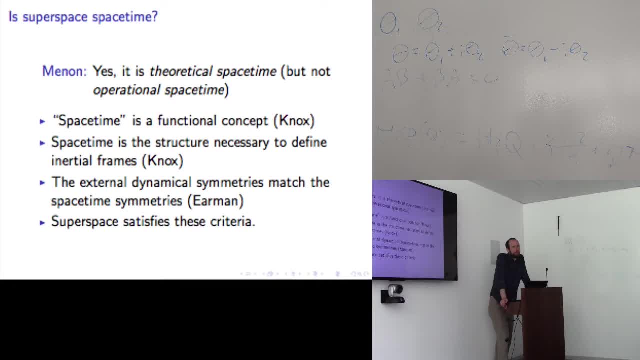 So now I'm constructing some superspace. it's not this superspace that you're talking about, but it gives you more information in a, some would argue, simpler form than you can get by defining the theories separately, And I would say that you could under your definition. 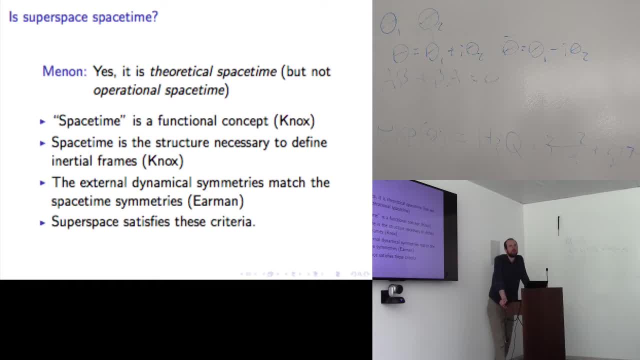 you could say: well, this is the structure necessary to define inertial frames. if you say inertial frames are the way you define them, And I would say that's sort of entrenched- Yeah, it is. I mean, there's something here which I very much agree with. 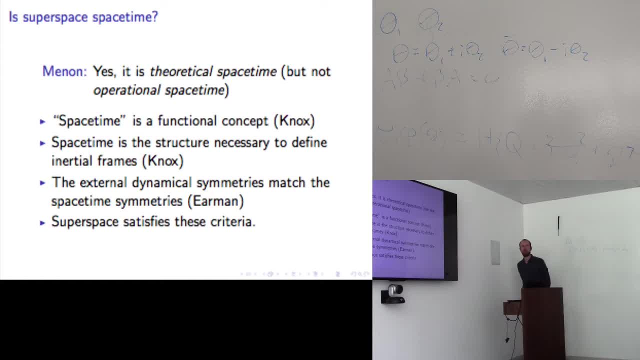 which is that there's a bit of arbitrariness in Knox's privileging of the stuff that she does privilege, You know it's like. so I mean spoiler alert. I don't agree with Knox. I have quite a different view of how to be a spacetime functionalist. 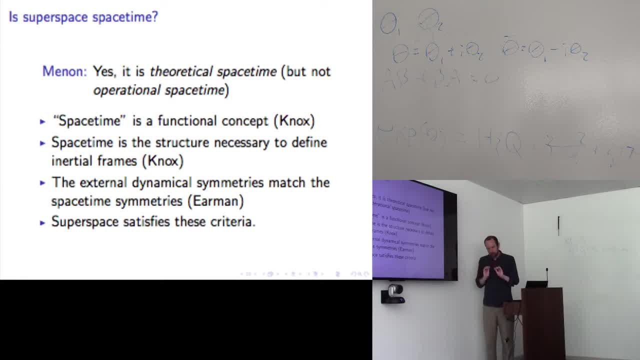 She would say, right, that it's not, that the inertial frames are the frames in which the theory as a whole can be expressed most simply. They're the frames in which the equations of motion, in particular, can be expressed Especially simply, right. 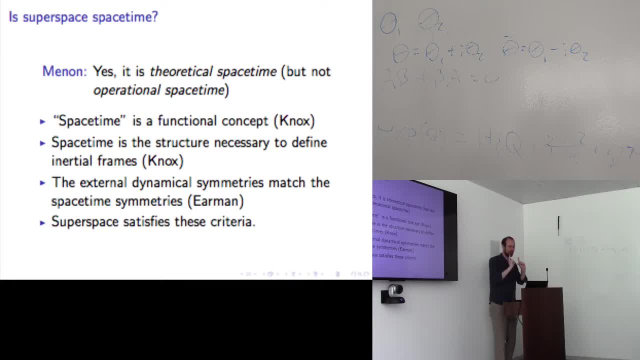 So that's, I think, where she would say: you can't find, you know you can't define. but there's another thing in your question, though, which I think I do really fundamentally agree with completely, which is we could come up with a new definition of inertial frames. 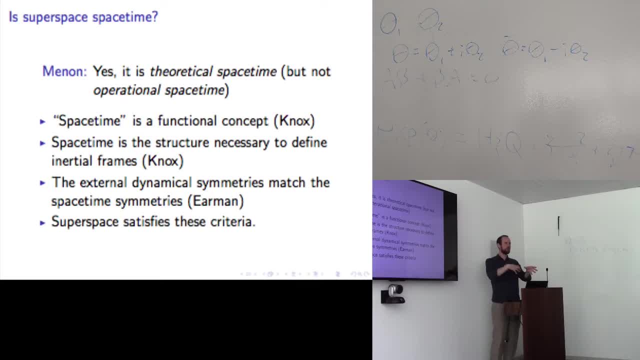 of inertial frames. by changing which kind of coordinate systems we're writing the theory up in right. So, like ordinarily, we write electromagnetism in four-dimensional coordinate systems, you know, for using regular spacetimes. Could you come up with a different version of it? 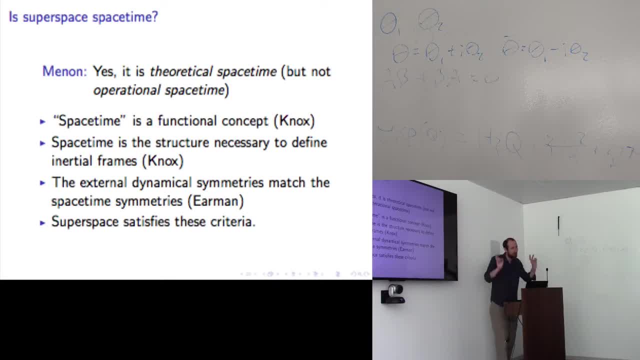 with higher dimensional, like quote-unquote geometries and define your inertial frames differently with those right. I actually think that what this kind of example shows is that Knox's picture doesn't have the resources to like tell the difference between those things. 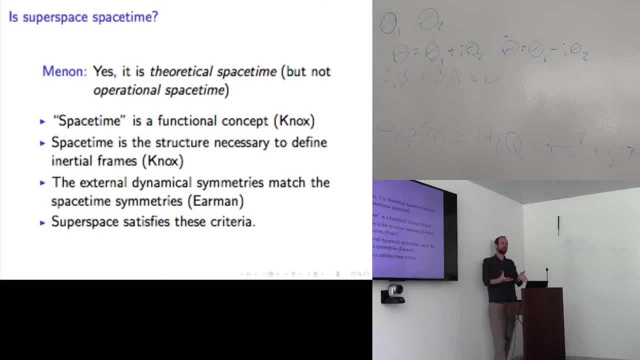 because essentially her criterion for inertial frame is: give me a bunch of different coordinate systems that are all kind of like the same type of coordinate system, right? So they're all tetrad fields of the same dimension, which is to say like they're all coordinate systems. 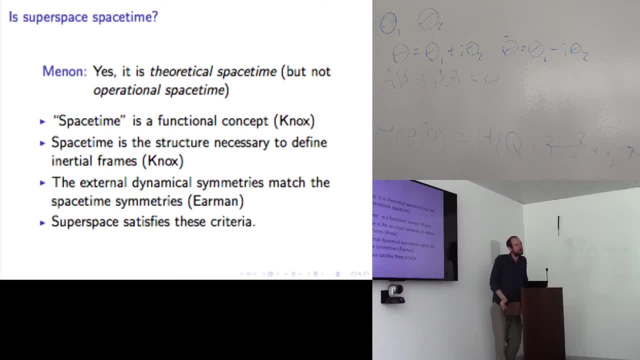 you know, like four-dimensional coordinate systems, something like that, right? So she says: give me a theory and give me some coordinate systems on it- Maybe they're four-dimensional ones, Then I can tell you which of those are the inertial frames. 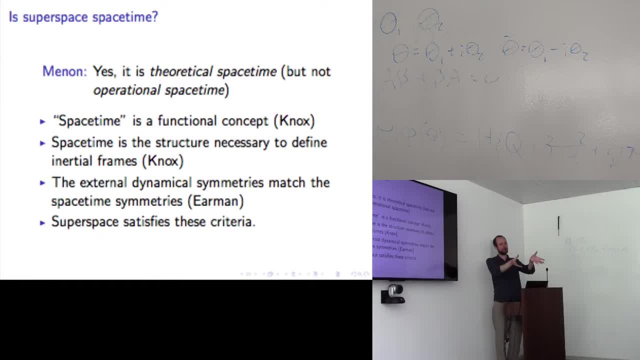 because they're the ones where the equations of motion take on the simplest form. What if you gave her eight-dimensional coordinate systems right? Well, there might or might not be an answer to how you would make the. I don't know what the analogy of equations of motion would be. 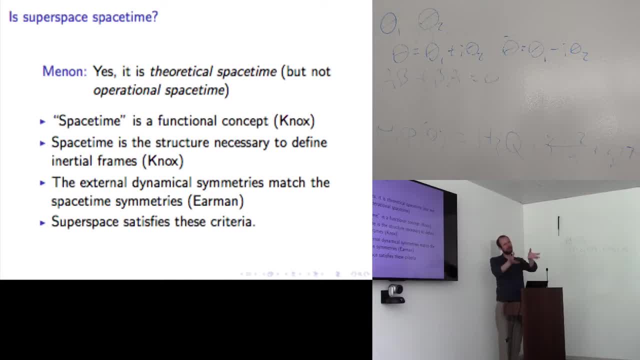 but you might be able to come up with some analogy of them and come up with frames of those sort in which they were as simple as possible, And then you could say to Knox: well, which ones give me the real space-time? Is it the four-dimensional ones that I can give you? 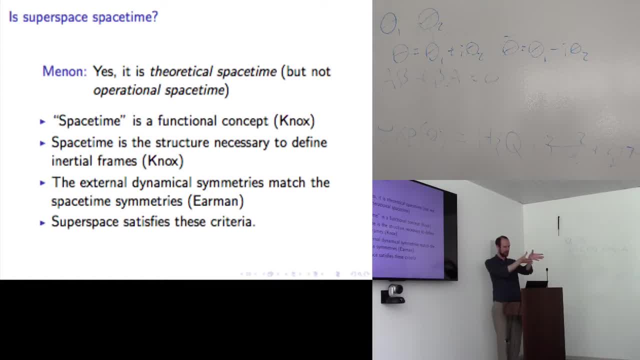 and get the- you know, the inertial frames from those, Or is it the eight-dimensional ones that I can give you and get the inertial frames from those? And she wouldn't be able to answer that question, right, I mean. 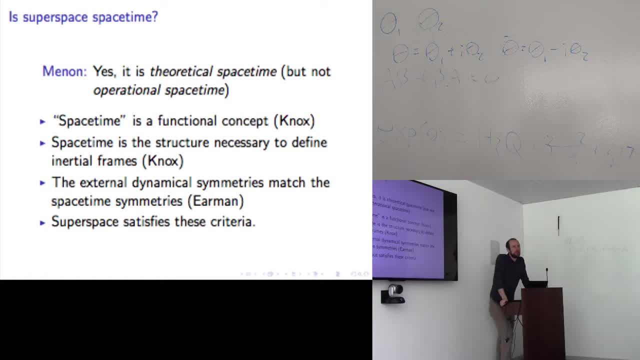 Sorry. Yeah, Like one of the Like. these questions were sort of discussed in the beginning of general relativity. You know they're like because of all this interpretation of, oh, you know, the general relativity field is some geometry. 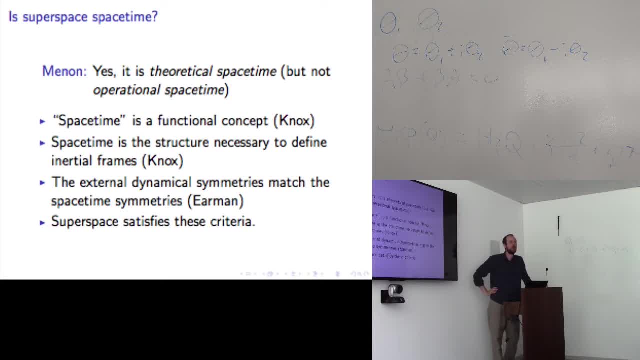 they're like: well, can't we just interpret the other fields as geometry? Yeah, yeah, yeah. And the reason they threw it? They didn't throw it out, but the reason they said no, or the reason you privilege the space-time metric, we know and love. 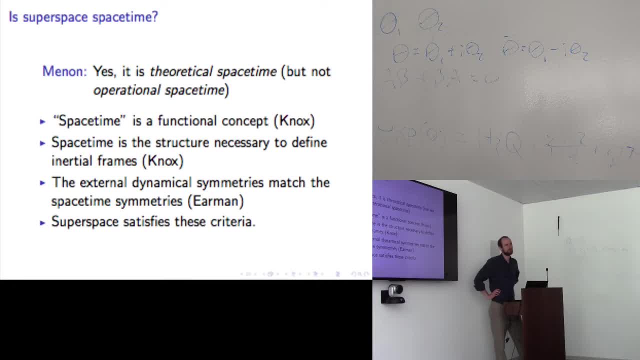 is because of universality. So it seems to me that if you want to use one of these criteria to privilege superspace, the supersymmetric superspace, you also have to privilege all of the other superspaces. you can build with other fields, And then you have to choose your reason. 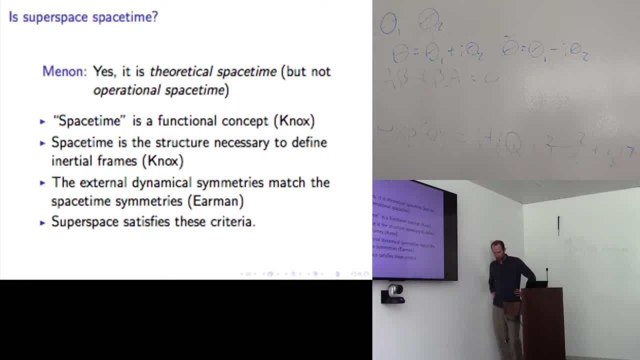 why you think the supersymmetric superspace is important. And if your reason is because supersymmetry does other things for us, that's fine, but you can't say that it's somehow unique. Yeah, Yeah, I mean I As a 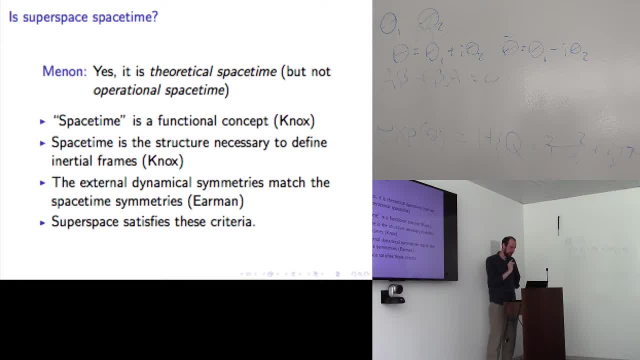 Right As a As an application of Dox's view. I totally agree with you Because I think I think essentially right. Nox's view doesn't give you the resources to say: should I take a supersymmetric theory and input four-dimensional coordinate systems? 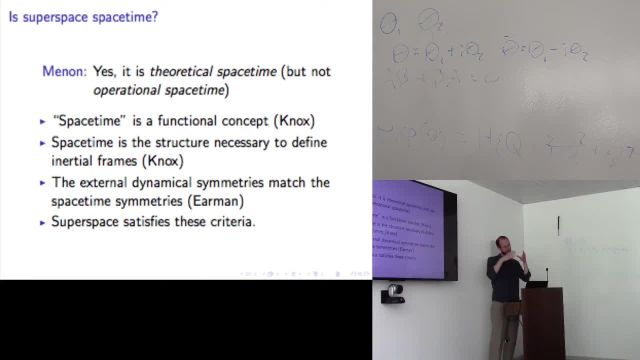 or should I take it and input, you know six-dimensional coordinate systems with the two Grassmann coordinates included right? Her picture just tells you what's an inertial frame, given that you have handed her a set of coordinate systems, Right? 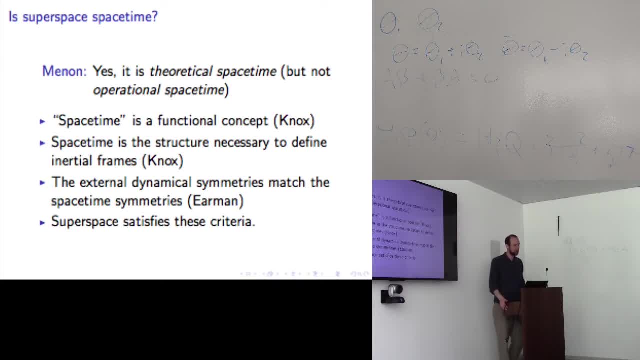 Yeah, So. So This is, Yeah, This is. This is very closely related to one of the criticisms of Nox that I mentioned in the kind of written version of the paper You know it's, I think there's. 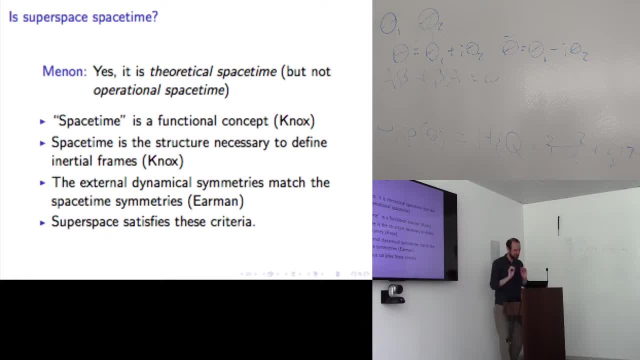 I think there's a serious problem for review here, And you're exactly right, I think, in a way About what it is, Yeah, Okay, Which is really good, because I was kind of hoping that I'd be able to get to that in some form in this talk. 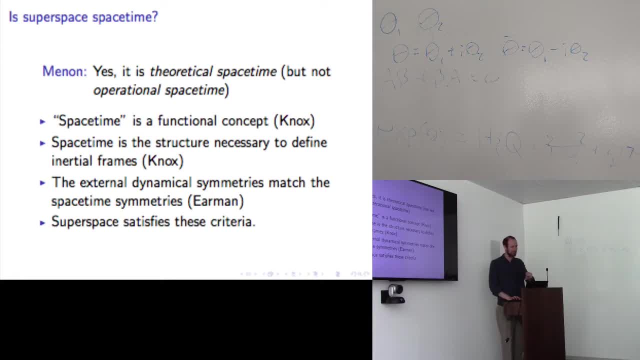 but like I wasn't sure I was going to, Okay, So Here's my reply to what Tushar has to say. Right, And this is closely related to my reply to Nox's view as a whole. So my 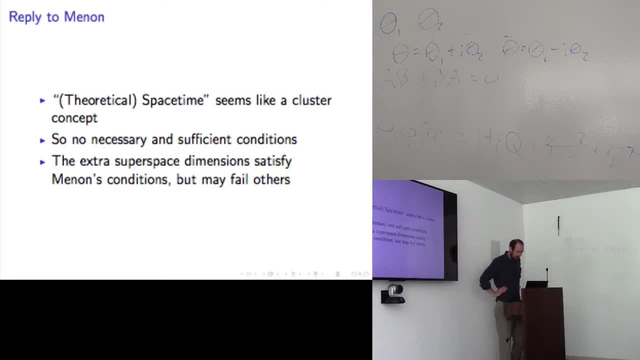 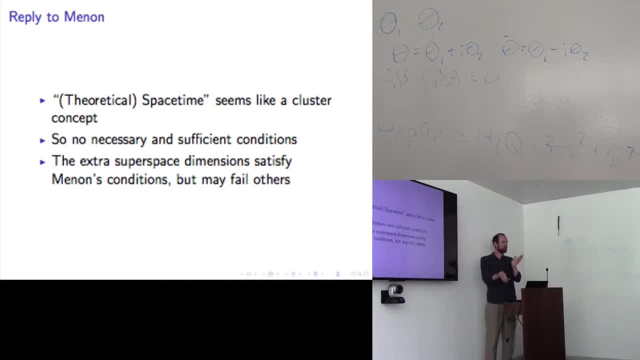 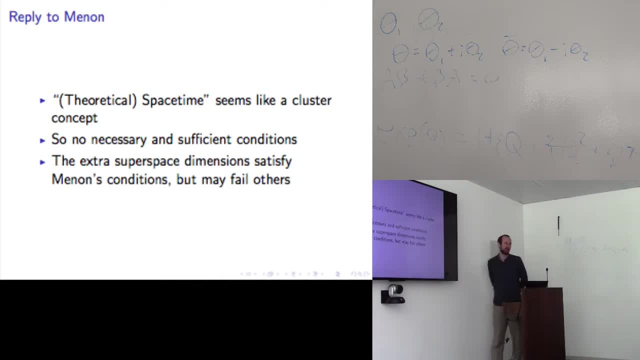 You don't have to talk about its genetic code or evolutionary characters. Think about unicorns, right, Well, to be a unicorn, it helps to have four legs, but surely, uh, that's such a sad, this is such a sad thing to think about a unicorn with a missing leg. 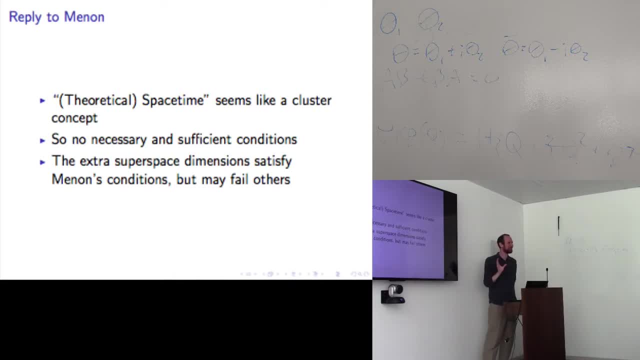 It's really funny. I just revisited The Last Unicorn. Anybody ever watch that movie? It's a classic, animated, beautiful movie. Um, so the thought of a unicorn missing a leg makes me really sad, A unicorn voiced by Theo Farah. 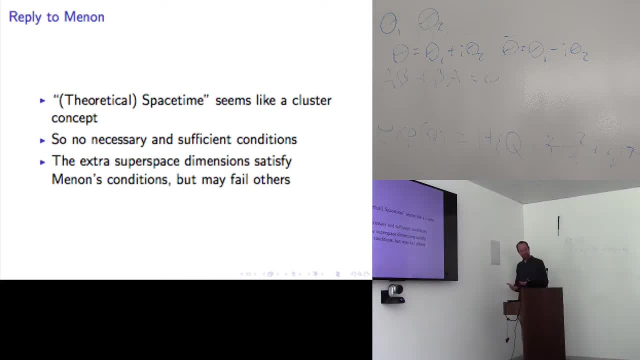 So, uh so, but if I imagine a unicorn with a missing leg, um, it could still be a unicorn, right? It's just that you know, having four legs helps you count as a unicorn, right, It gives you a unicorn. 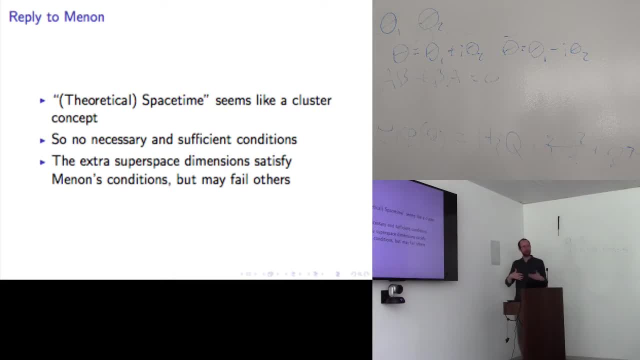 Having a horn. you know, if you had your horn cut off, you might still be a unicorn, God. this is, if you had your horn cut off, you might still be a unicorn. Um, uh, but um, but right, um. it helps of course a lot to count as a unicorn if you have a horn, an intact horn. 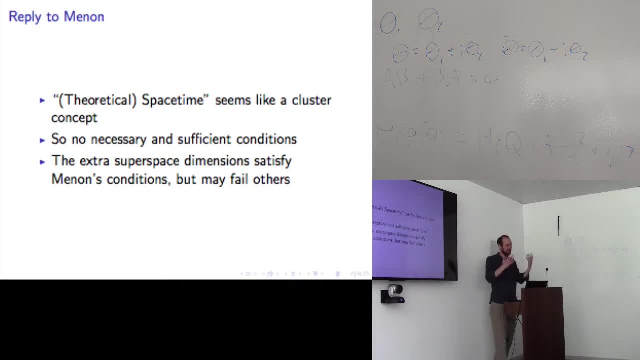 Um so unicorn seems like a cluster concept. right, It's one of these things, you know, of course. Wittgenstein famously talks about the example of a game. Uh, Bereskov talks about the example of art as a cluster concept. 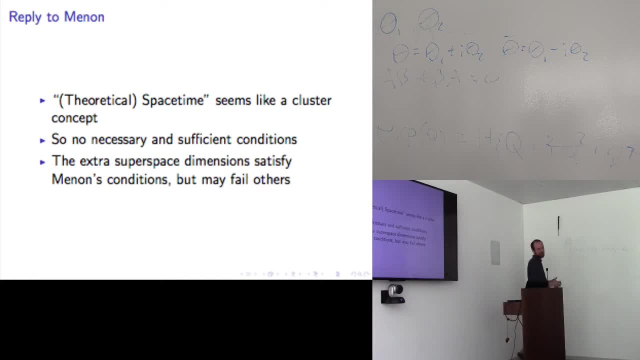 Um, the idea being there's no single necessary and sufficient conditions for it. Instead, um, there's a bunch of different factors And if you meet enough of the factors, to enough of a degree, you count as art or as a game or as space-time right. 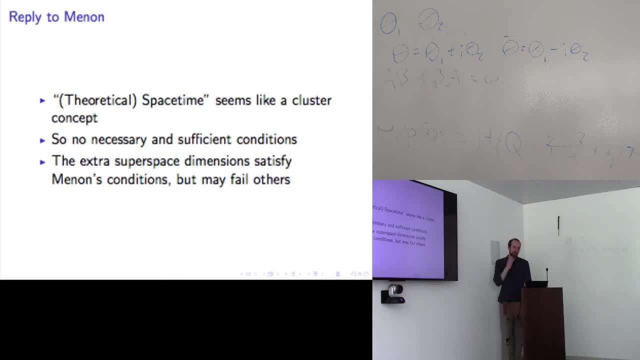 Um, that's how I like to think of space-time. There's no necessary and sufficient conditions for being space-time, There's just a bunch of different criteria, And if you meet enough of the criteria to a high enough degree in a given theory, then you know. in other words, let's talk precisely here. 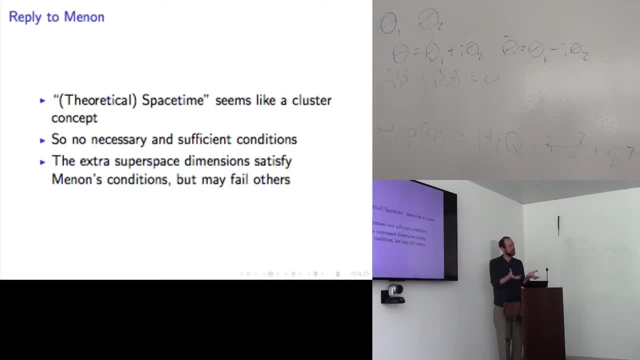 If I have a, a type of structure in a given theory and I think, how well does it meet different criteria within that theory? Like one of the criteria I I agree with Knox is uh, explaining the inertial structure of the theory. 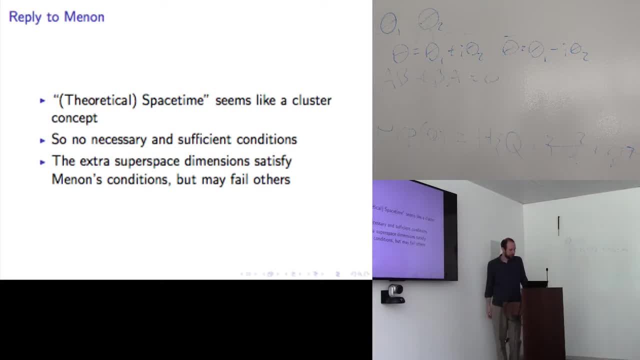 Right that that's a big job, Um, but there's other ones, you know, Um uh, operational criteria, like the ones that you know Tushar mentions, are important ones. Do rods and clocks measure this quantity? 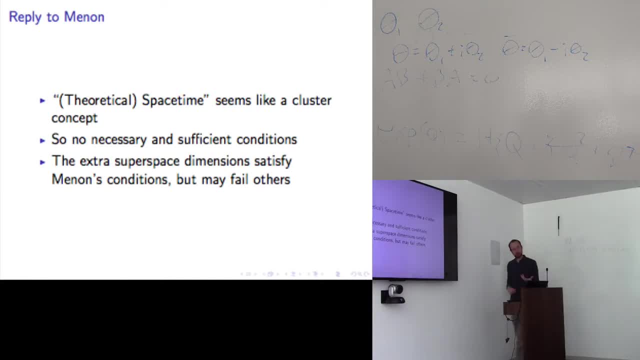 Right, And the case of super space actually shows that it's possible to have to meet those inertial criteria without meeting those, um, operational criteria, Right, Um, you know, there's other things you can think of, like, uh, giving us the distances along which forces fall off, and stuff like that. 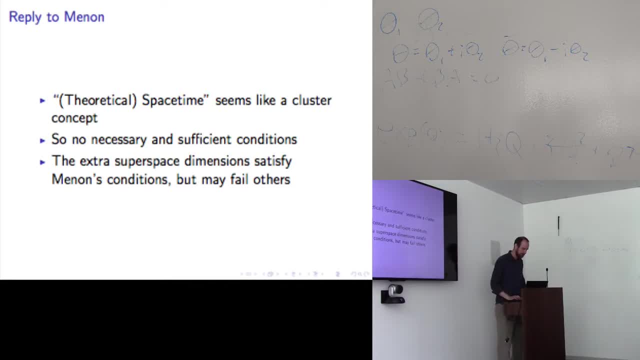 Right, Um. so the extra super space dimension, The extra super space dimensions. well, they satisfy Tushar's conditions for theoretical space time and they fail others, And indeed, as he notes, they fail the criteria for operational space time. 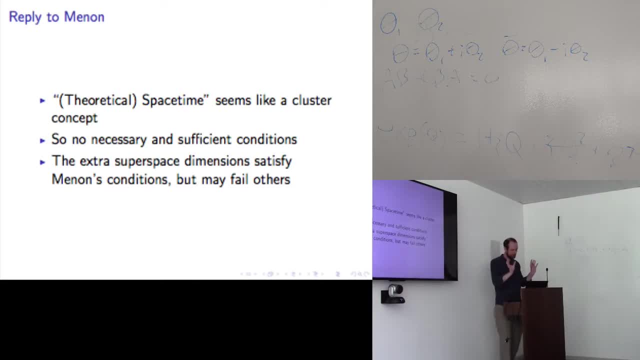 Um, I mean, in a way, this is a place where we're sort of separating our questions because, um, I would tend to say, uh, I'm not sure I have exactly a separate concept of theoretical space time. Instead, I might say I kind of unified concept of space time, and the theoretical and operational parts of it both count towards that question. 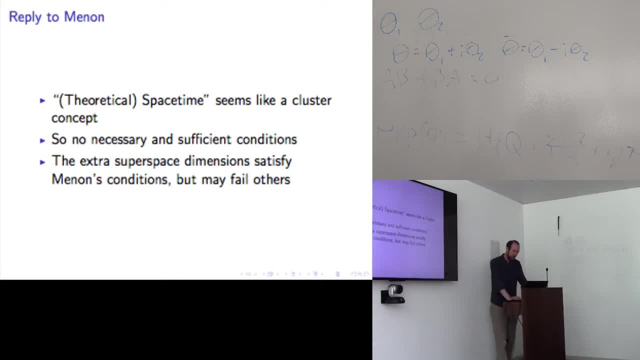 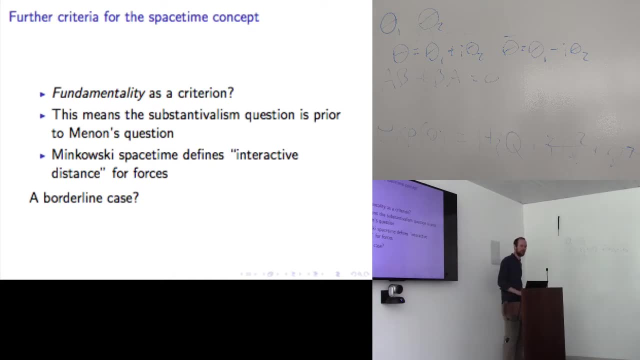 Um, but additionally right the, yeah, the extra super space uh dimensions might fail other conditions besides the one for Tushar's conditions. Now I want to talk about some further criteria that I think are plausible, In particular the Fundamentality criteria. 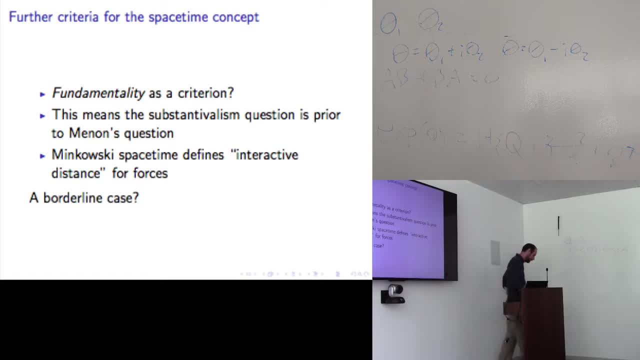 Right? Um, so it seems to me that pretty much everybody you know, substantivalist in relation to this right, disagree on a lot. One thing they agree about about space time is that in some sense, the facts about space time are highly fundamental facts. 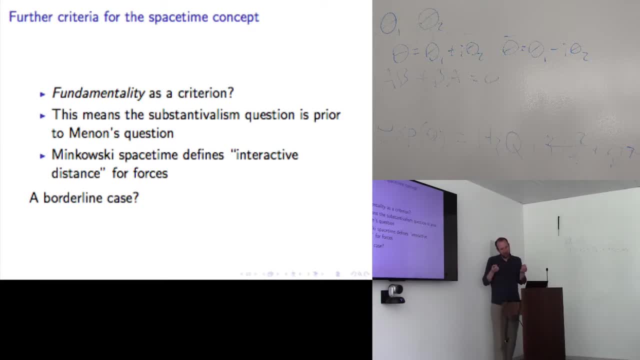 Right, For the relationist, they're highly fundamental, uh, not facts about ontology, but facts about what relations it holds between the things that exist, Um, whereas for the substantivalist, they're fundamental facts about what exists, This, this substance, space, time exists. 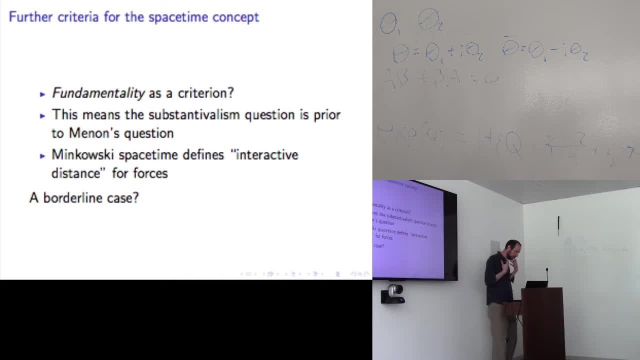 Um, So everybody agrees that space time is highly fundamental And it's probably not perfectly fundamental. you know, uh, unless you know Tim Modlin's pessimism about essentially all programs in quantum gravity research that are going on now. 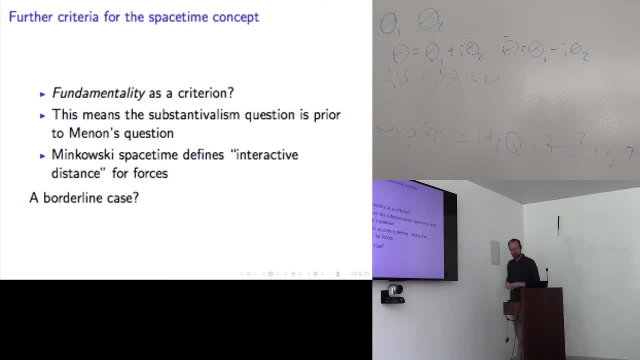 Unless that pessimism is justified, Um, or you know, unless, unless one of these sort of um, I- I should put that in a different way- Which is, unless one of these Bohmian research programs is trying to recover fundamental facts. 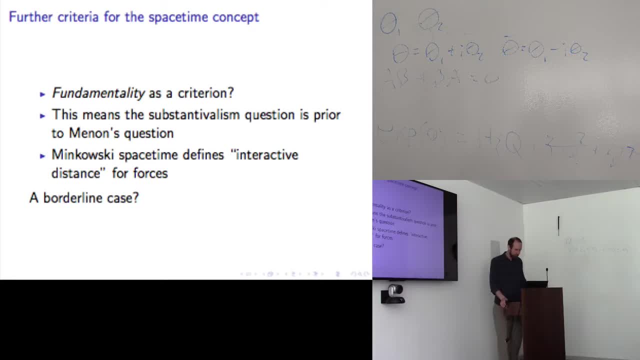 Um from quantum gravity succeeds, It looks like we might give up on space time as a fundamental notion. Just that's the direction that most research programs in quantum gravity are going, But still it's going to be a highly fundamental um. space time is going to be a highly fundamental structure. 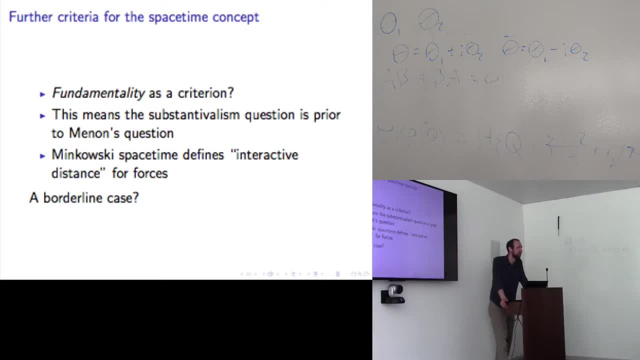 It's about as fundamental as anything that we have a good theory of right now, Which makes it highly fundamental. So I'm thinking, you know if I, if I, You know if I, if I look within my own, You know this gets to the point where questions about concepts can be kind of semantic questions in a way. 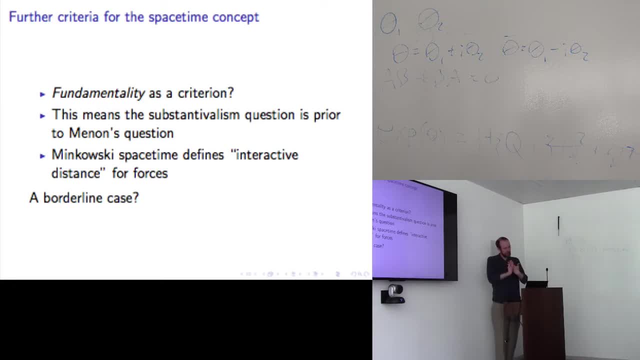 But if I look within my own heart at the question of um, what counts as space time, I think well, if it's highly fundamental, that makes it more apt to count as space time. Another type of example that's helpful to think about this is: you think about a structure that's isomorphic to space time? 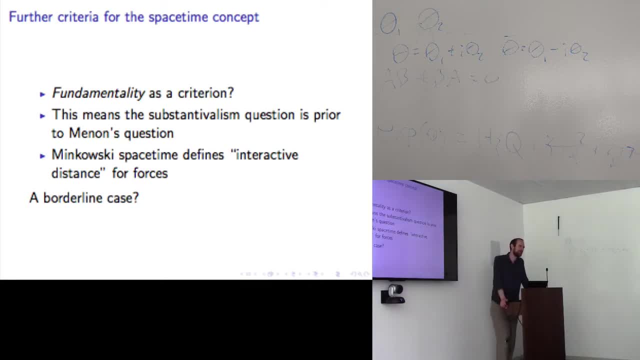 In some kind of computer simulation or something, right? Is the space time that they seem to live in Inside in the matrix um a space time, You know? is that really space time, right? Well, I would say no. 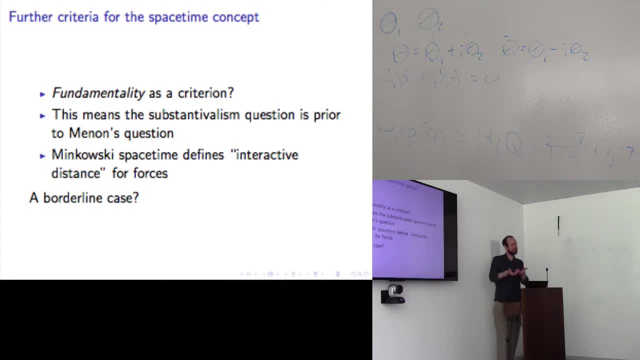 Why not? I mean it's, it has all of these functional geometric characteristics that we associate with ordinary space time, But it's not. it's not very physically fundamental, you know It's. it's made up out of- uh, you know, electronic goings on. 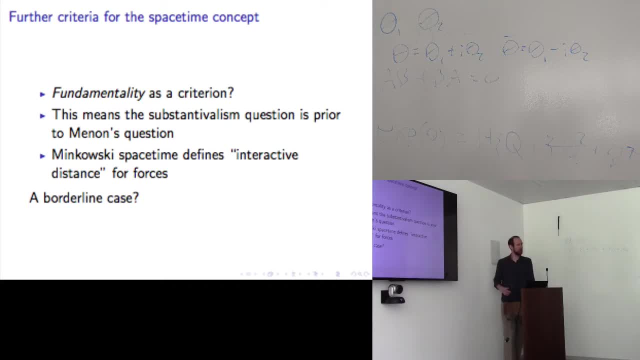 So that's why I don't think the space time of the matrix is fundamental. It is a space time, Um, if I'm correct about that, Maybe I'm not. That's an interesting debate to have. But I it seems to me that fundamentality ought to be one of the criteria for the space time concept. 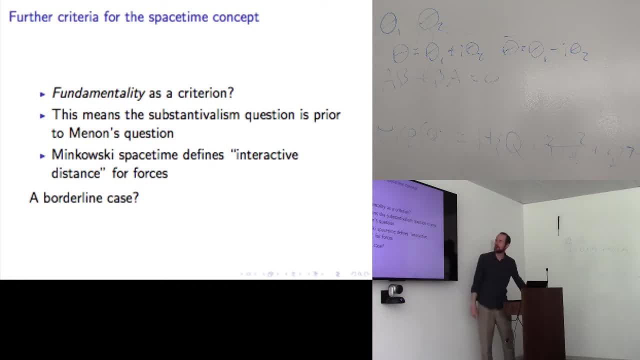 If it is a criteria, then that means we have to answer the substantivalism question prior to answering uh Tushar's question about whether super space is space time, Because I take the question of substantivalism to be the question of whether you know. 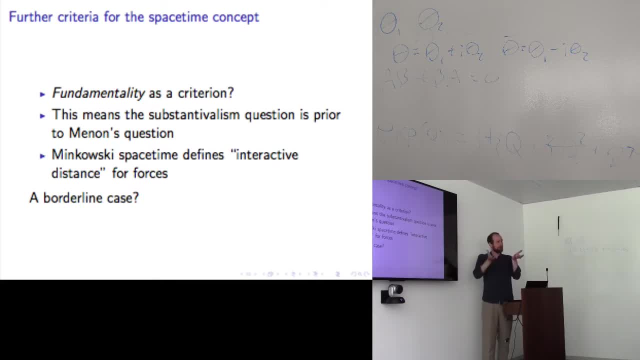 you know well, the question of space time substantivalism is the question of whether space time is a fundamental substance, Right? So the question of substantivalism about super space is the question of whether super space is a fundamental substance. And it might be a fundamental substance and not count as space time. 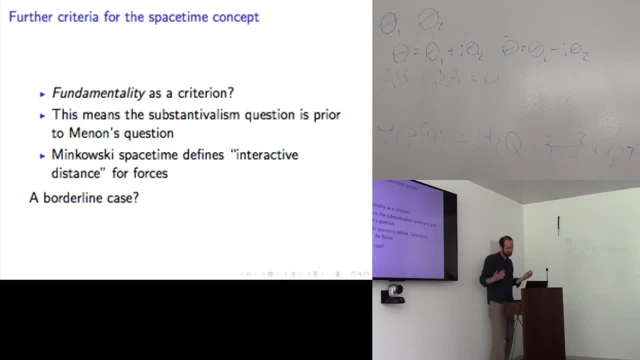 Right, You know, like um, like an electron is a fundamental substance and it's not space time Um. So Well, electron's probably not fundamental whatever Um In, you know, relatively fundamental Um. So 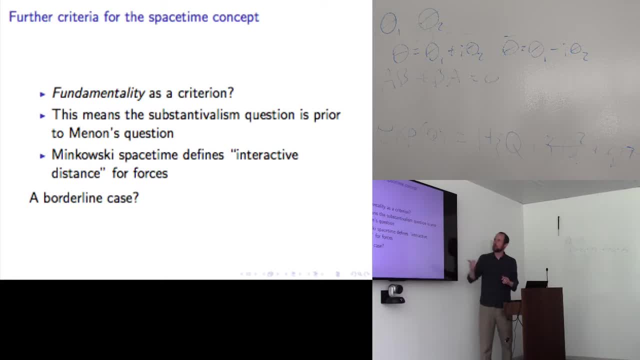 I think this might be a borderline case, Right, And as I mentioned before, you know, Minkowski, space time defines the interactive distances for forces And it has all those operational characteristics. So this might be a case where, ah, you know, it's, it's not exactly settled whether our concept 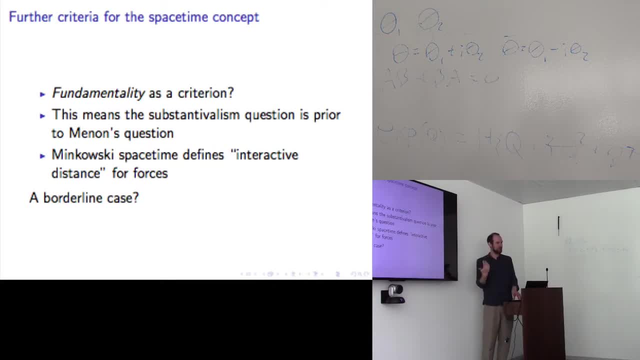 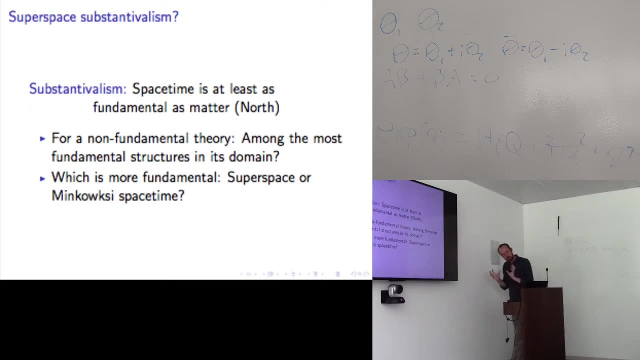 Our existing concepts are going to count super space as space time or not. But I want to just talk briefly about the substantivalism question, Because I think that's actually the most me question philosophically. It's a it's a real metaphysics question. 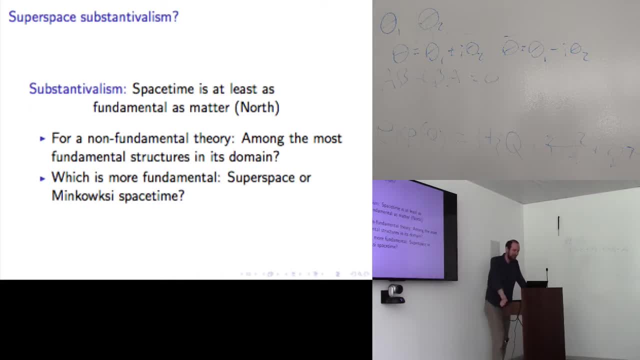 Right, Which you know some people don't like that, But I do like it. Um. So here's my definition, which is Jill North's definition, really, Um, Of what it is to be a substantivalist about space time. 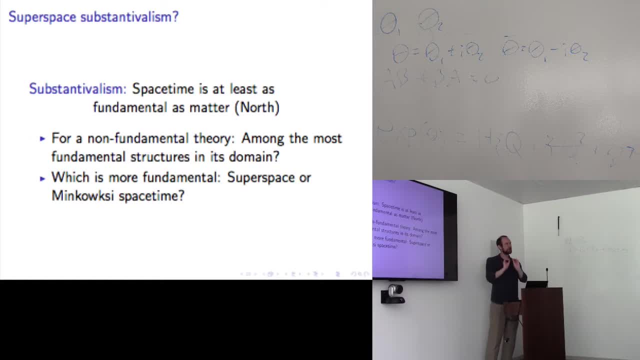 Right, You can be a substantivalist if you think space time is at least as fundamental as matter. Um, That is to say, if I tell you all the fundamental facts about matter, I've still left out the fundamental facts about space time. 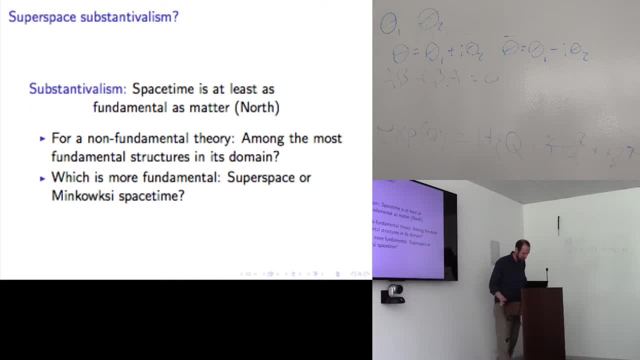 Um, That's substantivalism. Now For a non-fundamental theory. You know, If I say that general relativity is not a fundamental theory, But I am a substantivalist about general relativity. What gives Right? 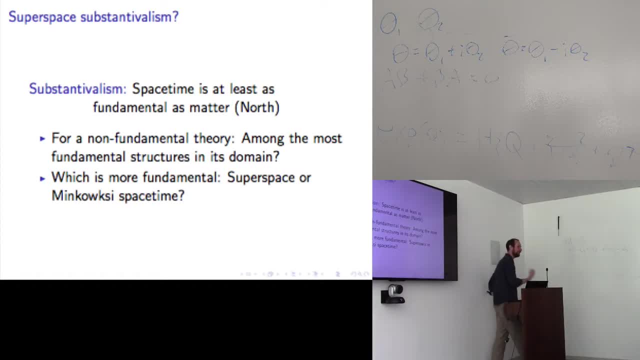 How can I, how can I, adopt this attitude towards a theory that I think is not a fundamental theory? Well, In the case of general relativity, what I want to say is that space time is among the most fundamental structures in the domain of application of general relativity. 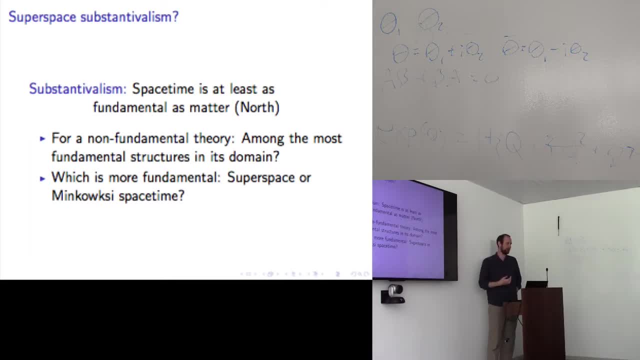 Right, It's one of the most fundamental structures we try to describe using general relativity. We don't try to describe, you know, spin networks using general relativity or something. So, even though spin networks might be more fundamental than space time, 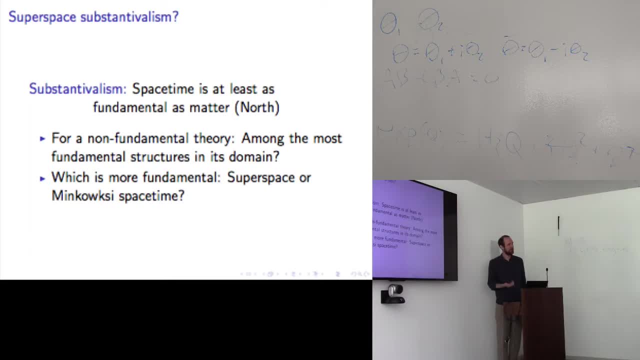 Um, I'm still a substantivalist about general relativity because I believe that space time is one of the most fundamental structures in general relativity. So this is a sense in which you can be a substantivalist about a non-fundamental theory. 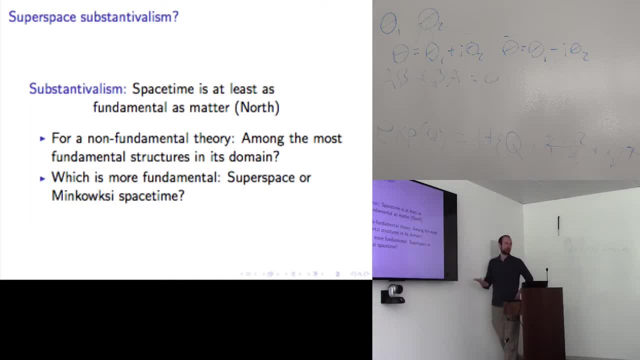 So now Right, Supersymmetric quantum field theory is also not a fundamental theory, But I can ask the question similarly whether you should be a substantivalist about superspace in supersymmetric quantum field theory And I. in that case, I take that question to mean the question of which is more fundamental: superspace or Minkowski space time. 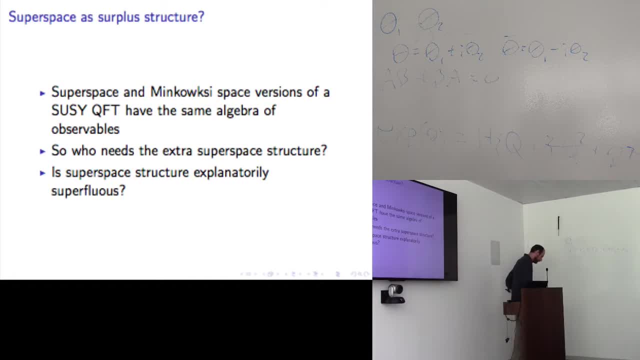 So here's one argument in favor of being a substantivalist about Minkowski: space time And not superspace, The idea that superspace might be a sort of surplus structure. Right, It's extra, We don't need it in order to do the work. 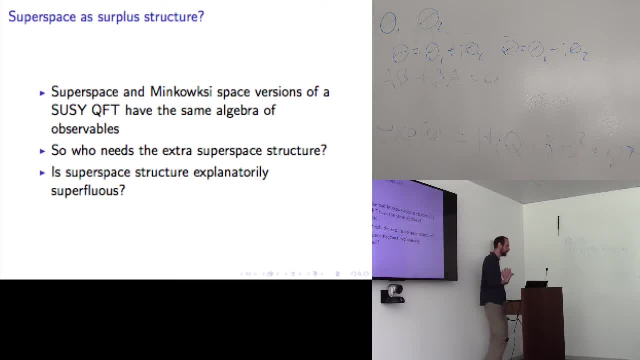 We can write up our supersymmetric quantum field theories in Minkowski space. Why should we add this extra structure? It might be calculational useful, But why should we posit it as part of our ontology? Um, And there's a sense in which it is surplus structure. 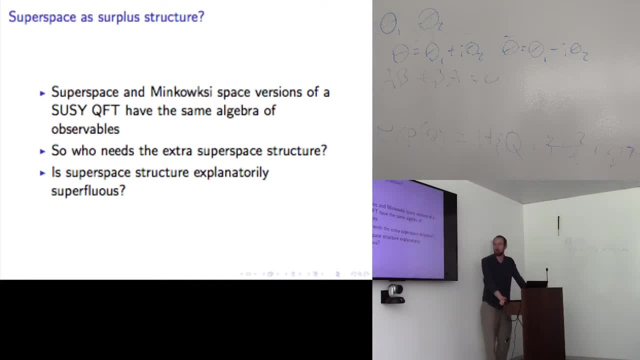 Right, Because there's kind of, if you look at the paper about this that I sent out, I talk a bit about this And there's some stuff that I cite which is incredibly. you know it's algebraic quantum field theory. you know from mathematical physics journals. 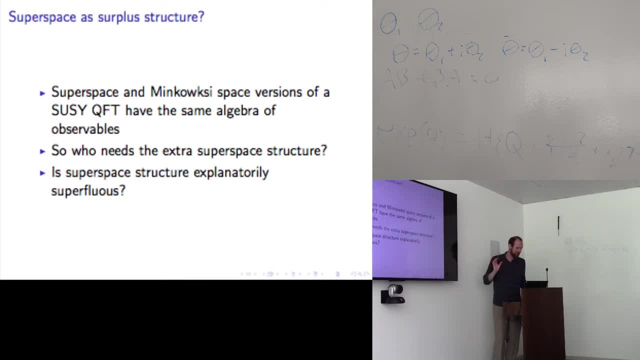 It's incredibly, incredibly difficult to read kind of stuff, But I have corresponded with one of the authors of it, So I understand it conceptually, which is all that I need for my purposes. So what these guys show- or it's actually a conjecture, but they show it in the case of this oscillator model and they're pretty certain that it holds in general. 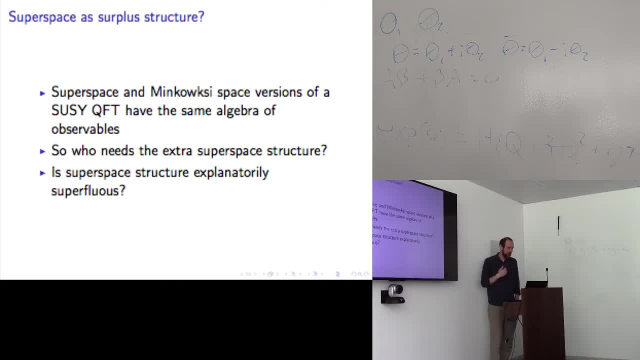 Is that you know, and it has to be true in general. Right, It would be crazy if it wasn't true. Superspace and Minkowski space versions of a given supersymmetric quantum field theory have the same algebra of observables. 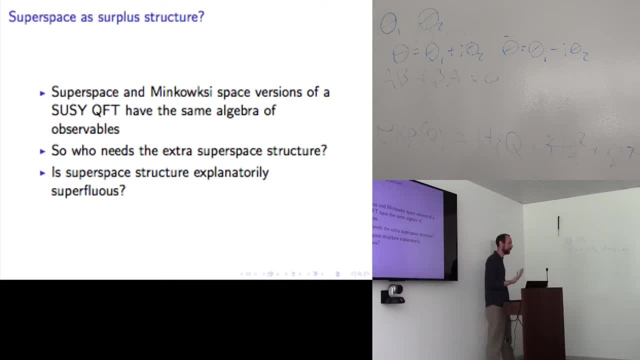 Right, That is to say that they're characterized by the same, By the same physical kind of measurable quantities within the ordinary quantum formalism. Right Again, if you want to be, if you want to have a hidden variable theory, you'll object here and say: well, the observables aren't all the real physical quantities. 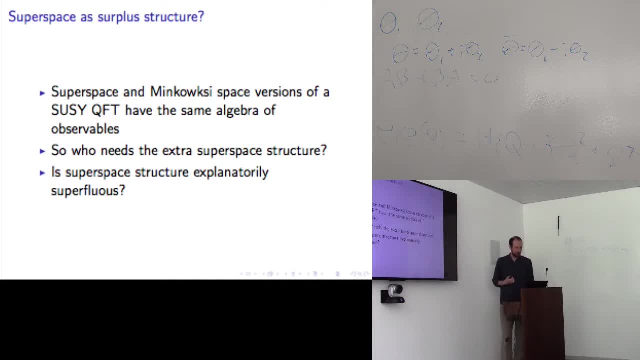 But within canonical quantum formalism, superspace and Minkowski space versions of the supersymmetric quantum field theory have the same measurable quantities, So like. why would we need the extra superspace structure when we can define all of the measurable quantities we need on the Minkowski spacetime? 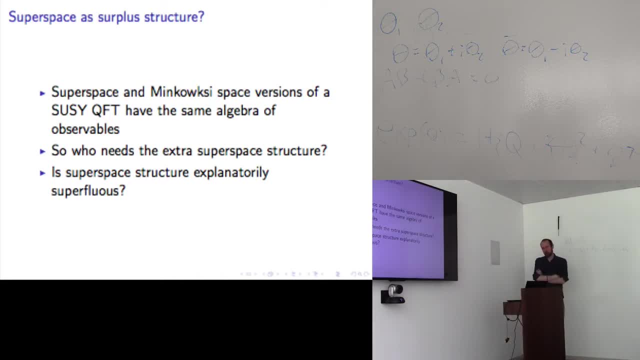 Right. We have a rigorous equivalence between the two algebra's observables. So in other words, if I take a given supersymmetric theory and I write it up on Minkowski space, And then I take the same theory and I write it up on superspace, 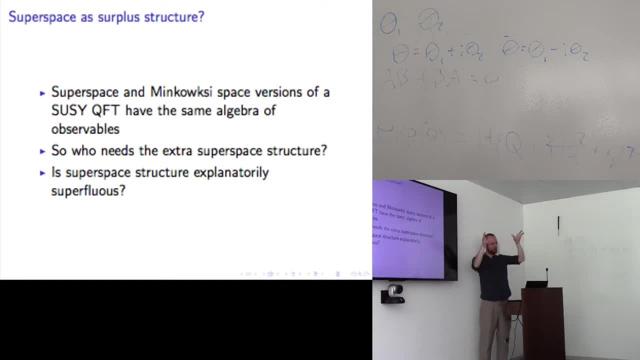 What these mathematicians think is that, yeah, there's a rigorous equivalence between the algebra observables on this Minkowski space theory, which we call the component theory, And the algebra observables on the superspace theory, which we call the super field theory. 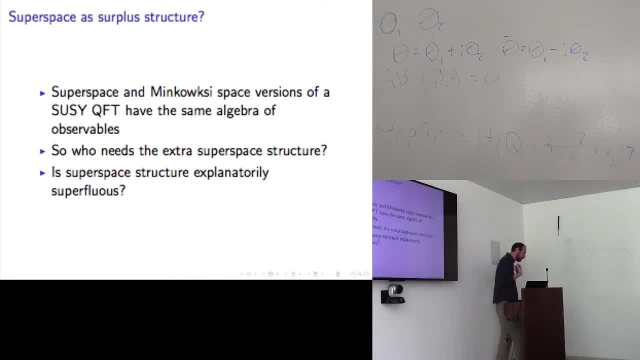 Right, And we don't usually think of operators other than observables as having physical significance. Field operators themselves. Well, they're not invariant under the symmetries, Right, So we usually think of them as physically uninteresting or physically unreal. 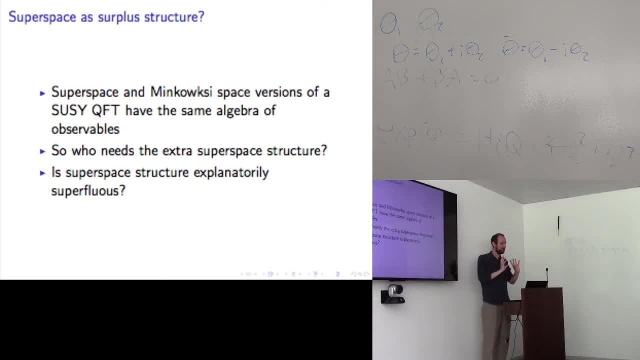 In other words the invariant. a way to put this is that the invariant structure, the invariant observable structure of the component theory and the super field theory are the same. The difference is one of them is on Minkowski space and the other one is on superspace. 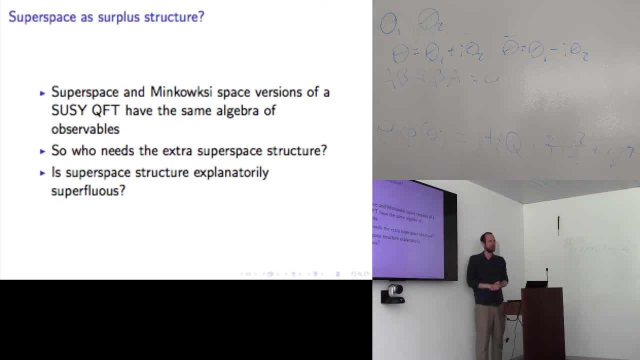 Right. So why do we have to add this extra superspace structure, these extra, you know, grasping value dimensions? Perhaps the superspace structure is explanatorily needless? Well, it is, and it isn't Right. If I just look at a theory by itself and say: what role is the superspace structure playing in explaining the phenomena within that theory, this equivalence in a sense kind of shows us that it's not playing any predictive role. 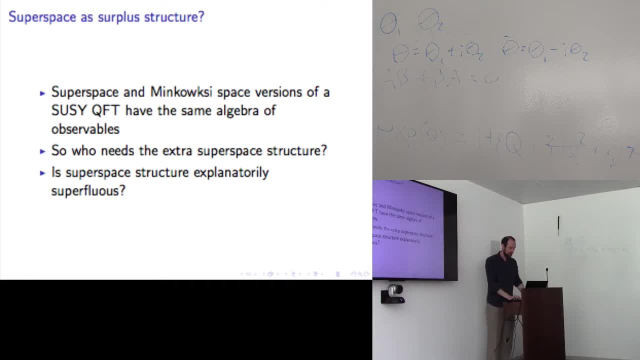 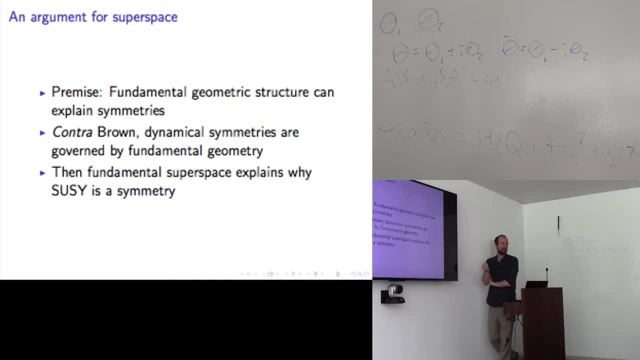 Any role that explains in that way. But it might explain something else which is important, Right, It might explain the fact that supersymmetry is a symmetry. Okay, So here is an argument for superspace substantivalism. This argument was suggested to me by James Wells, who's one of our theoretical high energy physicists at Michigan. 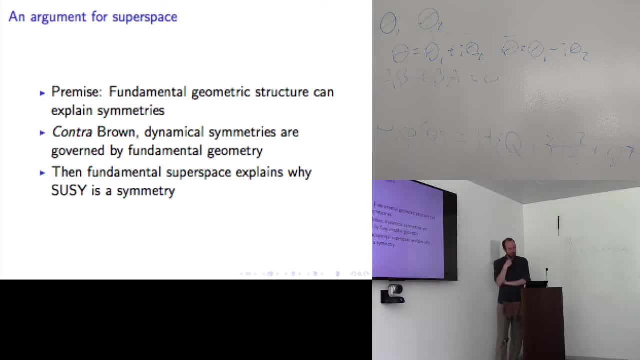 And I went to James and I asked him: James, Do you think which do you think is more fundamental- Superspace or Minkowski space in supersymmetric field theories? And he's like, oh, superspace. I said, why, James? 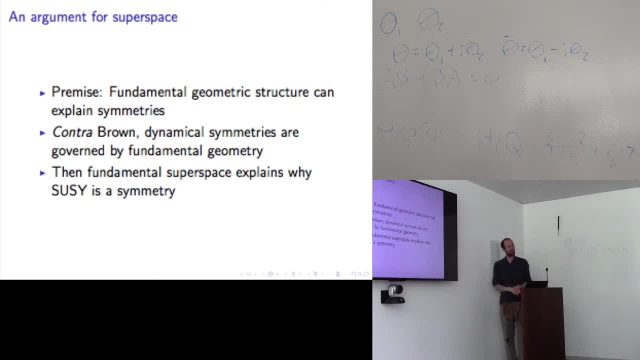 And he said: because if superspace is fundamental, then you have an explanation for why SUSY is a symmetry. Because, the way he put it is, there's no way to write up a theory that isn't invariant under supersymmetry in superspace. 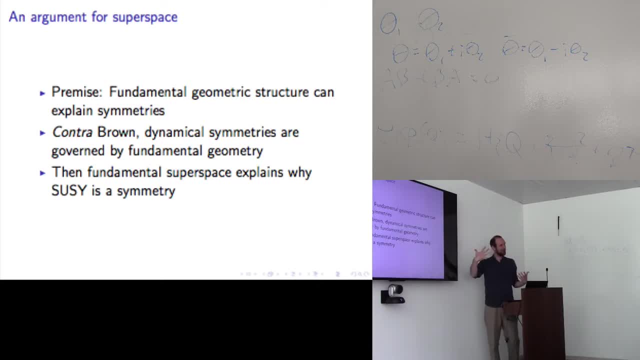 Whereas there is an easy way to write up a theory that's not invariant under supersymmetry in Minkowski space. So we have a sort of explanation for why SUSY is a symmetry. This in order to turn this into an argument. I have to add a premise, which is that fundamental geometric structure can explain symmetries. 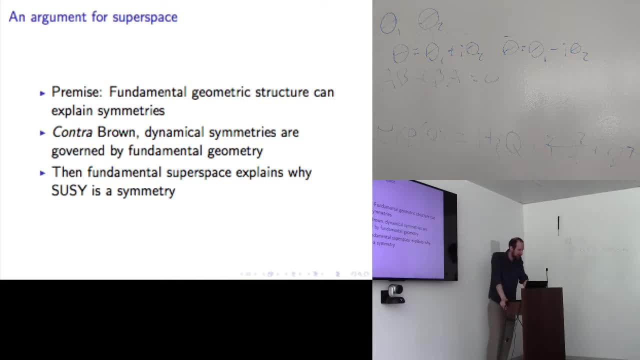 Right And I grew up thinking that this was an uncontroversial premise, And in a move that has been really useful, Even though I think it's ultimately misguided. In a move that has been really useful to the philosophy community in understanding the logical relationships between things. 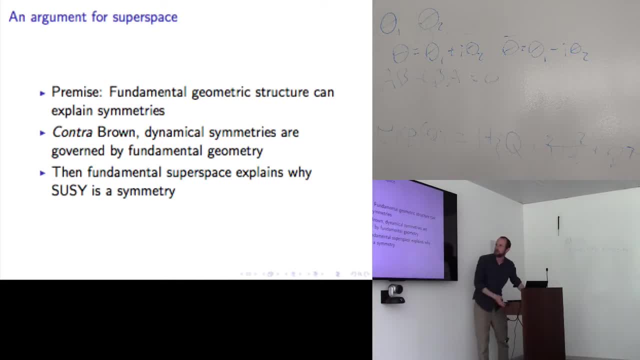 Harvey Brown has challenged this premise by suggesting that, no, you know, dynamical symmetries are not really governed by fundamental geometry. There's no sense in which spacetime forces the theories from the spacetime to have the same symmetries as the spacetime. 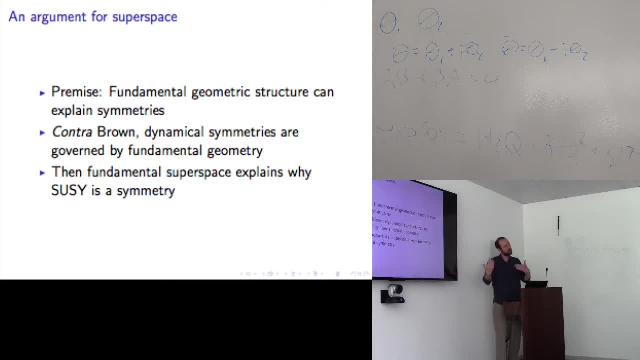 Right. Instead, Brown thinks like: well, you know, the explanation goes the other way. You look at what are the laws, you know what are the dynamics in a world. You think: what symmetries do they all have in common? 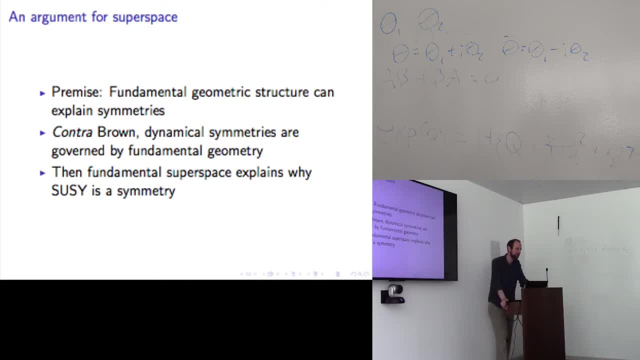 Oh, those have got to be like. you know, it's simplified, But those are the symmetries of spacetime, Right? So I'm? I am taking on board what I take to be a more, a more assertive. 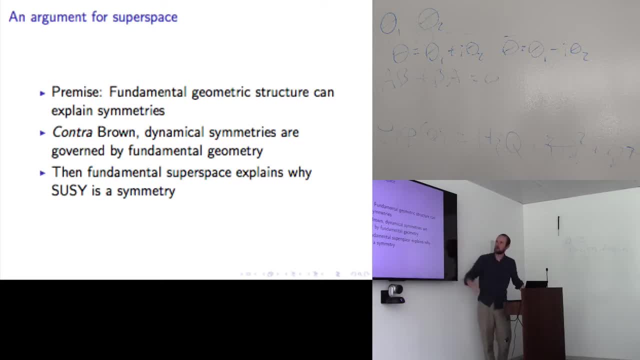 More sort of classic in defense of dogma kind of view against Brown. The fundamental geometric structure can explain symmetries. But if, if I tell you, the spacetime we live in is Minkowski space, for example, That that can provide a good explanation for why the right theory is Lorentz invariant. 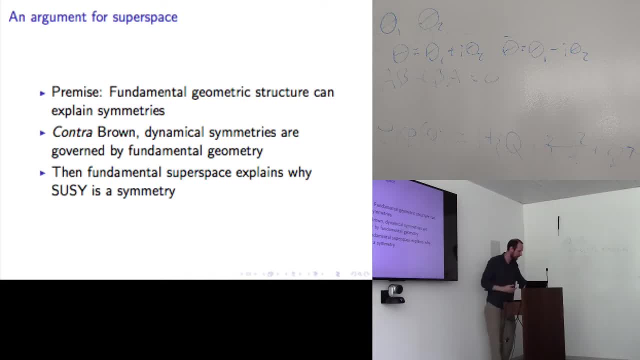 Right, And we can talk. you know, we'll talk in the- I'm sure we'll talk in the spacetime functionalism discussion about whether this is a great assumption to make, But I think it is a good assumption to make. Then, right, if superspace is fundamental, we can explain why supersymmetry is a symmetry. 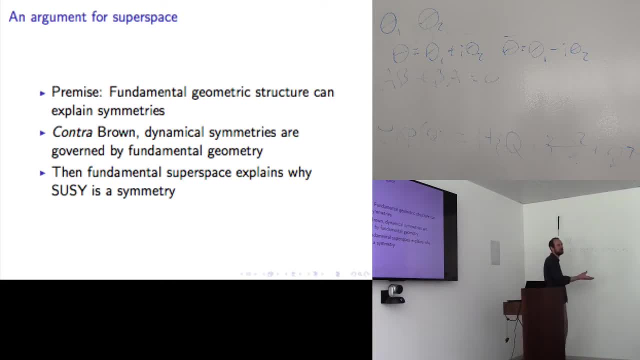 Because superspace is fundamental. It's the fundamental geometry of our world. I'm not going to call it spacetime now, because it's a separate question whether it's spacetime, But suppose it's the fundamental geometry of our world. The symmetries of nature have to match the symmetries of the fundamental geometry of our world. 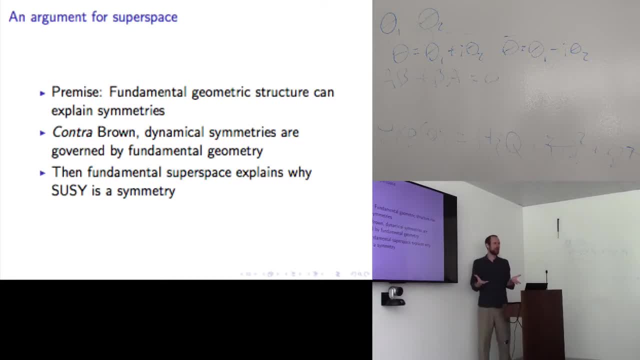 So you know. So if superspace is the fundamental geometry, then we have an explanation for why, in our oscillator example, the mass of the boson and the mass of the fermion are the same. On the other hand, if we, if we didn't live in superspace, if we lived in ordinary spacetime, we we could ask this kind of fine-tuning question. 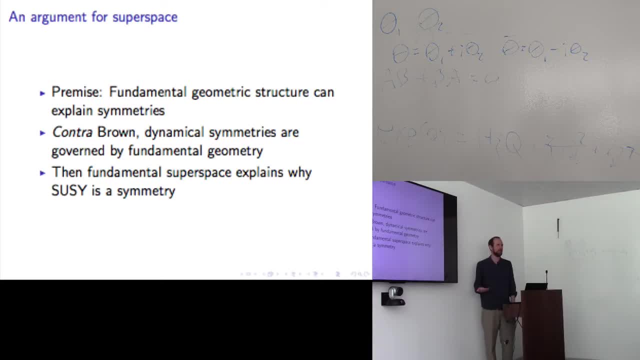 Since why is the mass of the boson the same as the mass of the fermion? And there would be no answer, Right, It would be a brute fact. You want to reduce the number of brute facts. You want to explain them. 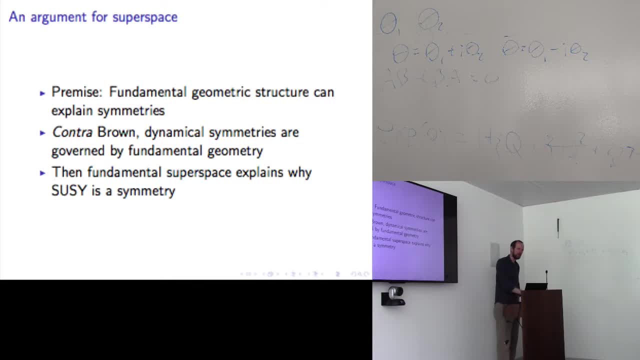 Superspace provides a way to do that. So this, I think you know there's a bunch more arguments you could potentially raise for and against superspace as a fundamental substance, But this, I think, is a pretty good one. 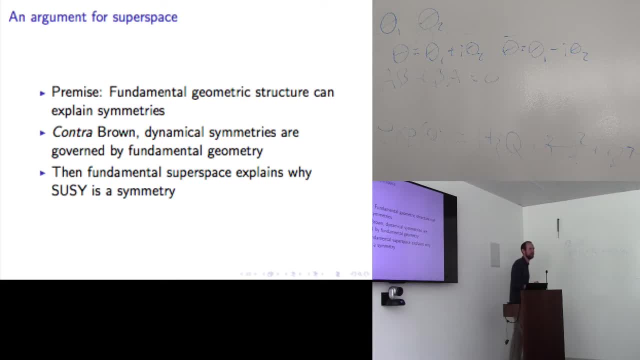 So I think this is a good place to leave it and kind of open things up for discussion. I don't know how you guys want to answer that. Can we take questions? Yeah, Totally, Totally. Thanks for the talk. I was wondering what the thing about the algebra of being the same. 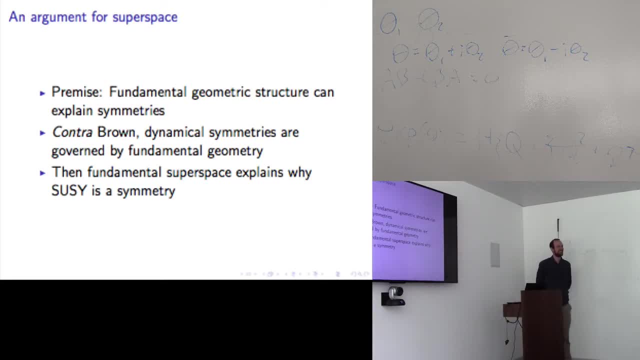 Yeah. Yeah, I was a bit puzzled because of course you have all these structure, you have superspace that you don't have in the cosmic spacetime And I was wondering if you could construct some artificial kind of look at if you have. 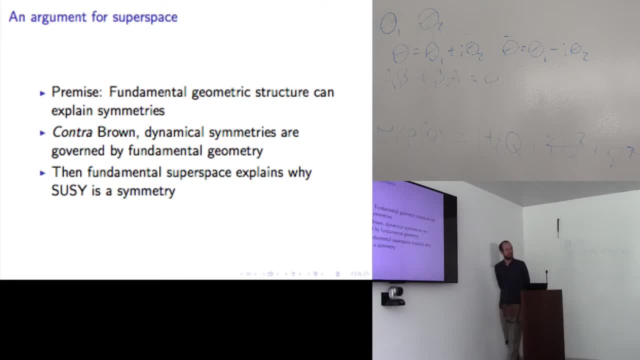 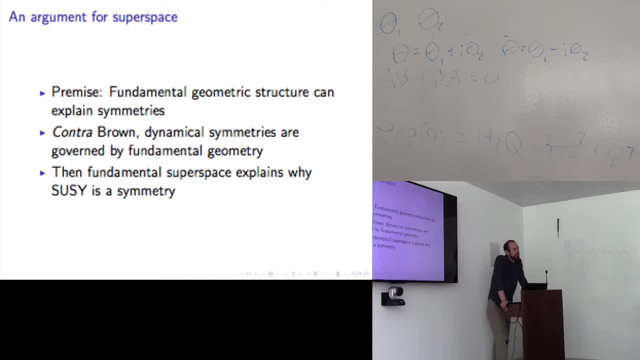 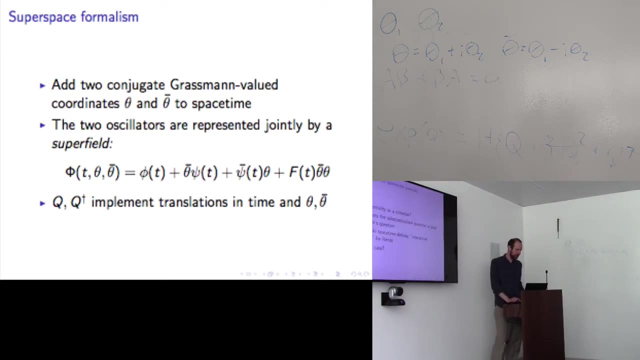 Yeah, and you say, of course you cannot, because if you kind of measure things with rods and plugs, Yeah, You are restricted in some way. But maybe you kind of deal out these kinds of observables in these extra structures. Yeah, I mean, you can absolutely construct operators that are not. 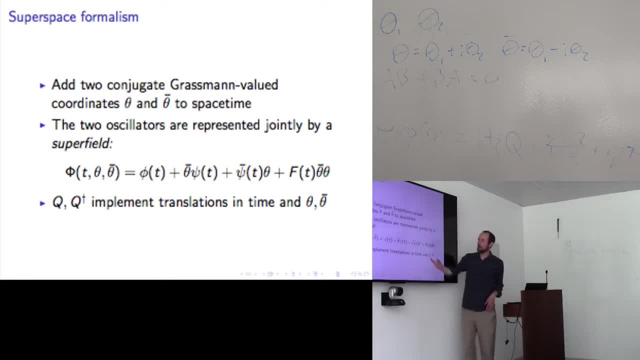 I mean. so, like you know, any combination of these components in the super field, like basically- other than the super field, is going to be definitely an operator right that is not going to be constructible in the Minkowski version, right. 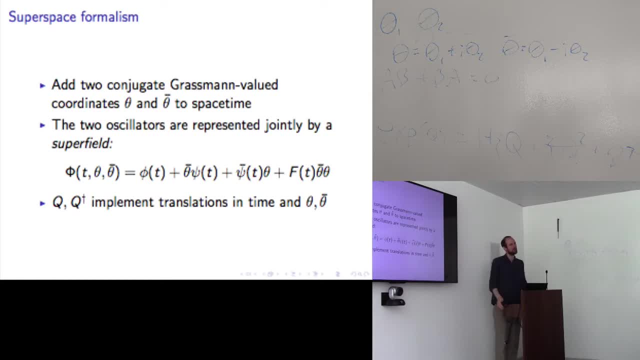 You can construct it in the superspace version, you can't construct it in the Minkowski version. So yeah, there's going to be a bunch of operators like that. Let me make an analogy, right? So take just a regular fermion field: this: I wish I had an analogy that would be more. 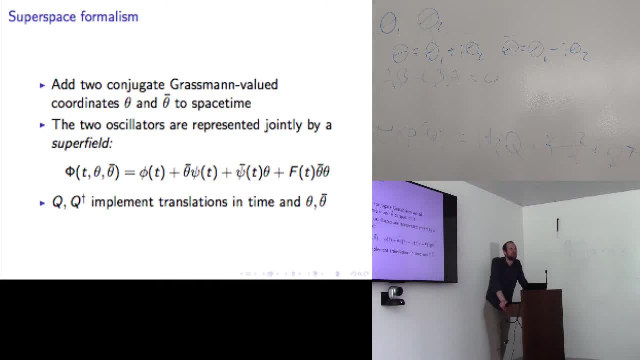 helpful to people who weren't kind of already quantum field theory people, but I'm not sure I do, but maybe this would be helpful. Yeah, so just take a regular Fermi field, right All of the observables. so here's the difference between boson and fermion field theories. 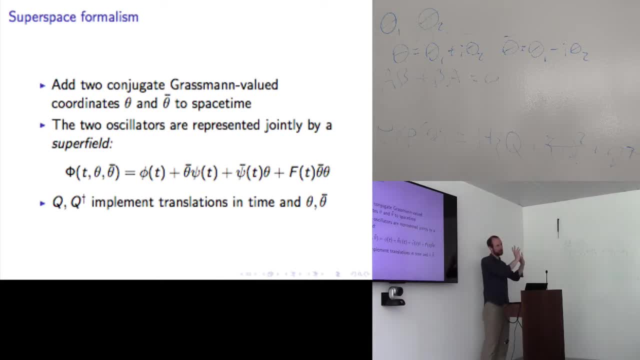 In boson field theories all polynomials in the field operators are observables, right? Which is to say, all of the polynomials in the boson field operators are invariant under the symmetries, and so you're right that the measurability is kind of a weak condition. 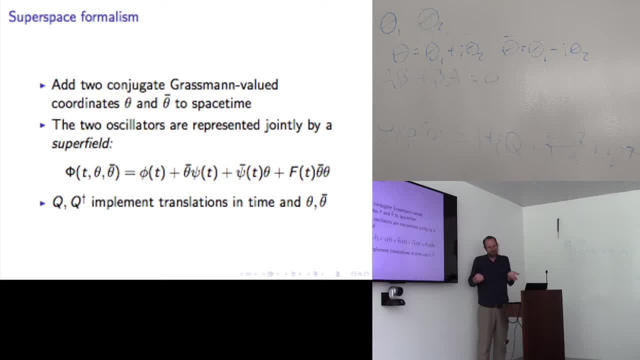 and it's like: yeah, we want to have all kinds of like physical quantities that aren't measurable, but being invariant under the symmetries, I think, is an even more kind of basic requirement. Okay, so sorry to get back to what I was saying, though, in boson field theories, all, 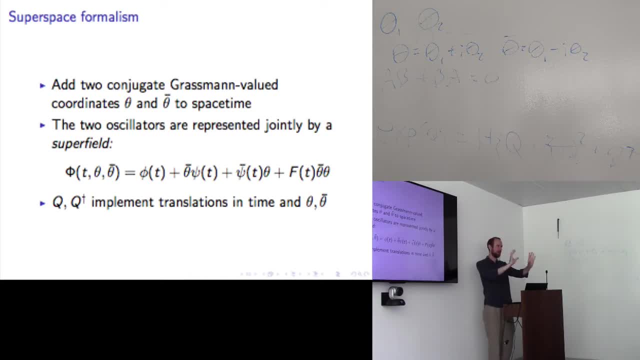 polynomials of the Yeah Of the field operators are invariant under the symmetries and so are observables. In a fermion field theory, only even polynomials of the fermions of the fermion field operators are observables, And there's a kind of deep reason for this, which is that the fermion field operators 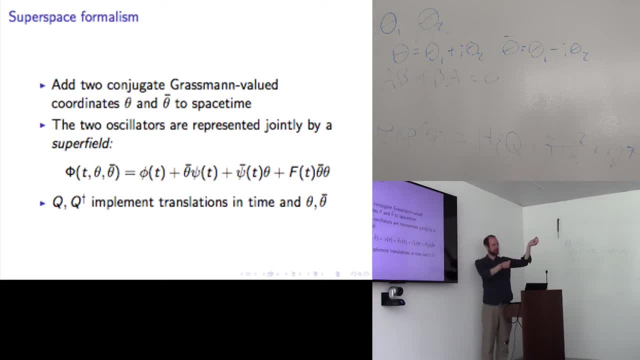 anti-commute- at space-like separated distances rather than commuting. and so if you were to say they could all take on values together, you would get a jumble right because- or another way to put this is, they don't have like. they don't have like real eigenvalues. 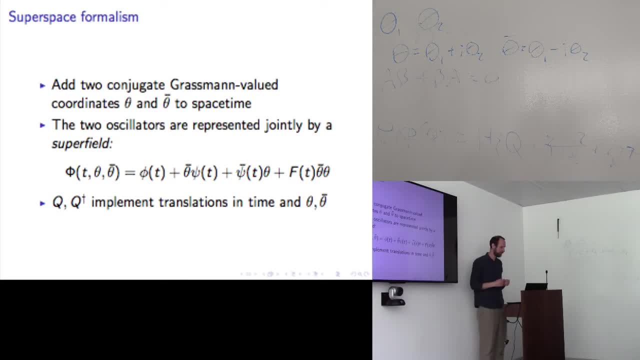 in the way that the boson field operators do. So you have to restrict which combinations of the fermion field operators you're allowed to use to construct observables. And then we tend to- Yeah, Yeah, We tend to say the odd polynomials of the fermion field operators. they're not real. 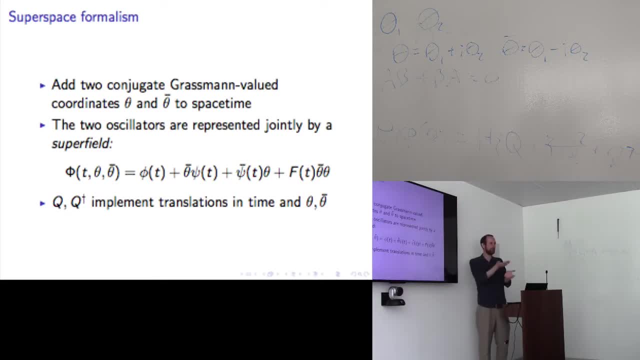 physical quantities. They're kind of calculation tools, right, They're useful in putting the theory together, but they're not part of the real physical content of the theory. That's at least the sort of prejudice that I was bringing to my discussion of the superfield. 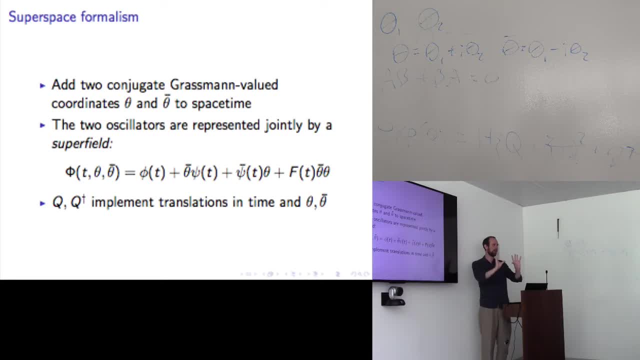 that only the operators you can construct out of the superfield that are going to be invariant and so count as observables in that sense. Only those operators are going to have physical significance. Yeah, That's essentially where that assumption is coming from. But if you were to ditch that assumption, then it's totally true that there'd be a bunch. 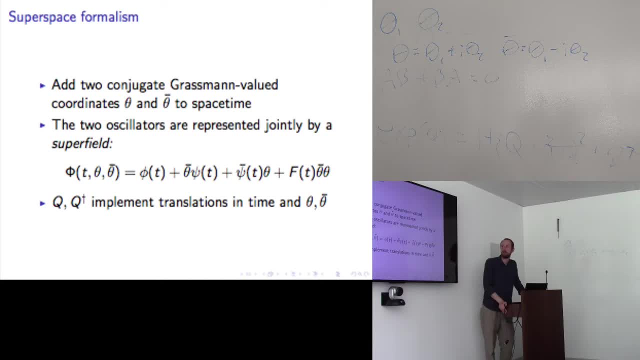 of other functions of you know the different operators that you can put together. that would not be available, So they're not invariant. They're not invariant. Yeah, There's no invariant operators. that only live in the Griezmann. Okay, 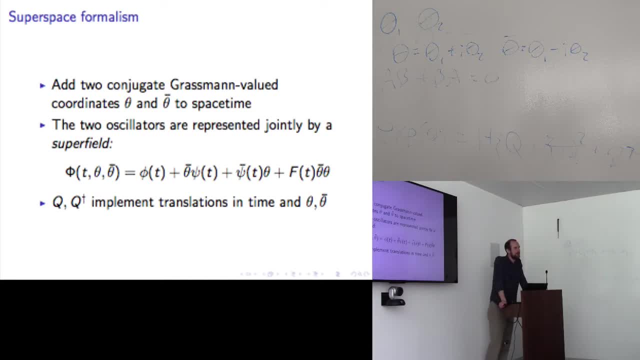 Yeah, that's right. Yeah, There's no invariant operators that are. There's no invariant operators that are going to be non-trivial functions of the Grasmann. I mean Yeah, Yeah, Oh, This is small. There's a very small fault on this. 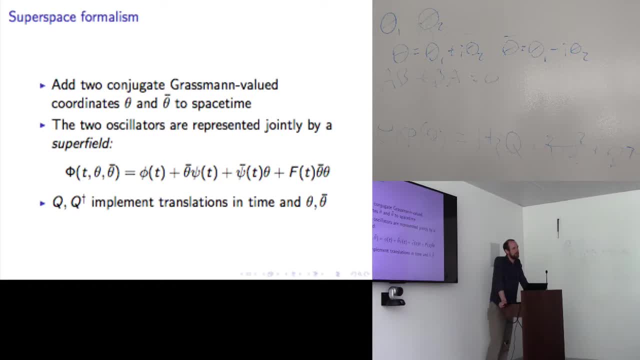 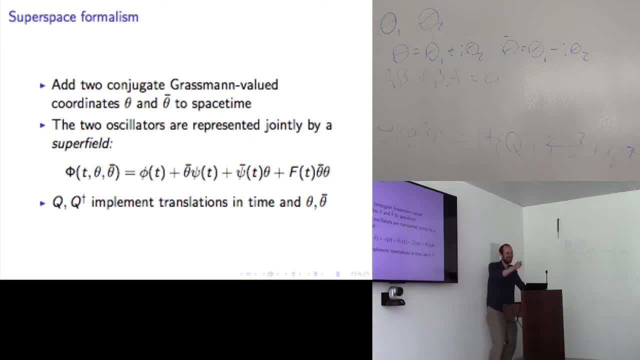 Yeah, Yeah, Yeah. Is the equivalence supposed to be robust up to other things? that you might not. This could be a part of the native theory, but you might want to do with the eligible observables. So, And here's the example, 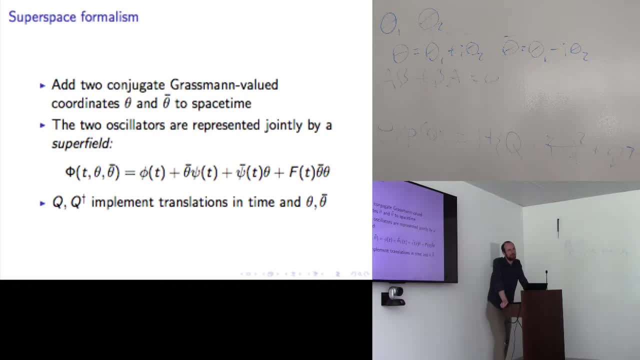 It's a concrete example of New England. We know that we can localize the rigid symmetry and get a gauge right turning interactions. It's also a generally thought that the strategy constructing gra grupos means you localize In this case. so you localize super symmetry and you get super gravity. 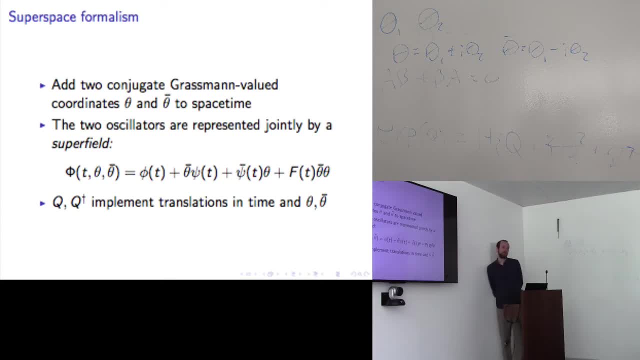 Yeah right, Yeah Right, And generally people do that trick within the superspace formula: Yeah, So is this something that the equivalence is robust up to? I would bet that it was, but I don't know the answer to that. 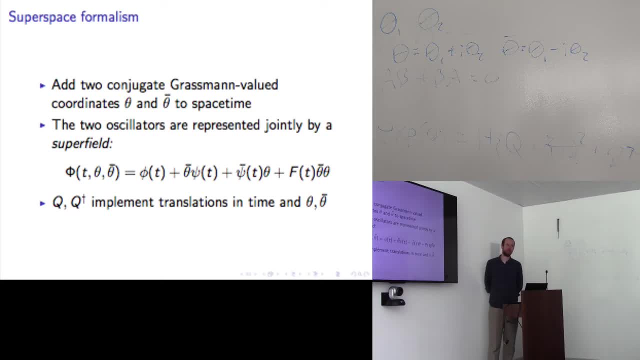 Yeah, I mean it would be really weird if that was not true. So I suspect it has to be true, but I don't really know the answer. Okay, Yeah, It's a question about the general metaphysical picture. So let's take for granted, about superspace and that space-time is not superspace. 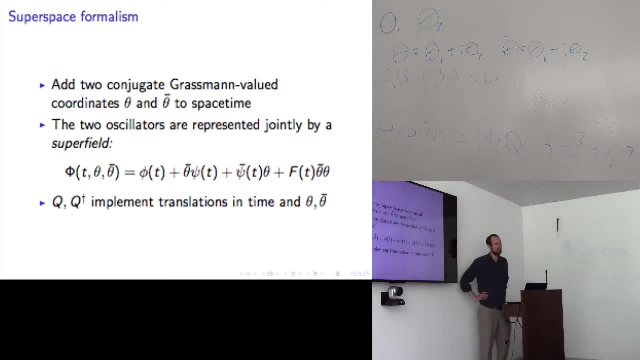 Yeah, Then one question would be: should we be about space-time or not? And it seems that, according to definition, it should be, because it could be as fundamental as matter, And you said at some point that, well, if space-time is fundamental enough, then it. 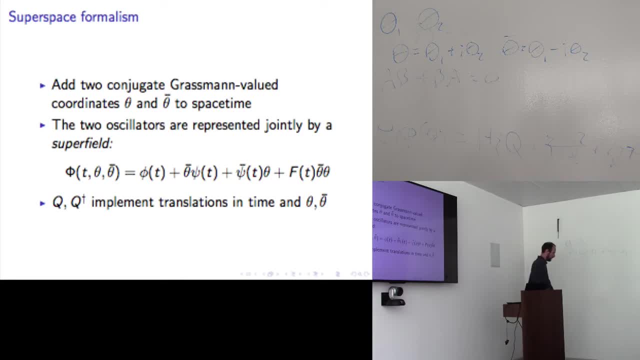 should be in some sense. Ah good, But still, from another point of view it's less fundamental than superspace. And if superspace is absolutely fundamental and space-time is only relatively fundamental, then there is a kind of tension. Maybe it's just a semantic tension. 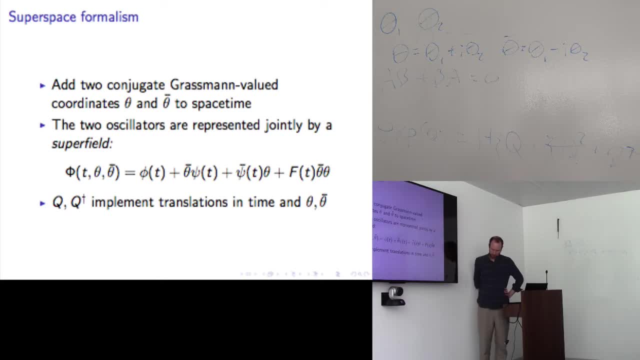 No, No, I think it's not. I guess what I was probably assuming here is that if we take the point of view that superspace is absolutely fundamental, then there is a kind of tension. Maybe it's just a semantic tension, No. 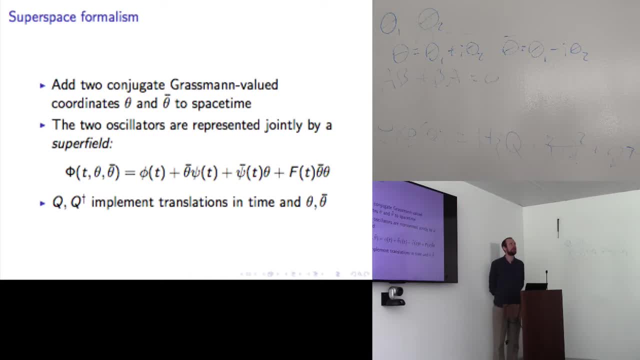 No, I think it's not. I guess what I was probably assuming here is that, if we take the point of view that superspace, well, no, Actually this is. oh, this is good. OK, I was about to say something that was in extreme tension with the answer I just gave. 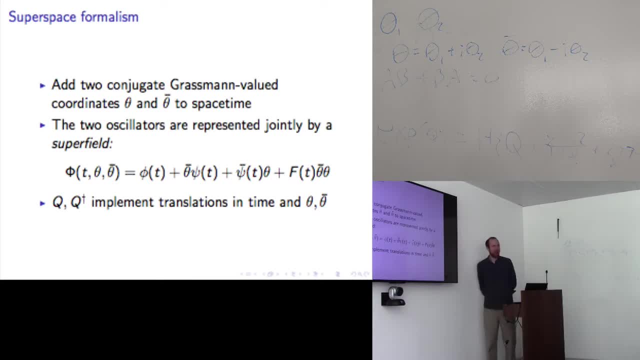 to Sebastian. OK, I was about to say that if we, if we think that superspace is fundamental, then we would. we would want to say that matter is given by the super field. But that's that, doesn't. that doesn't fit with the answer I just gave to Sebastian. 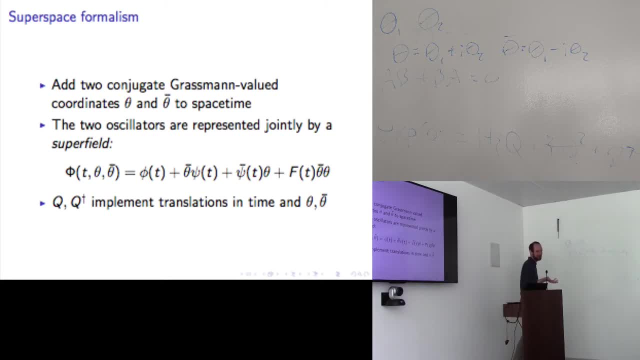 The answer, you know I would. I would want to say: if superspace is fundamental and matter is given by the super field, then it's the answer that matters is given by the algebra observables of the super field, which is the same as the algebra. 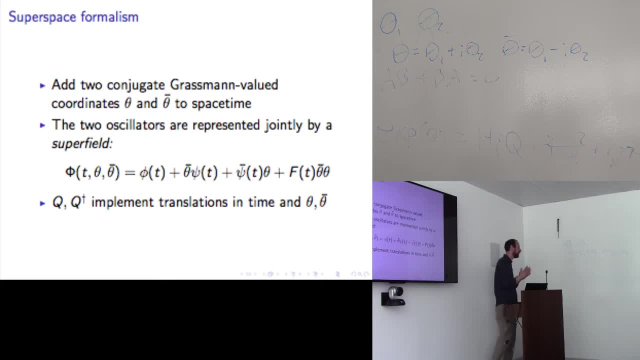 observables of the component fields. So you're right, We have the same algebra observables. This is very rigorous, since which you're right, but the same algebra observables are treating as the matter, And the question is: do we treat the spacetime as the super space that we can? 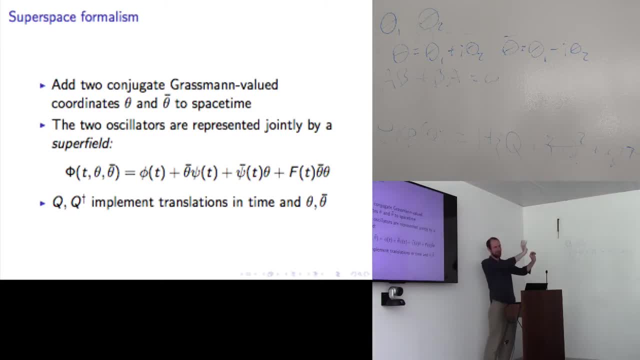 define that on, or do we treat it as the Minkowski space, that we can also define the same algebra observables on? So yeah right, I mean, one point of view you could take is that the fundamental, the most fundamental constituents of a quantum field theory are its spacetime. 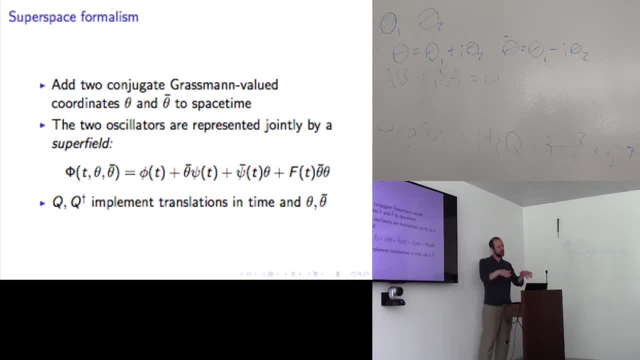 its, you know its geometric setting Right, Right Together with its. you know the observables characterizing the matter of the field Right, And then, from that point of view, you know if those two inputs were super space plus. 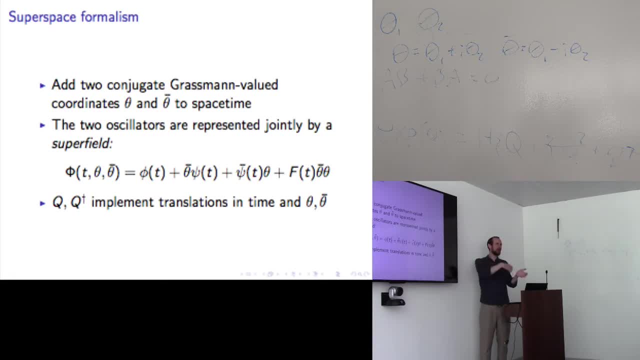 the super field algebra observables, then it would kind of just follow from that that Minkowski space is not part of the fundamental, part of the really fundamental structure, and so it would be less fundamental than the matter, Right? Yeah, I'm not 100% sure that that's the way to look at it, but that's one way to look. 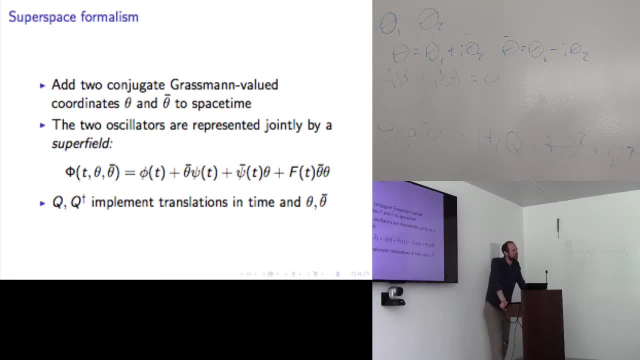 at it. that would address this concern. Yeah, Yeah, But yeah, Yeah, You, I think there. I think there is a really substantive question there. It's delicate work to avoid making this a semantic question, So I may. 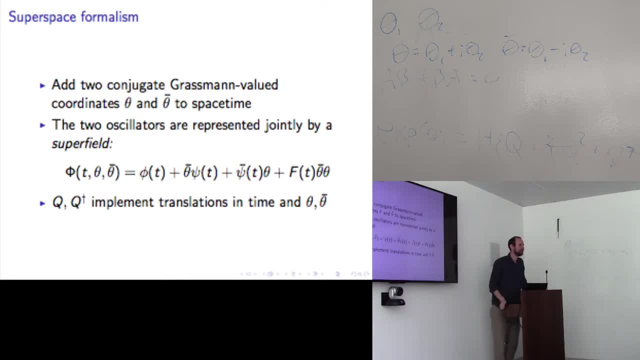 not have succeeded with that, Alex, Oh yeah. So I agree that explaining that you know the, you know the you know the you know, explaining that supersymmetry is a symmetry, is like a pro tanto reason for being. 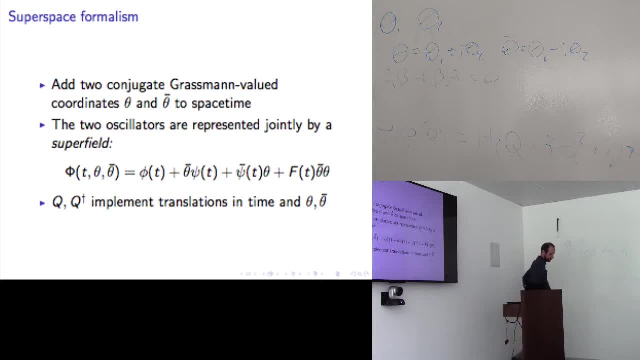 Yeah, a substantivalist about super space And I was thinking there might be like two- you know- possible responses. I don't I wish I had like a more concrete example, But like one would be, maybe that argument would over generalize. Maybe there are other cases where 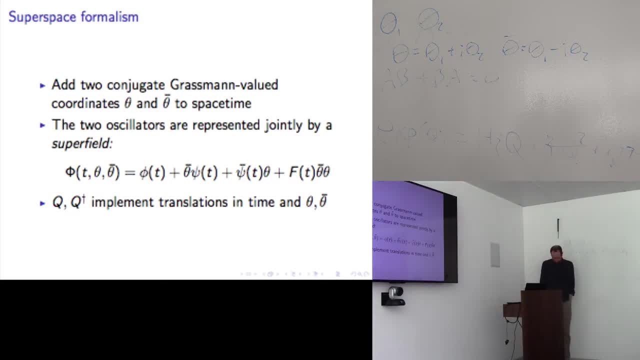 these, these symmetry, like some symmetries, and then you can define some sort of space. and then the argument: you know, this is maybe not super charitable because you're not saying like in every case, Yeah, Like that's a sufficient reason for being substantival. 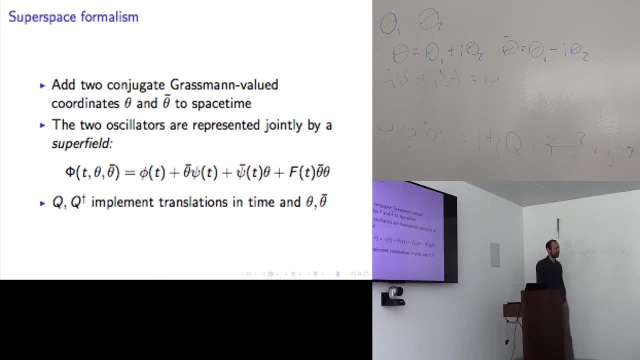 Yeah, My view is: it is just a pro tanto reason for sure, Right, Yeah, But yeah, So I wish I had a better example for that. But then another worry would also be that maybe being a substantivalist about super space would then raise other explanatory. 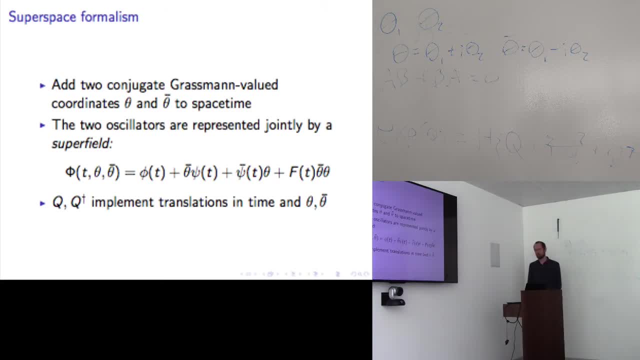 questions that might be then harder to answer, like explaining why you know, why you know ordinary space-time is what singled out in our perception, or something like that, And maybe you could still answer that with the tools of like functionalist approach to the. 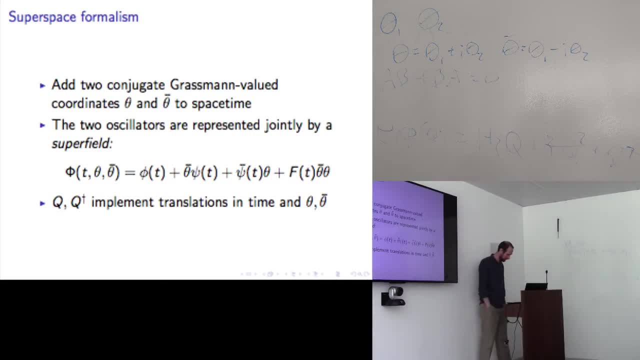 plane of space-time is Yeah, But the more subs space-time like substances there are, I feel like the more those kinds of questions. Yeah, Yeah, I mean. yeah, I think in the second case you would want to give a functionalist. 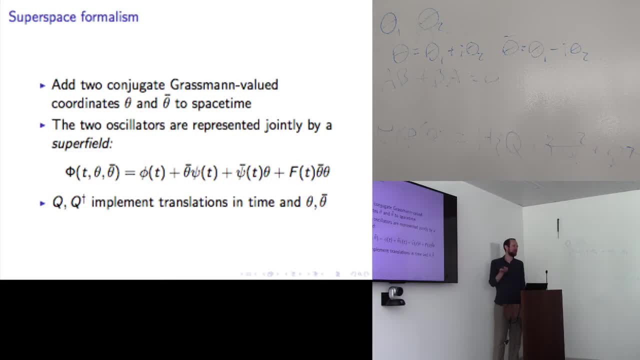 answer to, And you know I mean yeah. So basically one would be in the same place with David Albert in his picture of why regular space shows up out of configuration space, which I think is basically, you know, being a pretty good company. But I mean not that. 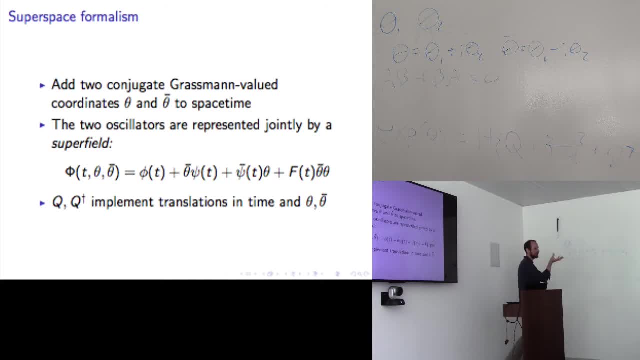 I'm a- not that I'm a configuration space realist, but I think that that aspect of Albert's view works fine. Yeah, And the first part of your question, right? I think a good analogy would be: why aren't we, for example, like, like, let's. like you know, let's say let's. 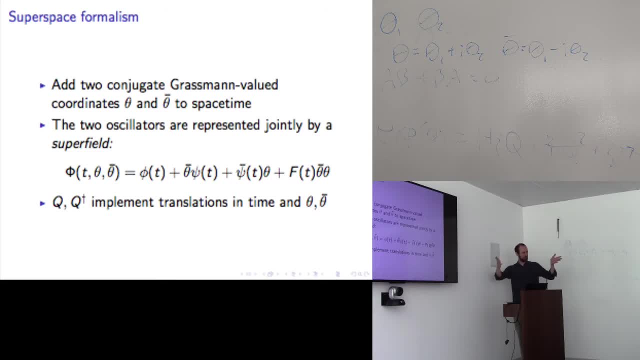 write up a gauge field theory, you know, just electromagnetism or something. Why aren't we substantivalists about the whole fiber bundle, that we could write that theory up on right, as opposed to just space-time, And you know, maybe we should be Some people. 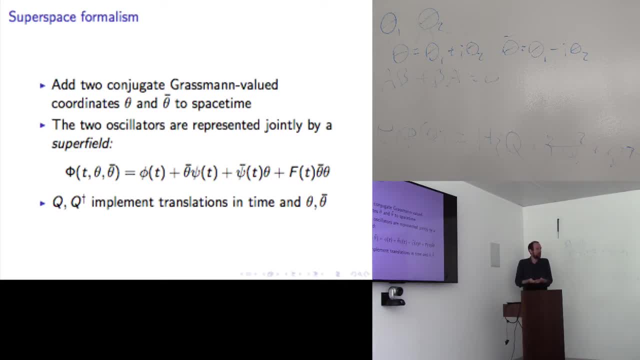 have have said that they were fiber bundle substantivalists. You know, I think there is a particular, there's a particular reason to be a superscriptive of the theory that you're a superspace substantivalist in this case, because I mean like, unless you're- 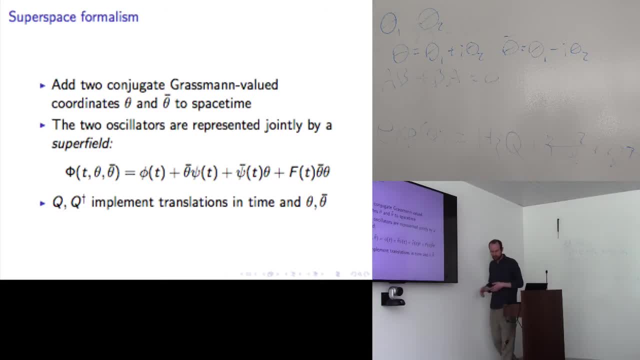 a relationist. which? who wants to be a relationist? That's a joke. I, I, I take relations very seriously, But although I am a substantivalist. But so, unless you want to be a relationist, 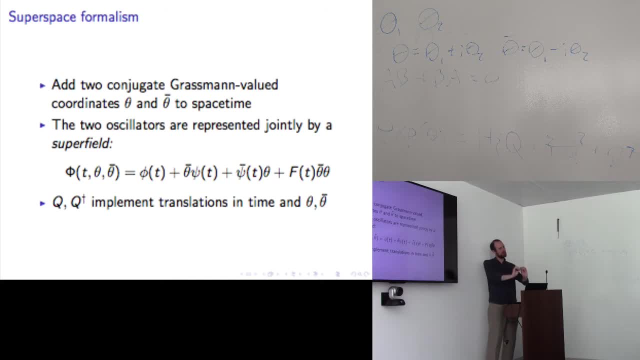 you're either going to be a substantivalist about Minkowski spacetime or a substantivalist about superspace. right, And superspace is not that much different from you know the fact that superspace is not that much of an extra commitment over being a substantivalist. 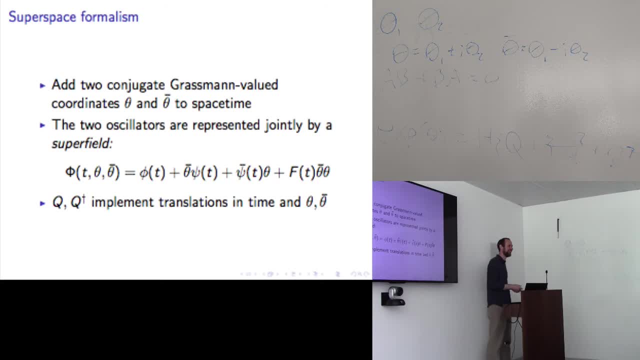 about Minkowski spacetime, And so you know you might think like the extra explanatory gain is worth it for the very small additional logical price, as you know, as compared with like being a realist about like the whole fiber bundle or something which is kind of. 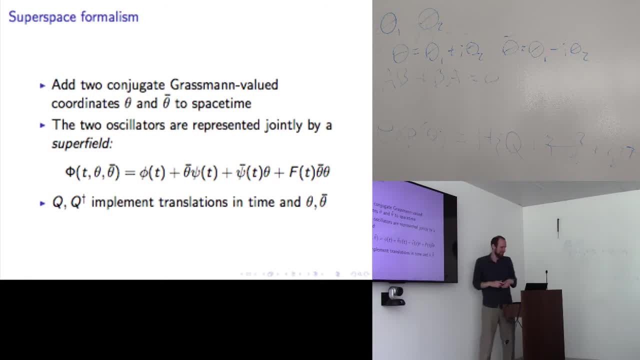 a weirder structure. But superspace is a weird structure. But, yeah, that that's kind of how we're going to do it. Yeah, Yeah, Yeah, Okay. So just asking the, and I'm just asking the: in what sense exactly do you mean that substantivalism from substantivalist? 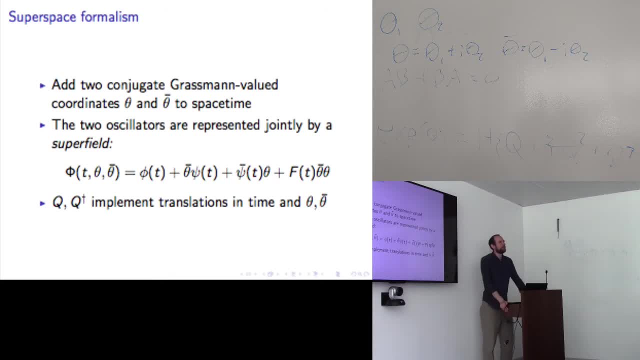 equation is somewhat prior to Reynolds equation. Ah, yeah, So so good. So so that that that's helpful, because I feel like I wasn't very clear about that. So so let's suppose that I say yes to the question about superspace substantivalism, right? Well, if I'm asking? 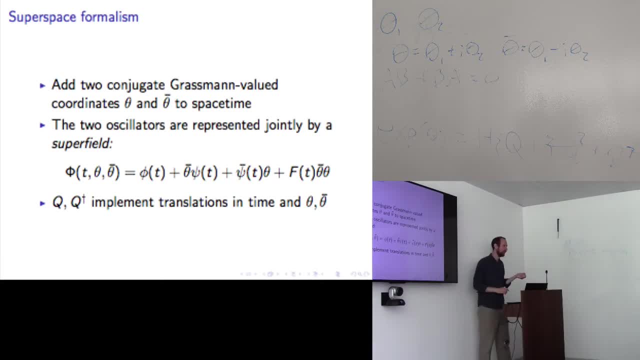 the question about whether superspace is spacetime. Part of that is, you know, like. so I'm. I'm looking at Minkowski phase, I'm looking at superspace. I'm thinking: which of these two things is spacetime right? And and one. 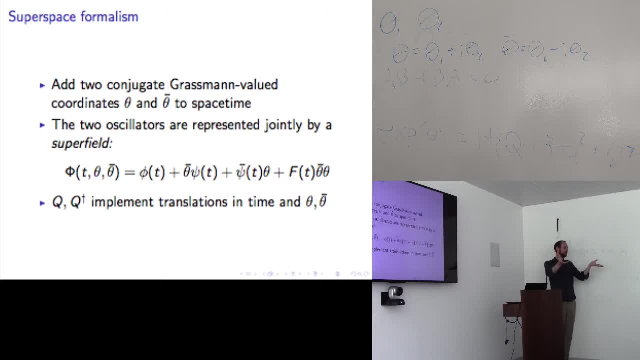 thing you might do. you know there's a version of functionalism where you say it's not exclusive right. You know it's like it's not as if there can be only one. You know, maybe they're both spacetime in a sense right Depends on how exclusive you want to be. But suppose 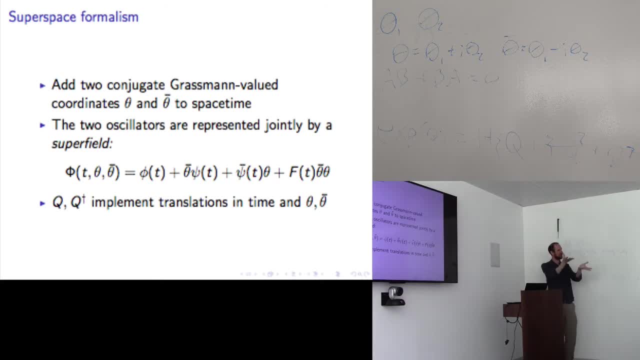 you are an exclusivist and you think there's only one spacetime for a given period. You might say, well, Minkowski, space and superspace, they both look pretty good from the point of view of whether they're spacetime right. It might be that, one of them being more fundamental, 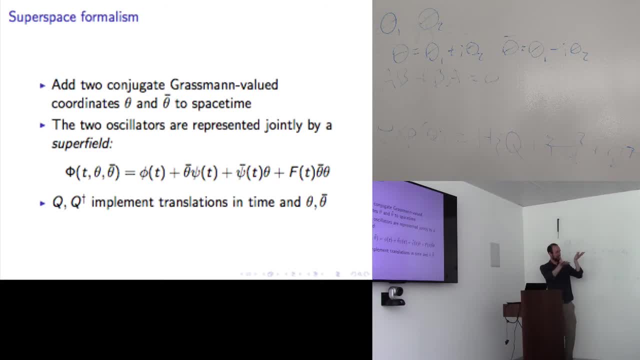 than the other could break the tie here. So if I say, you know, it might be that they're tied on their other virtues and vices with respect to to whether they count as spacetime, so that I think, oh well, if Minkowski space is the more fundamental one, then that's going. 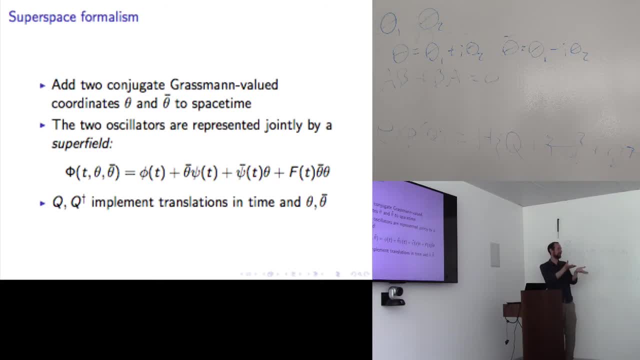 to push it over across the finish line and that'll be good, Yeah, And that would count as spacetime. But if superspace is more fundamental than Minkowski space, that would push superspace across the finish line and that would count as spacetime. 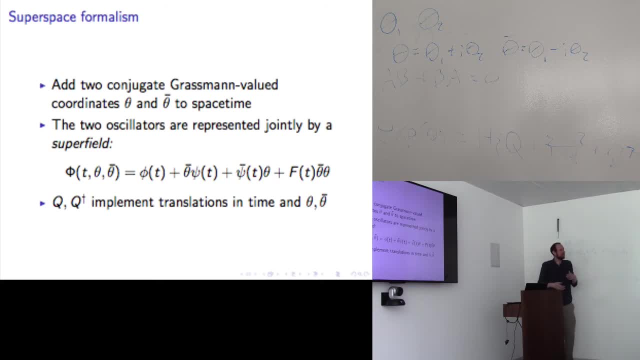 right. So that's. it's not necessarily going to break the tie, because it might be. one highly credible view is: well, look, the operational criteria are going to push Minkowski space to be the winner anyway. right, Because those operational criteria are very central to our 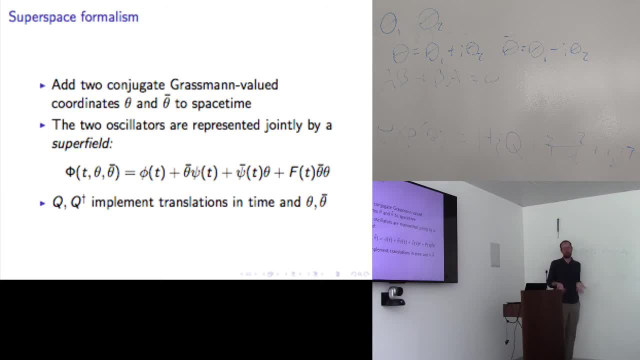 spatiotemporal, our overall spatiotemporal concept, Right. But if you don't think that, if you think that they're tied on the other virtues, then the fundamentality might push one or the other ahead. That's, that's what I was thinking. 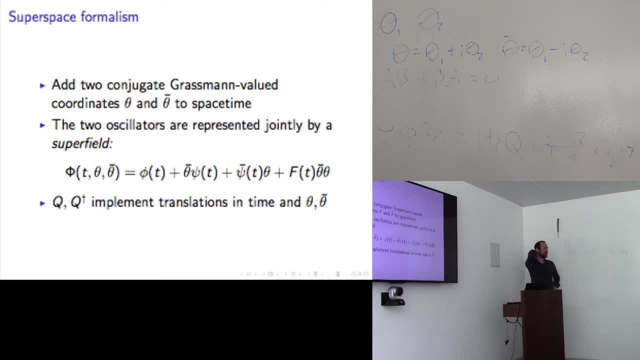 about the. Yeah, just a finger on this. Yeah, yeah, yeah, I have a bunch of questions, but I think I'll save those for the discussion. Yeah, yeah, Just a finger on Neil's question. Why is fundamentality, then, prior to the spatiotemporal? 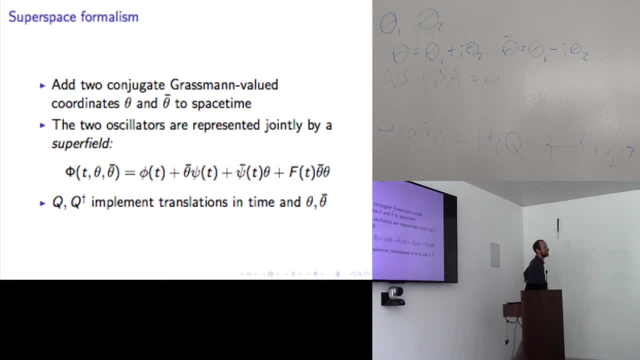 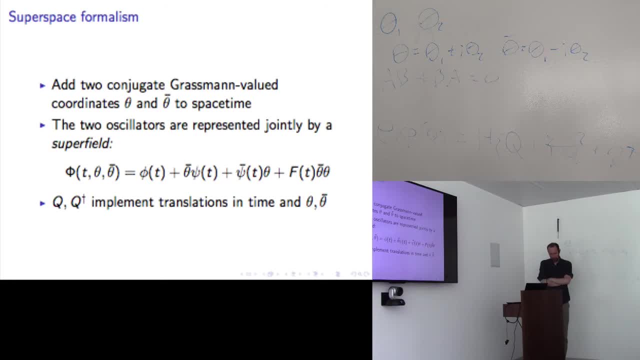 Yeah Well, it's Couldn't, the couldn't, the couldn't. my view on whether or not the spatiotemporal form, my view on whether or not the ah. so this is interesting. I mean so like OK. 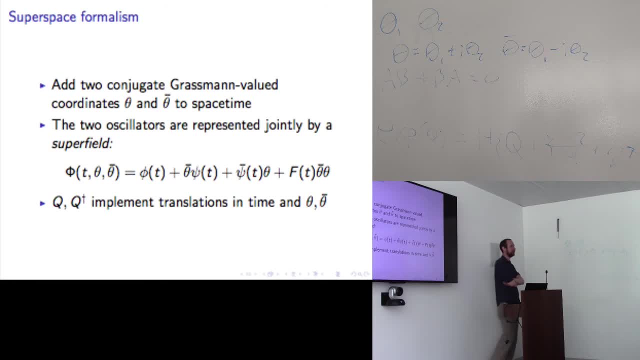 So in the evidential sense, yes, but not in the kind of order explanation sense. So let's think about another. let me make an analogy with another cluster concept, Right? so like I have, you know, I have somebody hands me a box and they're like, hey, you've got to figure out if this contains a game, right? 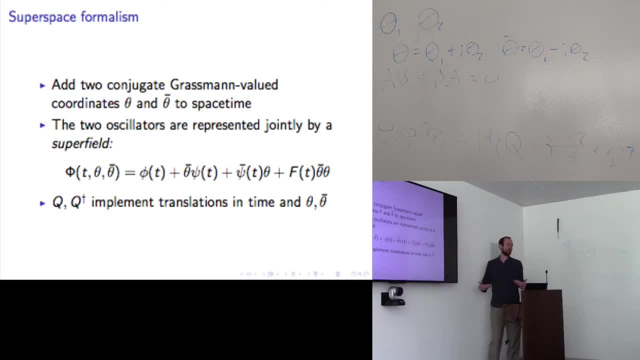 And the box has, like you know, like sorry in it or something, And so I could perceive one of two ways right. But I could look at inside the box and see, oh, you know, it has rules and there are turns in this activity that you know you can use these pieces for. 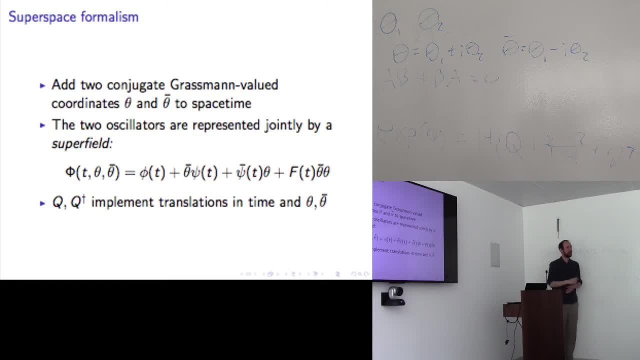 That would be evidence that it was a game right. On the other hand, I might go to a bunch of people I know and trust and say, hey, I haven't looked inside this box that says sorry, but I trust you. Tell me, is this a game? 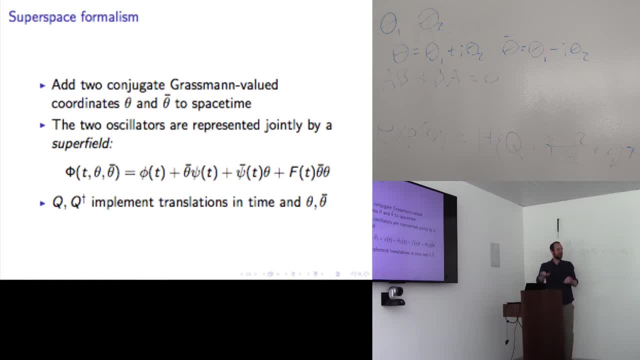 And they, you know, they could say, yeah, it is a game, right? You know, like I played that when I was a kid, it's a game. So now I've gained evidence that it's a game And that gives me a bit of evidence that it has turns okay. 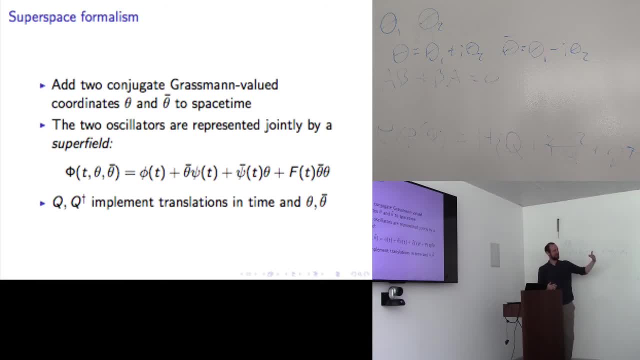 So I can either proceed by trying to find out if it's a game and raise my credence that it has turns, or I can proceed by finding out that it has turns and raise my credence that it's a game. right, But for explanatory purposes, I think. 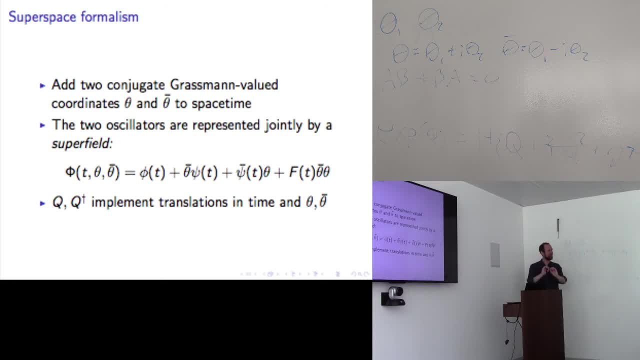 Figuring out that it has turns and discovering thereby that it's a game gets the error of explanation right, Whereas figuring out that it's a game and thereby inferring that it has turns, gets the error of explanation wrong. That's what I would say to that. 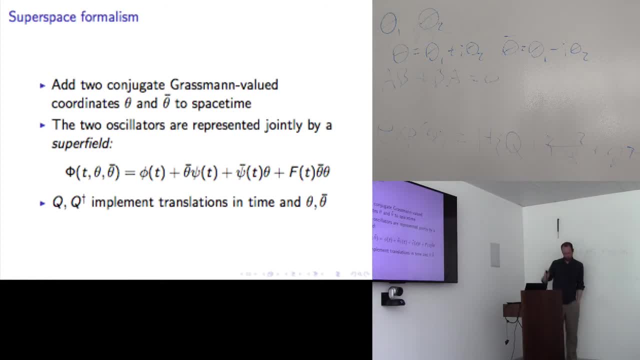 Jamie, Thanks. So when people say that dynamical symmetries are governed by fundamental geometry, I think that there are various things that one could mean. Some of them seem to be binding, Some of them seem to be not, Some of them seem to be less binding. 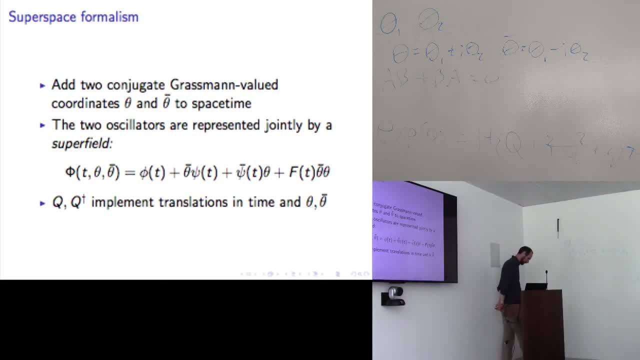 So here's a sense in which I think it's fine: Consider, say, the massless line-bordering equation coupled to a microstimetric field, And then ask, why is that on a gray invariant, Whereas he's given a legit explanation to say, well, it's coupled to a microstimetric field which is almost going to be autonomous. 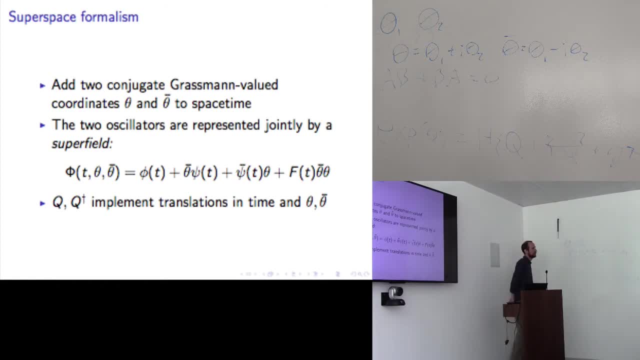 That explains the symmetry of this equation. Here's a sense in which I think it's not fine Write down an isochemical structure like a microstimetric field And then the thought is that, simply and virtually, if I had written down that 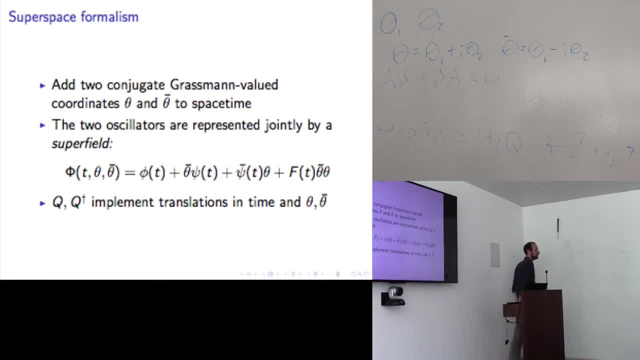 this is a geometrical structure, I can only have dynamical equations which manifest as symmetries for that piece of structure. And it seems to me that principally, it's the second which is criticized by, say, Brown and Cooley. 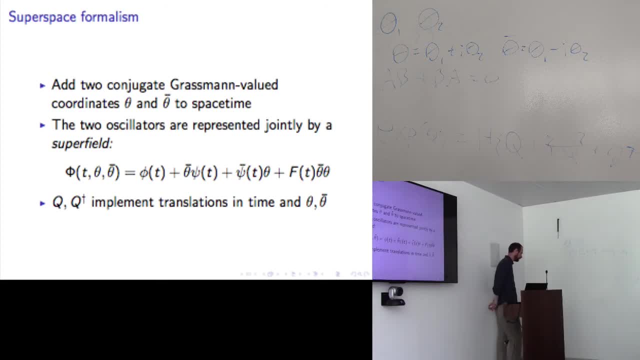 So they say something like as a matter of logic alone. it doesn't follow that like write it down as a geometrical structure, We have to have dynamical equations for certain symmetries. The thought is that we could have other pieces of geometrical structures which the mass fields couple. 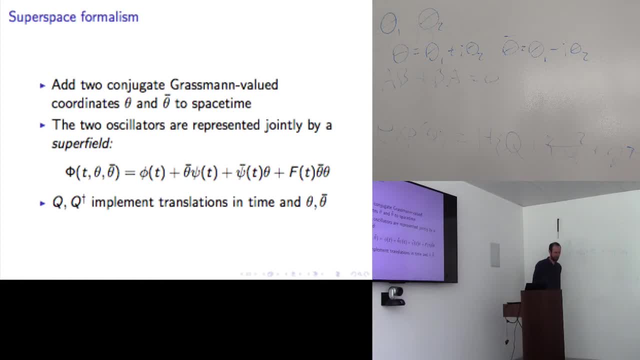 such that they're dynamical equations but they don't manifest as symmetries. Yeah, Symmetries. So that initial privilege is a geometrical structure. So I was wondering which of these two views, the former or the latter- you are more or less aligned with. 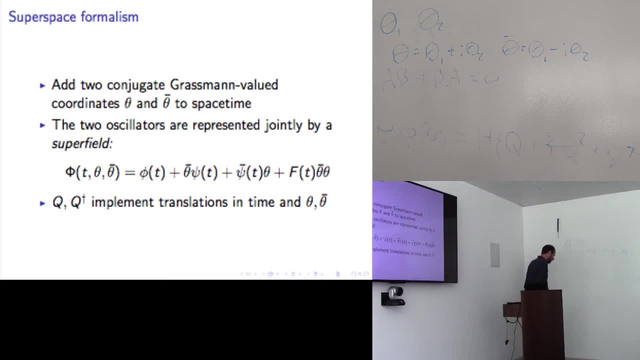 when you made this claim that dynamical symmetries become like dynamical symmetries. Well, I think it's something that was a little bit between, Because, so you know, I absolutely agree with Brown that, like there's no mathematical or logical or metaphysical necessity, 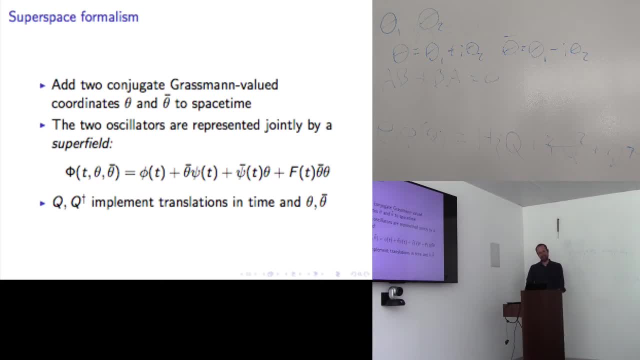 that says that any you know, A to I, J, needs to, needs to always like govern the symmetries of matter fields in the world that it's defined on. What I would say is that it is. I'll put it this way: 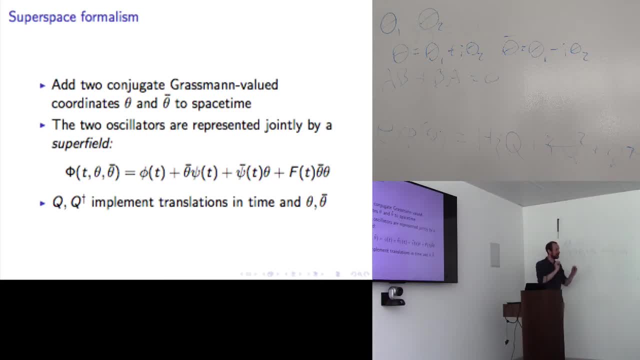 The following hypothesis makes sense to me: I can take an A to I, J- you know the substance represented by it, the geometric substance represented by a metric, and declare that it is a fundamental background, which to me amounts to saying it's a law in the world where that metric exists. 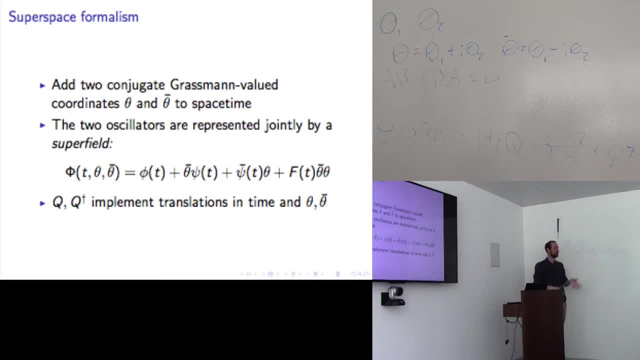 that all of the fields in that world have to obey the symmetries of that metric Right. I can say that that's a law And that's not the same as taking it and coupling it to a particular other field and saying they share the same symmetries. 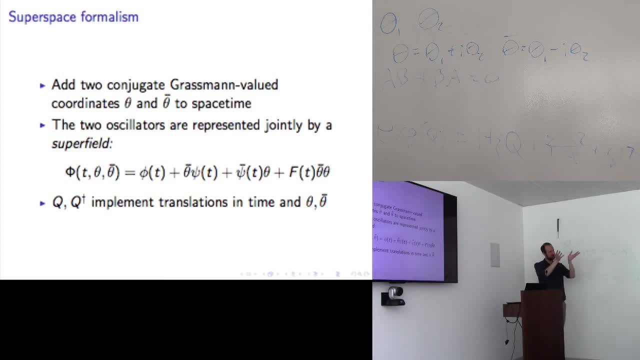 Instead I'm saying, like this is a this, this, this metric is a substance, and it's the sort of substance that governs the other matter, substances that might show up in the same world. Yes, I think I actually agree with you that if you, if you make the stipulation that this is the only piece of geometrical structure, 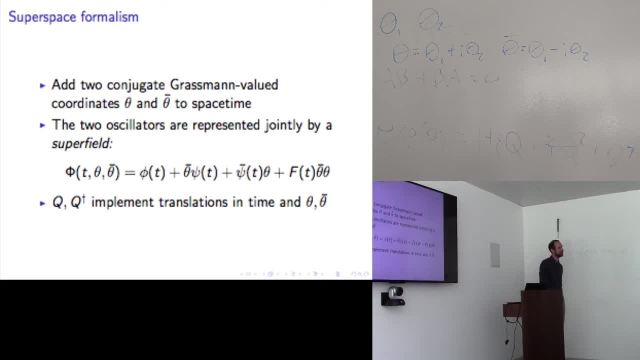 which you can work your math with. then this can explain all of the symmetries of all of the matter fields. Yeah, I think. I think Brown might also say there's a sense in which you can make that stipulation, but it doesn't make sense to say that that's. 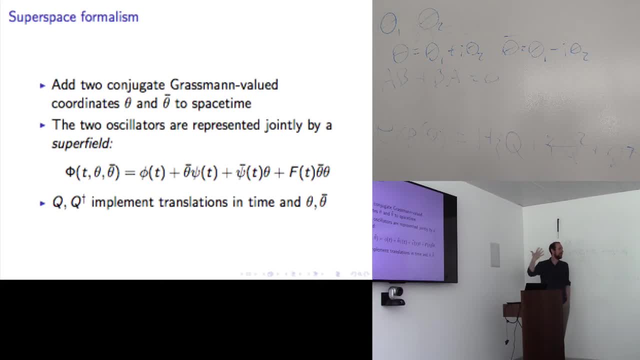 that that stipulation is a law of nature. Yeah, I think I think Brown would say it doesn't make sense to say that stipulation is a law of nature, Whereas I think it does make sense to say that that stipulation is a law of nature. 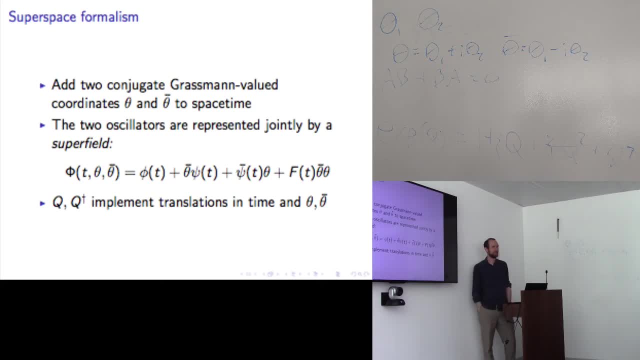 We've got a couple minutes left. Is there any questions? I have just a question which might be a bit provocative, but you mentioned this idea of your friend or colleague in Michigan who claims that super space is more fundamental. Yeah, I guess I would like your comment on how you judge the ontological weight of accepting this super space as a greater space over just positing that the mass scales are similar. 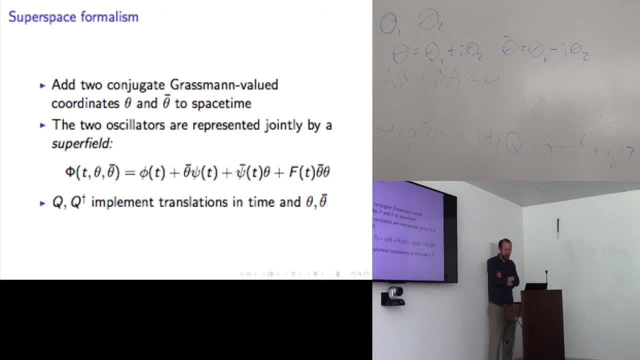 Yeah, Oh, you mean, you mean. so there's two ways to read that question. One of them is: which is a more reasonable posit, and the other one is: is there anything to the one posit over and above the other? 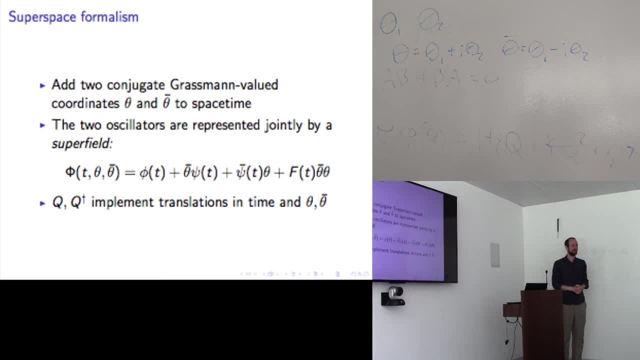 So which of those two, Which of the two questions do you ask? I don't want answers to both, but the latter would be would be the primary answer. Yeah, I mean, right. So so I think one way, one way to to answer the latter question would be to say: you know, it's a little bit related, actually, to what I was just saying to James, right? 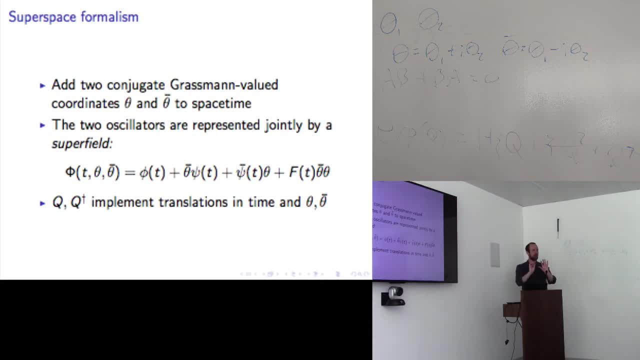 Because there's a difference between saying X is a law of nature versus saying that a law of nature this particular type governs this particular structure, right? So like, for example, I might say: it's just a law of nature. So so like: here's a, here's a weird, implausible system of laws, right? 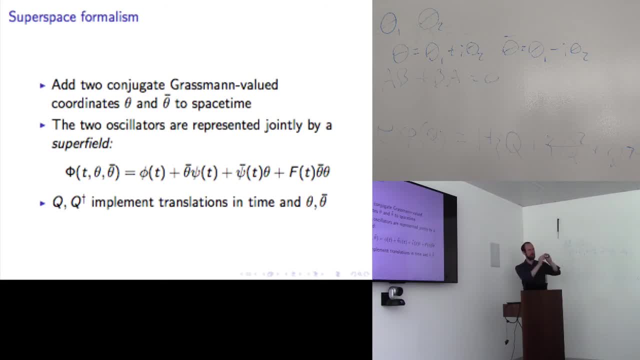 Like I, I chuck this pen and we look at the exact trajectory it takes and I say it's a law of nature that this pen would take this exact trajectory, right, Like this exact pen. This exact object would take the exact trajectory, this one right. 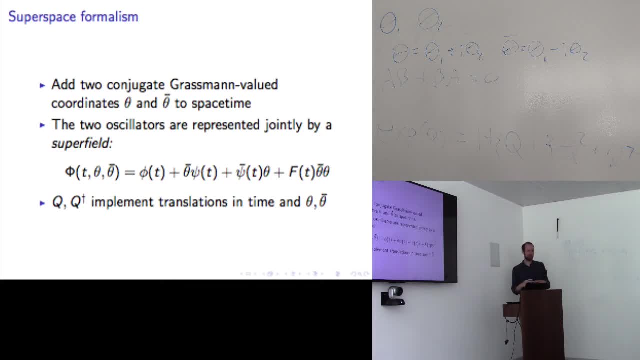 Or I could say it's a law of nature that the trajectory of the pen would follow a geodesic in you know the space-time that it exists in, right? I guess that wouldn't really happen if I chucked it, but whatever. 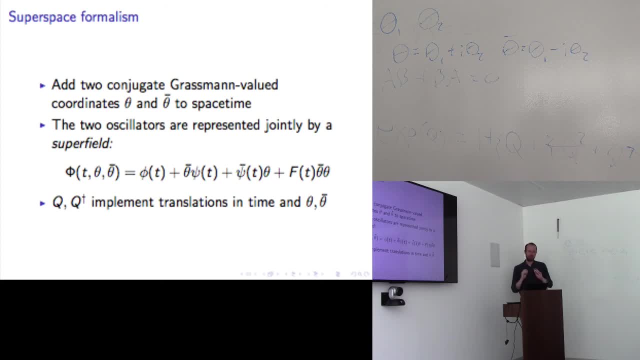 You know I'll let it go So to me positing that it's a law that the masses are the same. I mean you could say it's just a coincidence that the masses are the same. That would be, that would be weird. 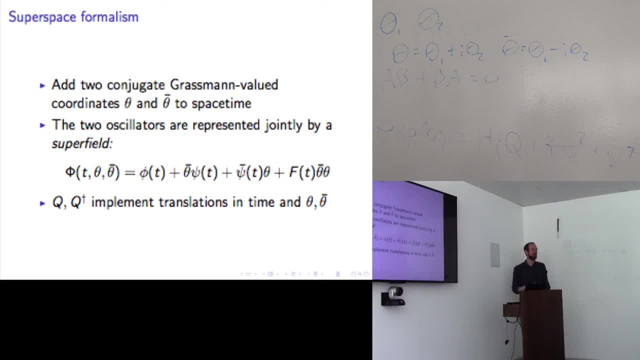 But like positing it's a law that the masses are the same is. you know, it's a law that's kind of like, that's kind of dictating particular facts in a more direct way, as opposed to saying: you know, there's super space and it's a law that the symmetries of matter have to mirror the symmetries of super space. 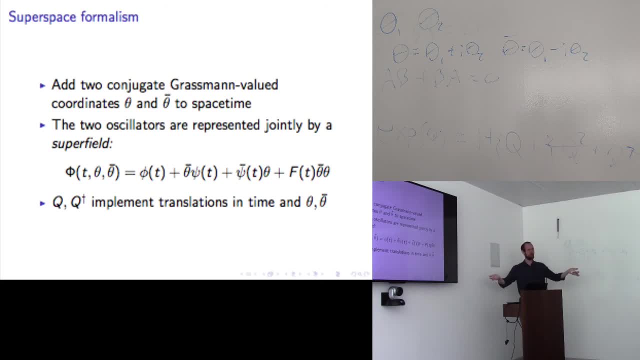 That's kind of a law that dictates circumstances in a more general way. And you know it's a bit fuzzy. The theoretical virtues are really hard to pin down, but it seems to me that we like laws that dictate the circumstances in a more general way. 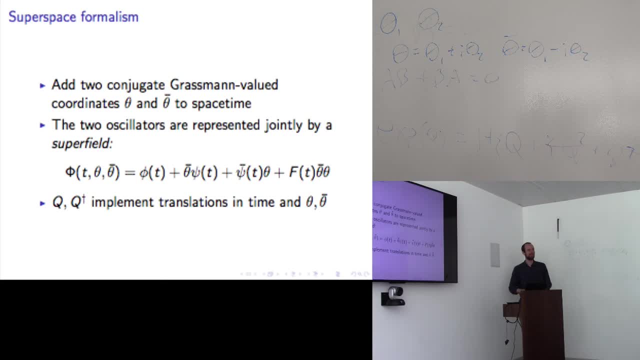 Oh, certainly, Yeah, yeah, I understand that. Like. my question is: you know we can, Oh, oh, This sort of goes back to Go ahead. Yeah, yeah, Okay, good, Good. So now the difference. 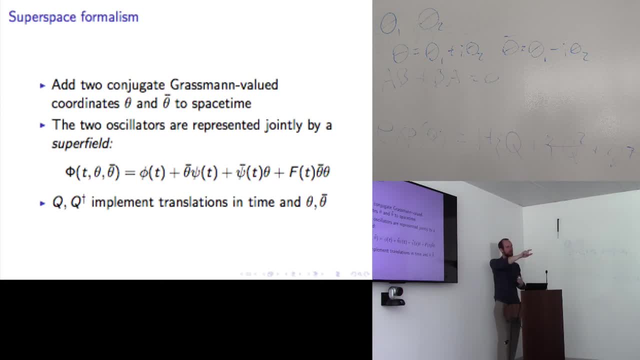 Sorry, Am I wrong? or were you about to say you were asking a question about what's the substantive difference between Between those two hypotheses? Is that right? Yeah, yeah, yeah, Because you're right, I like turned your question into something different. 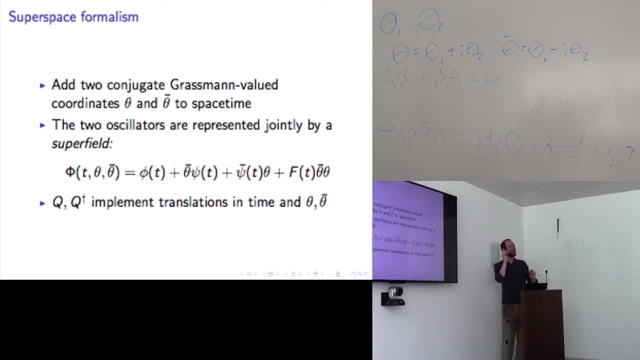 Okay, So I understand. Yeah, yeah, sorry, So okay. so here's a question like: what's the difference between a law that says every object that actually exists follows every exact trajectory that it follows, versus a law that says like, as a general matter of fact, objects will follow these duties? 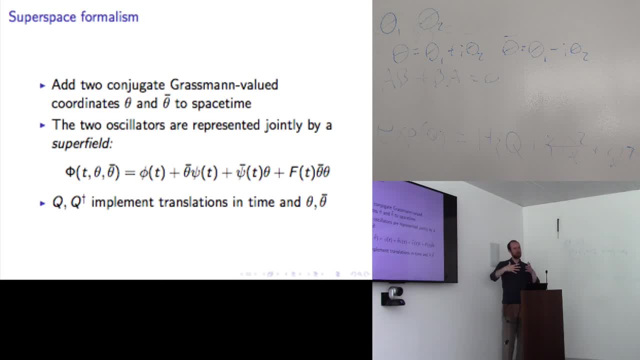 In other words, one of them has a kind of like A more unifying structure, one of them has a kind of like more particular structure. okay, But the specific answer is: you know, I like the idea that's coming out of contemporary metaphysics.